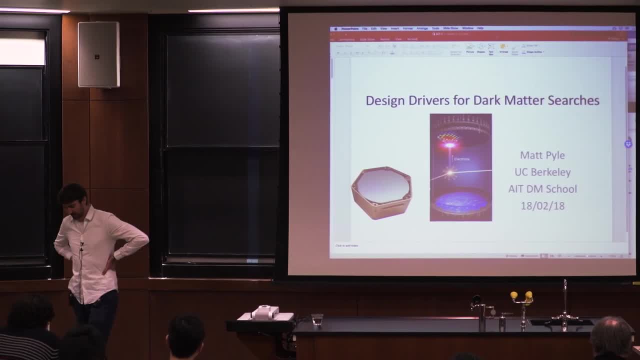 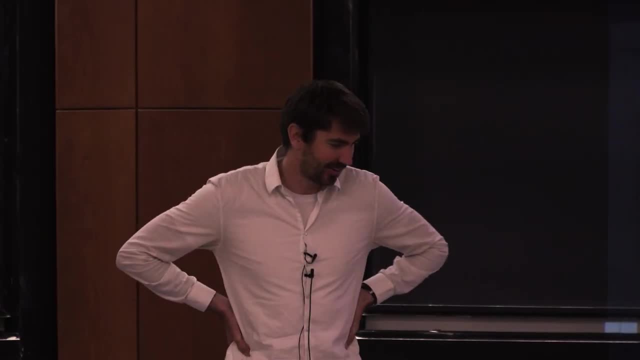 up with a new experiment. of course, like you know, when you go to grad school and you're, and you have- like I'm gonna go work in the LHC- the experiments already there, and then you're just trying to figure out what your analysis is. But every once in a while you get into this world where it's an 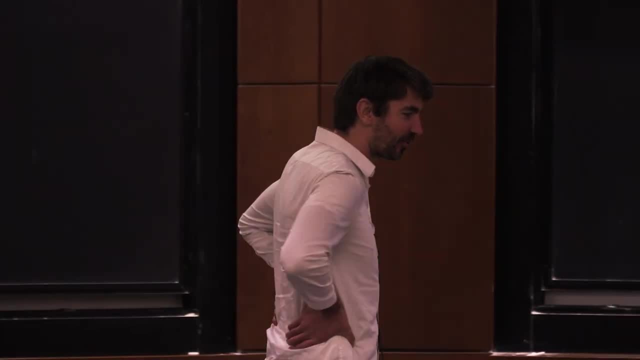 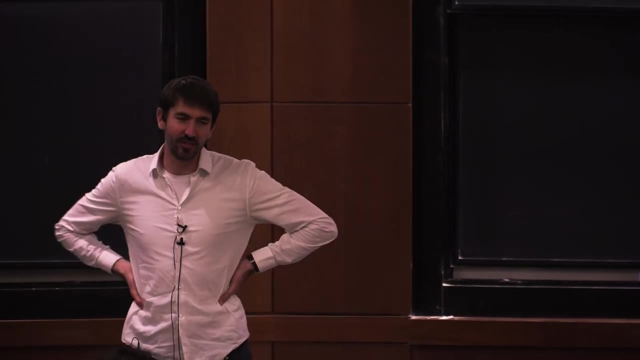 exciting new world right, and there's a new theory out there, and in this case, light mass. dark matter is this area that's exploding right now, and so you really want to ask: if I could just start with a white blank sheet of paper, what would my detector look like? 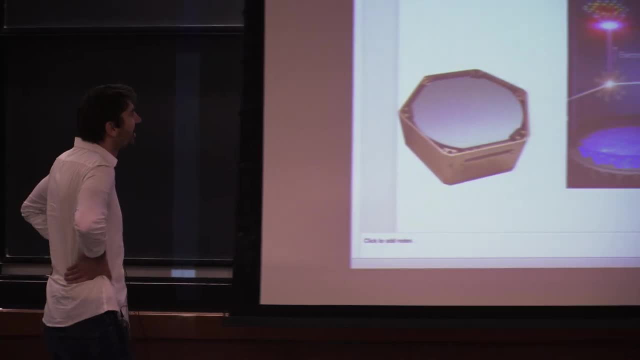 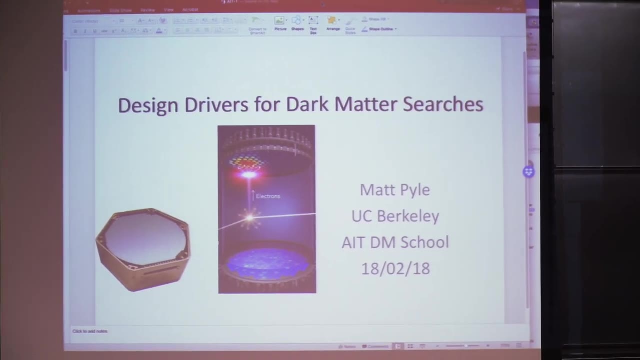 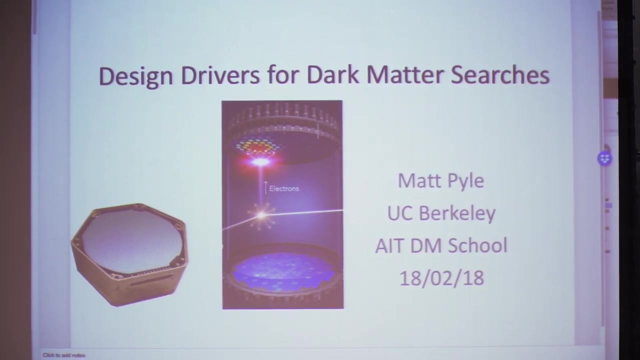 What is the best detector to search for this stuff? And so I think we're gonna start with that idea of a blank sheet of paper and we're going to go through and say what would be the best detector to search for dark matter in all these different mass ranges. 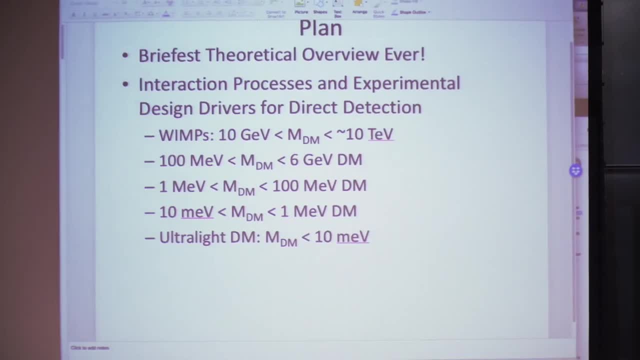 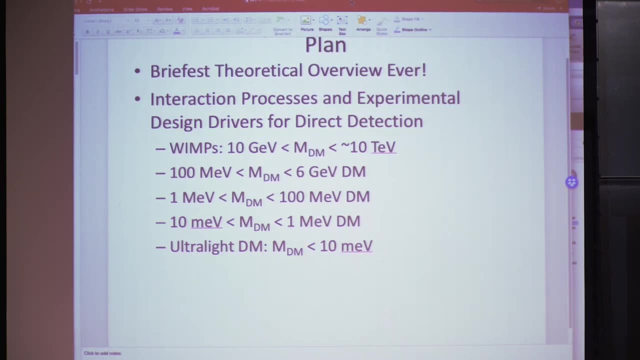 So that's basically the plan here. the theoretical overview is going to be crazy brief. it'll be one slide, because you've already had two talks on theoretical overview, and then we're just gonna go through all of these different mass ranges and try to come up with theories of. 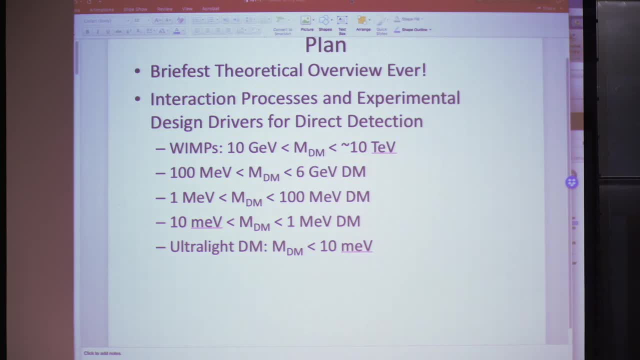 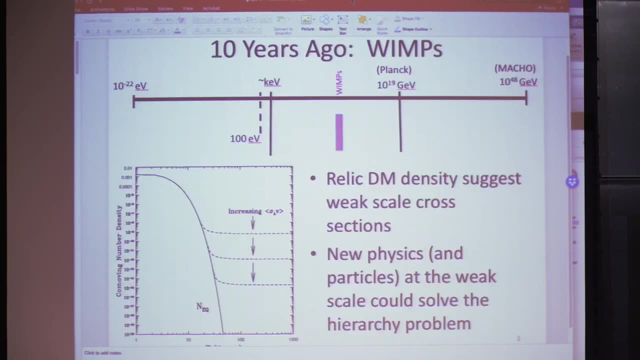 how to build a detector. I actually have plenty of time, so feel free to converse. We even have chalk on some chalkboards, so you know we can swap to a chalkboard whenever we want. So This is roughly the experimental world 10 years ago. 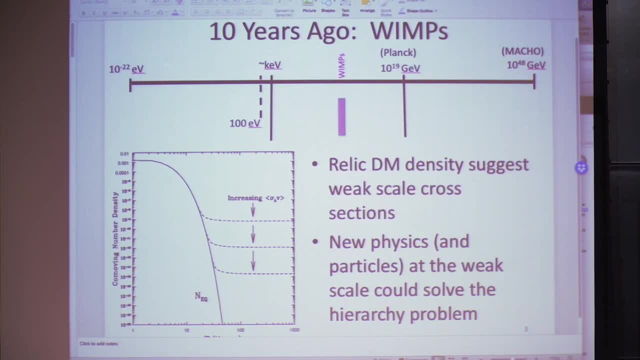 All of us were searching for WIMPs, so things above 10 GV and below a few TeV, And there was a few exceptions to this. A very tiny amount of money was going to ADMX for axions, but the vast majority of experimental physicists 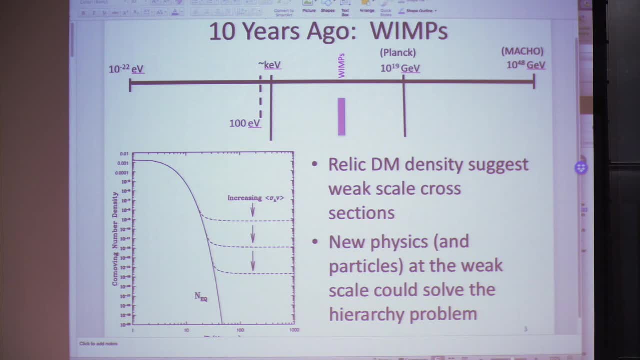 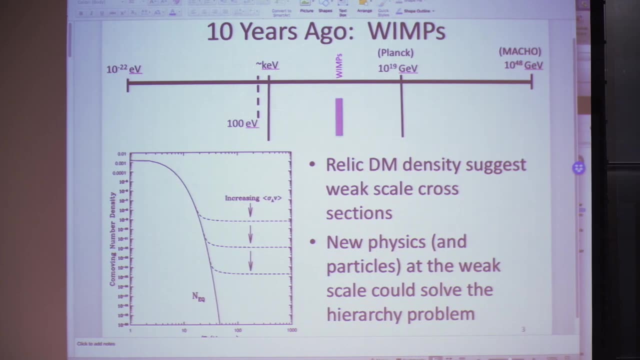 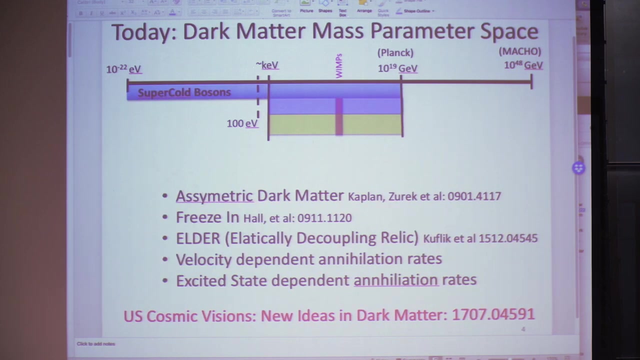 working in direct detection were searching for WIMPs, And it's a beautiful theory. We have this idea of the WIMP miracle, where there's new physics of the standard model which would exactly explain this relic density, And the problem is, unfortunately, 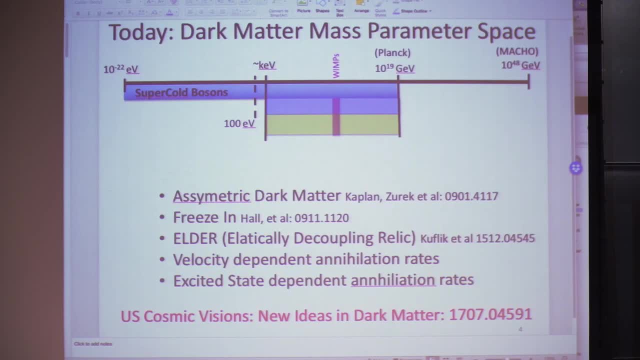 we've been searching for this both at the LHC and we've been searching for this with these amazing detectors that we're gonna talk about, actually, in the next 10 slides, which are xenon and noble gas, TPCs, and we haven't yet seen anything. 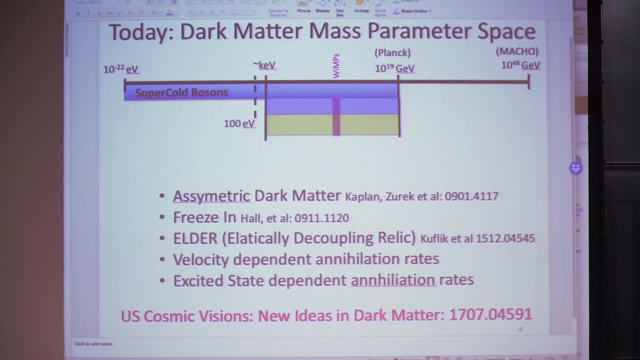 So because of those two issues we really now started to push and say this was a mistake to limit ourselves solely to this little region. here There's this vast region all the way down to 10, to the minus 22 EV in mass. 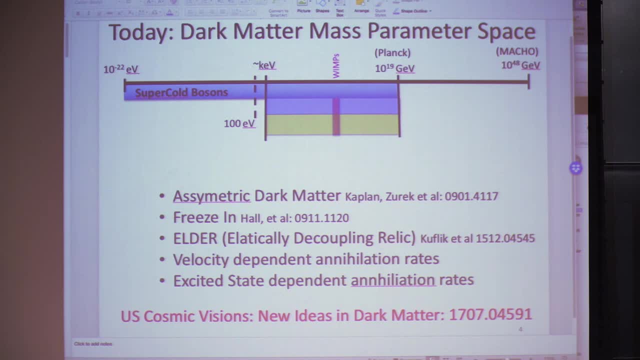 where we could have ultra-cold bosons, and then all the way up to 10, to the 48 GV, And we really wanna design experiments to search this entire range And, in particular, I actually tried to think about how to build experiments. 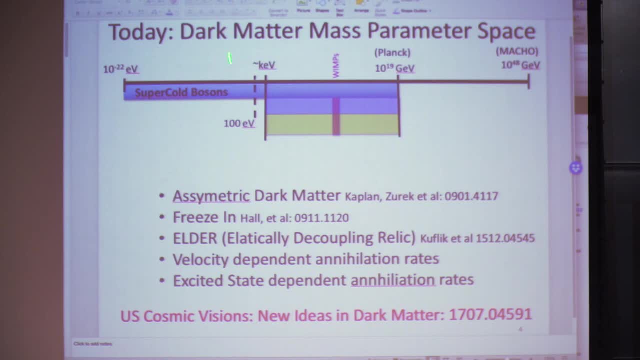 from one GV down to something like 10 mil EV. That's the range where I try to play, And you've actually already heard about a lot of these ideas. Asymmetric dark matter was just this last talk. Friesen was this last talk. 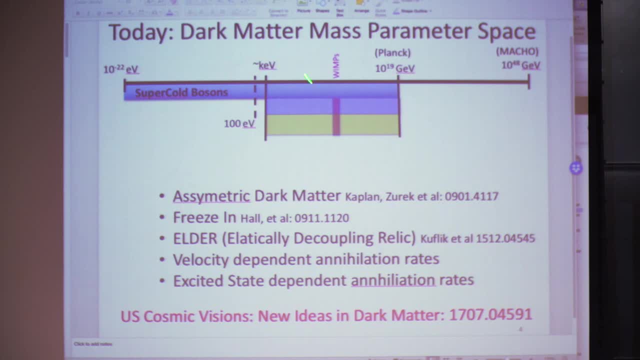 And you can actually see all of these new ranges below the WIMP. so all of these areas here, as well as axion searches, in this new community white paper that we wrote, which was US Comic Visions, which is- there's the archive number. 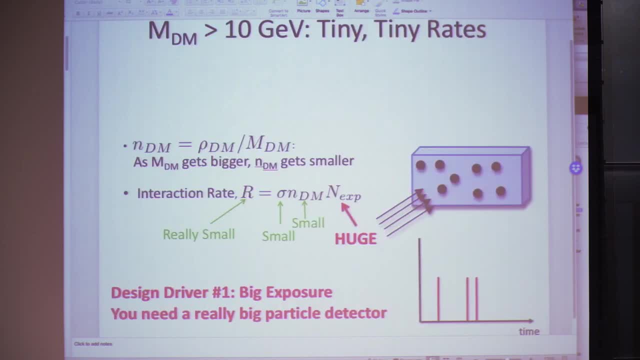 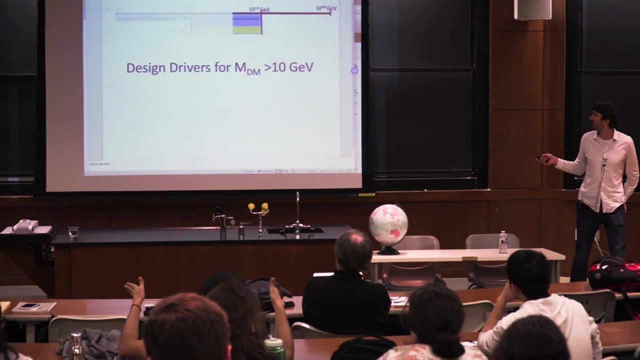 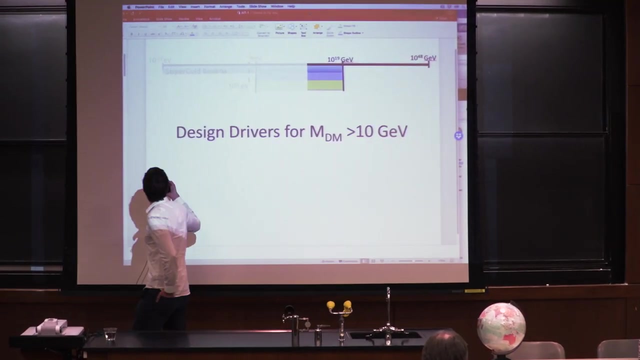 So let's now go and first talk about design drivers for Yes, Where you choose the minus 22 and the 48,. why not higher or lower? Oh okay, so No, so minus 22 is basically the scale. I have these slides. it's a shame. Minus 22 is basically the value that we get you guys there, My face is up. This doesn't have. it's okay, sorry, we didn't want to do this. I wasn't working today on this. Okay, the parallel close and we just been on it for half an hour. 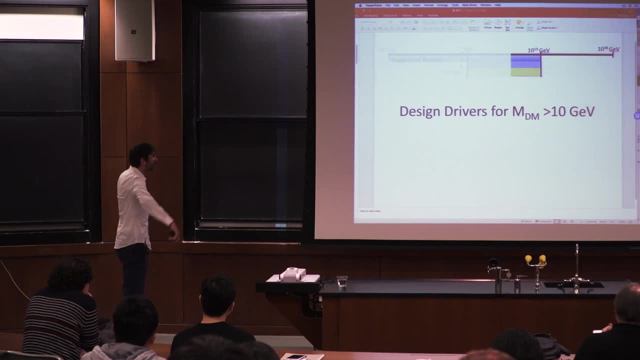 it's good to be very cold over the last 24 hours. It's not cold here, but the world is warm in here. The roller over the next year, holly mollin' hot, is basically the scale of galaxies, So we know mass has to be there. 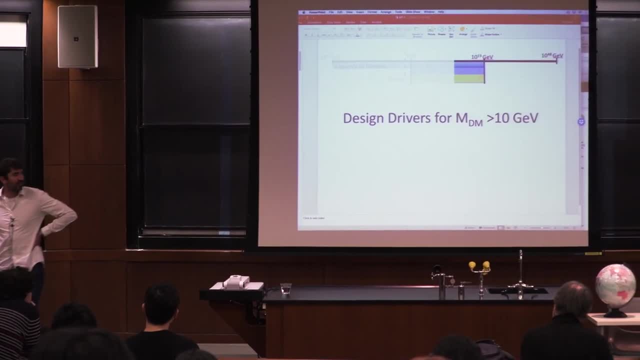 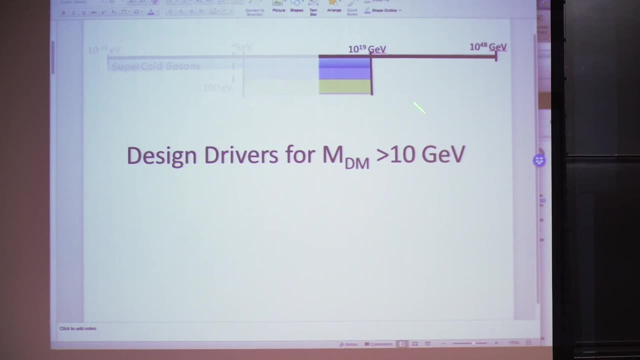 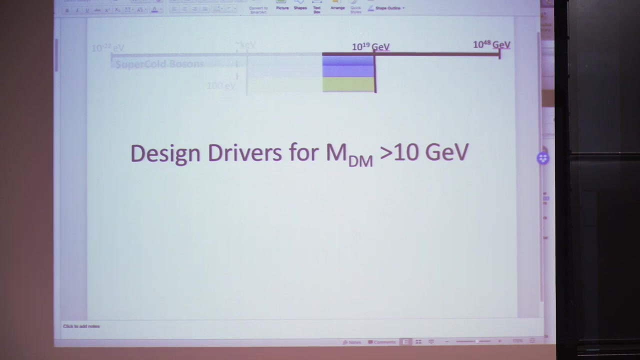 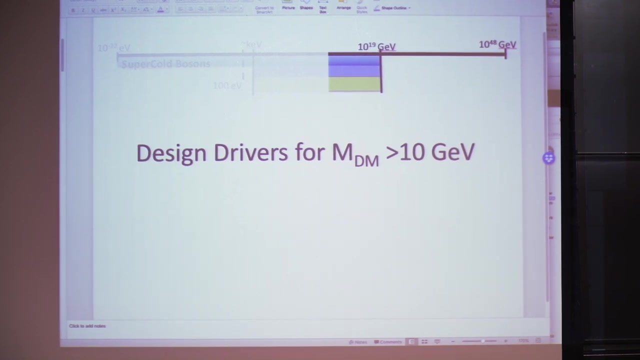 10 to the 48,. oh gosh, I don't, actually I don't think why that's set Up here. this range is everything with like, basically black holes and machos, like massive compact objects. Yeah, no, so that's how you would search for those areas. 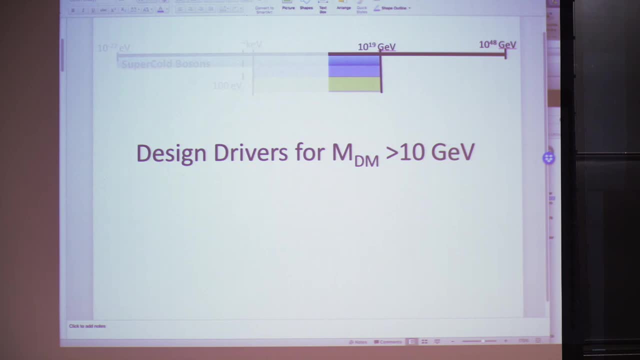 Yeah. so I'm actually not gonna go all the way up, I'm really gonna talk. I'm gonna start my design drivers at the WIMP scale, which, let's say, is below something like 10 TV. So that's where we're gonna start our design drivers. 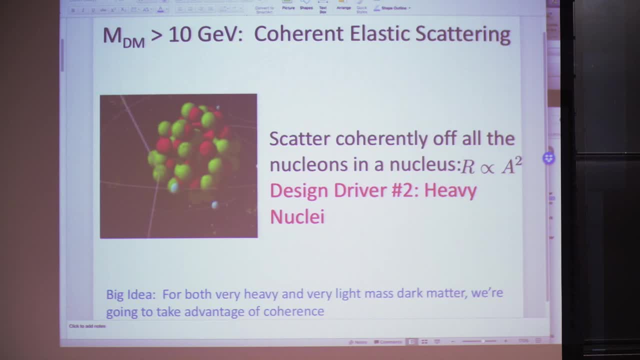 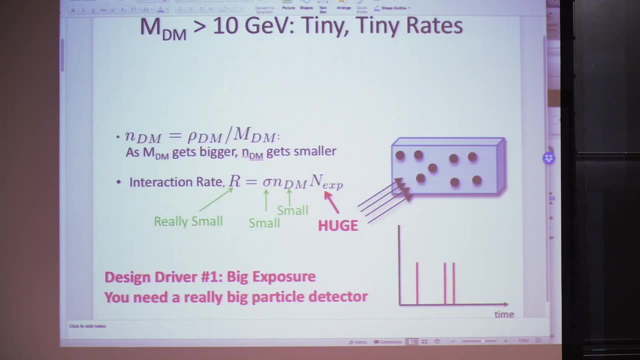 So, oh, wrong way, So let's go okay. so, for 10 GB to 10 TV, I skipped one slide. what's the first thing we have to recognize? And that is that we have really tiny rates, right. 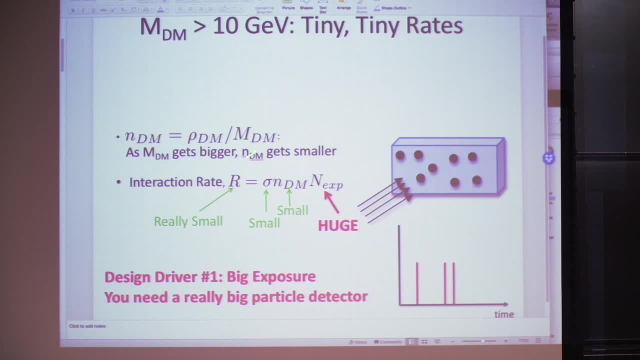 So when we look out at the galaxies we know the mass density for dark matter And then you know if you say that dark matter has something like 10 or 100 or a TV of mass, then you divide through and you get the number density. 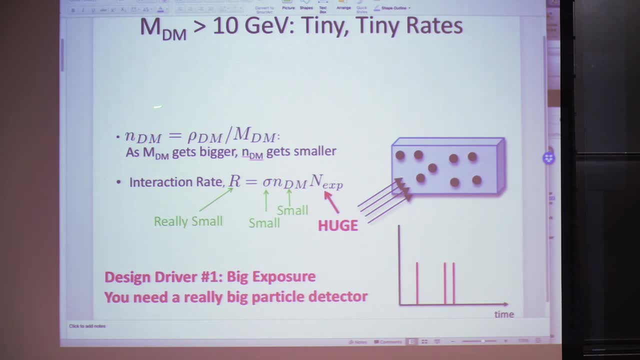 And basically it's just this basic fact that you know, as mass gets bigger, the number, density gets smaller. And now we have this interaction rate, which is gonna be the cross section times the number density times by the number of targets in your experiment. 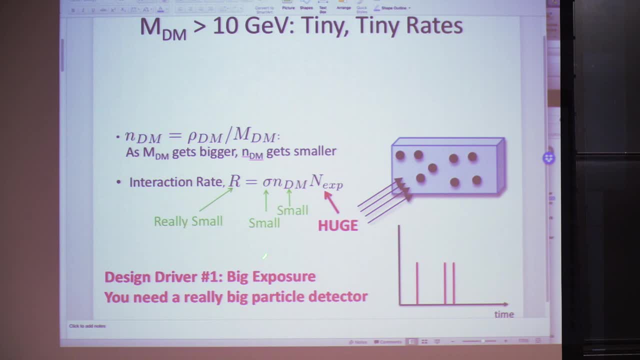 And that's gonna be the reaction rate. So your cross section, you know, is small because it's dark matter. We call it dark because it doesn't interact via all the forces we know. So this is gonna be tiny If your number density is small. 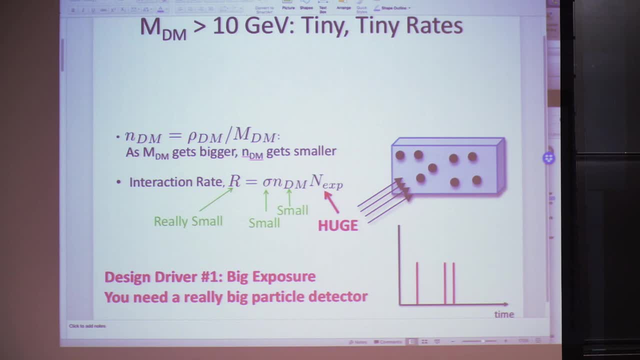 then your experiment has to be huge. so the very first thing we know is that the bigger in mass we go, the bigger your experiment has to be. and so if you know, if you're looking for stuff that's at a hundred TV or or or higher, when you go higher what you have to go to bigger and 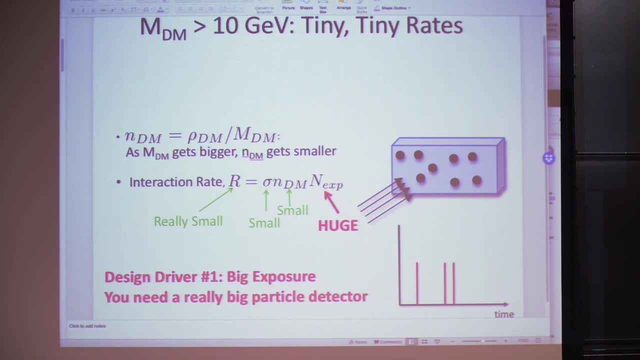 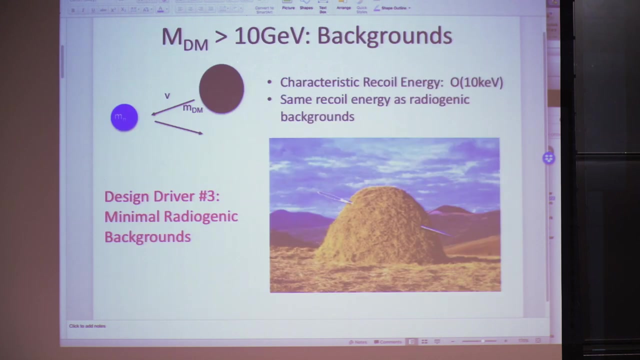 bigger experiments, right? so that's why ice cube is such a big thing. if you want to look for super heavy dark matter, because you need it to be large, so what about? so that's the first design driver that we know for dark matter experiments. ok, so the second one is we want to boost up the delay here, which we're going to. 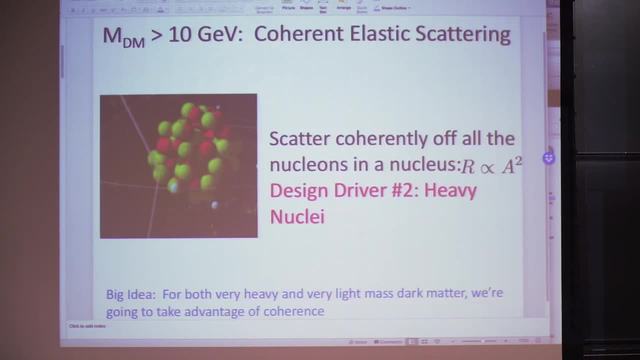 learn. ok, so this? the second one is: we want to boost up that tiny rate and we're going to use this idea of coherent elastic scattering, so we're going to scatter off all the nucleons in a, in a nucleus, and that means that the rate will scale as a. 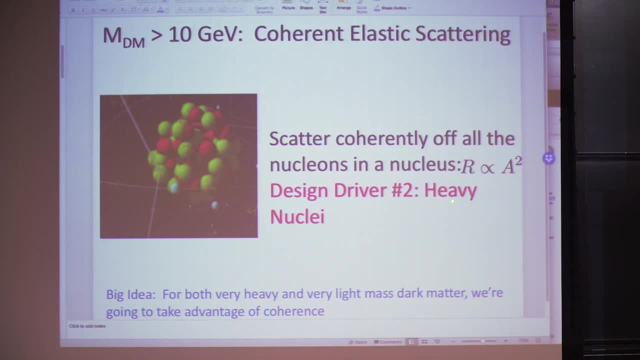 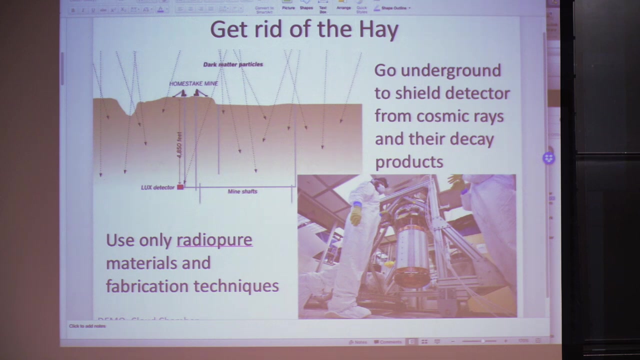 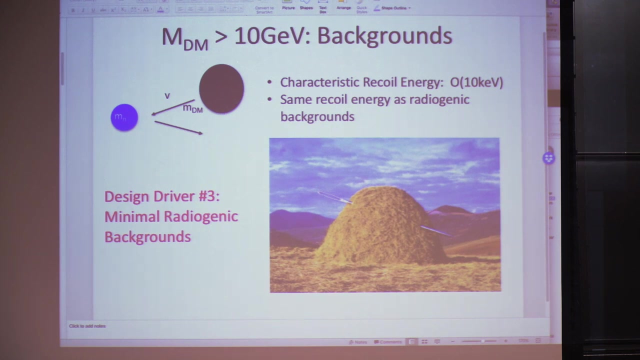 squared, and so that means that the second design driver for high-mass dark matter searches is a heavy nuclei. ok, so the third. we have his backgrounds. so if we just go through the kinematic of this, of the other thing, we have some dark matter particle banging into a 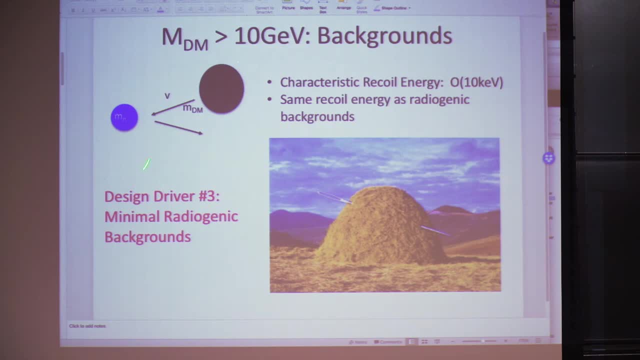 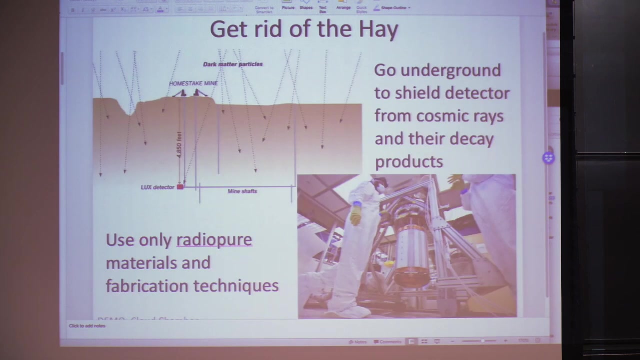 nucleus it elastically scatters. we look at what is the recoil energy here. that characteristic recoil energy is going to be of 10 kV, and 10 kV is exactly the same recoil energy as, like many radiogenic processes, Compton backgrounds, betas. so the third is going to be minimal radiogenic backgrounds. so how? 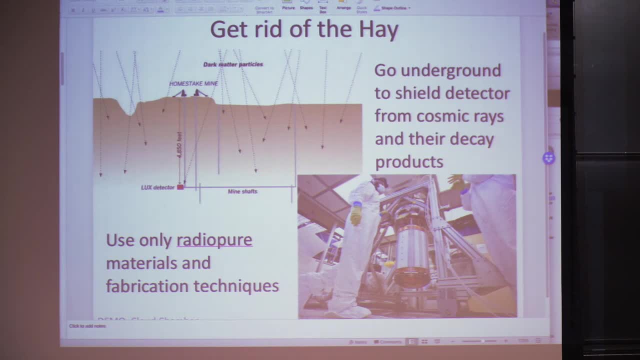 we're going to get rid of that. we're going to go underground. so if we have all these cosmic particles, only highly high-energy protons, flying through, we're going to shield the our detectors with with soil. so we're going to toss, for example, LZ and Lux something. 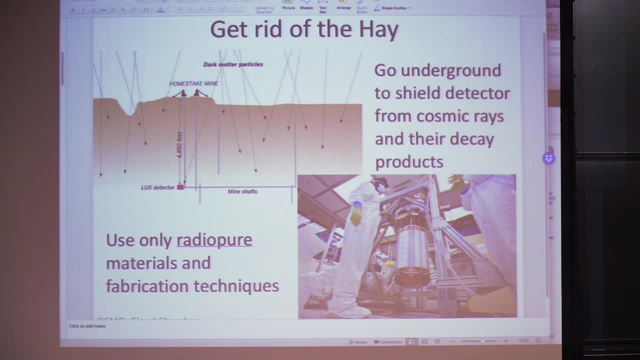 like 5,000 people of the surface. my experiment is at snow lab and it is around six thousand feet below ground. so that's how we're going to get rid of all of these cosmic backgrounds and, secondly, we're only going to use radio pure. 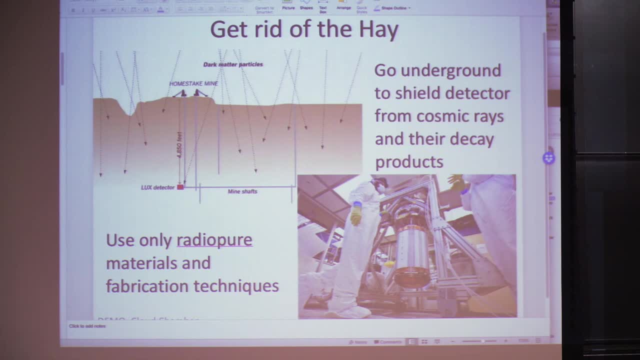 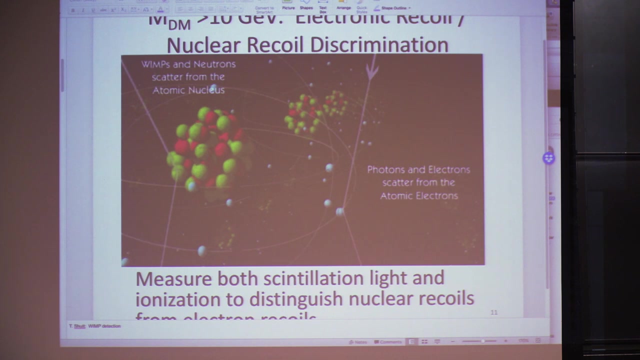 materials and fabrication techniques. so here are people building Lux and you can see the inside is built only out of copper and out of teflon. these are materials that are known to be incredibly radio pure. ok, so even that won't be good enough, because that rate is so tiny and that. 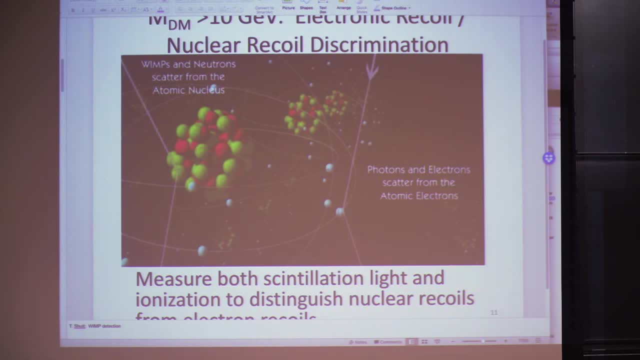 rate so tiny again because there's so few particles going through your detector, plus the Sigma small. so the final thing is we're going to have to. that background will still be measurable. so the idea is, let's try to distinguish between that background and the signal we want to see. so the signal we want to. 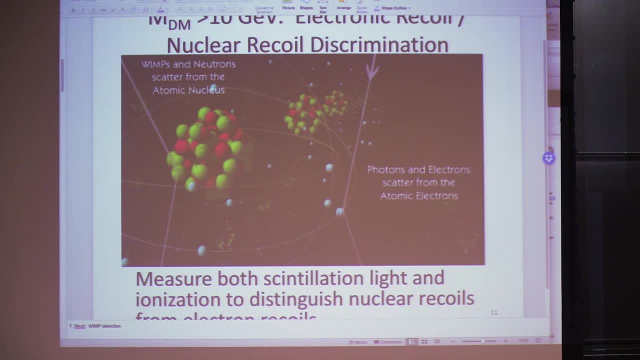 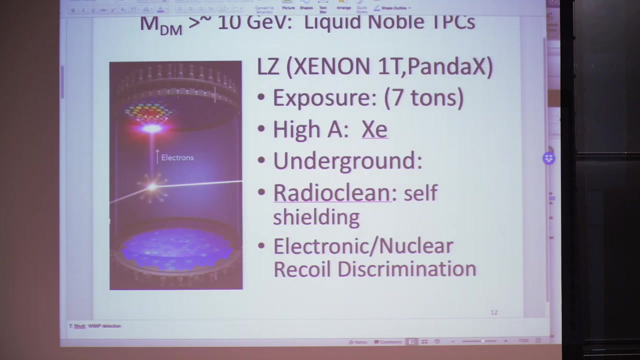 see, is this nuclear scatter and all the background, the vast majority of that background, is actually a electronic scatter. so a photon comes in, scatters off, an electron flies out, an electron shoots out. so if we can distinguish between these two, then somehow we can also drop that background right down. so I- here is a I. 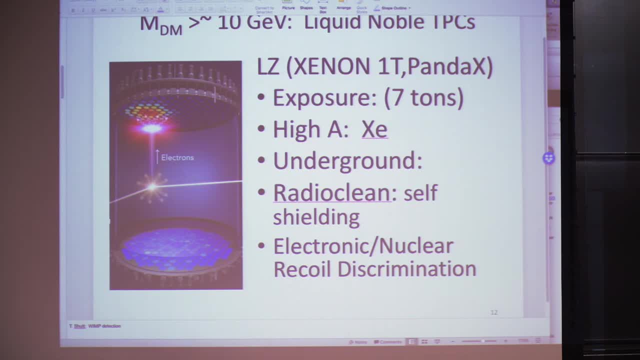 think, truly the perfect detector for for this mass range, and let's just go through why it's a perfect sector. so I, this is LZ, is will be next generation, but equivalently there there's three different collaborations. really, they're trying to build large xenon TPC's and so what is it being on TPC? it's just a huge vat of xenon. so, and by 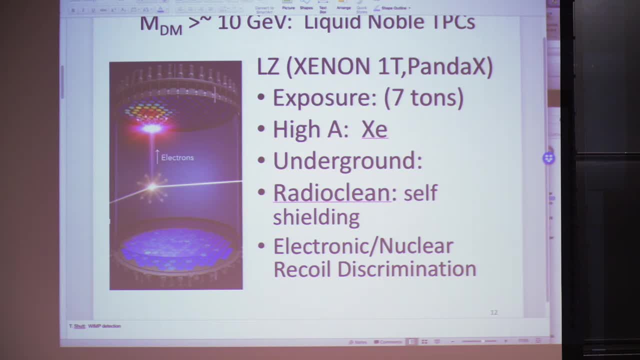 huge. I mean it has seven times right, so it's it's massive. so you, you check out the, the exposure. you can get many years. you have many nuclei. secondly, it's high a. it's xenon. third, we're going to put this underground and xenon itself is. self shielding. so xenon is a noble gas. so noble gases, of course, are noble. they don't interact with anything, and that's this amazing advantage, right? so that means that they don't pick up other materials. they don't pick up uranium and thorium very easily, and they all you can. 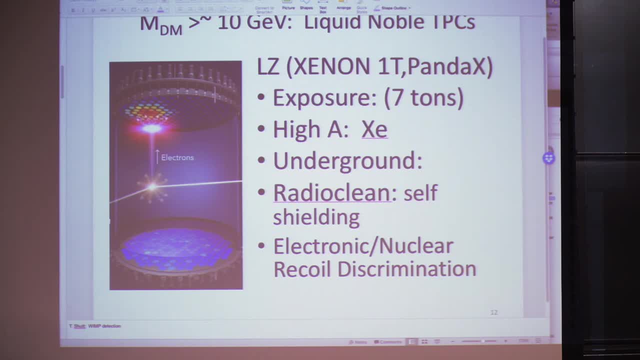 also distill them incredibly easily, right? so I can just go sit at the liquid point and I can distill them. I I can. I boil them off and then collect what's boiling and leave behind what's what's left over and I can make them ultra pure. so because, so that they themselves are. 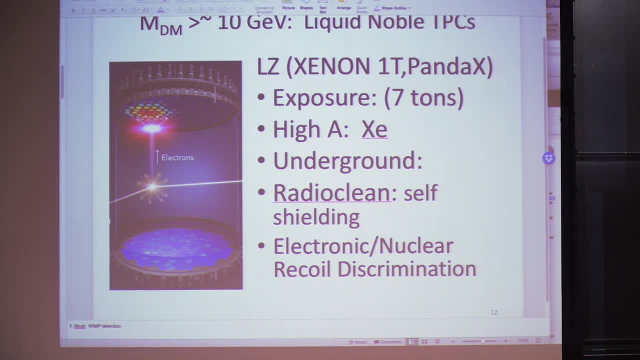 ultra pure. so that means I can use them as a shield from outside photons. so the if I have some I don't know in my material, or let's say a concrete outside of my experiment, and it has some uranium in it, it shoots off a photon. that photon- 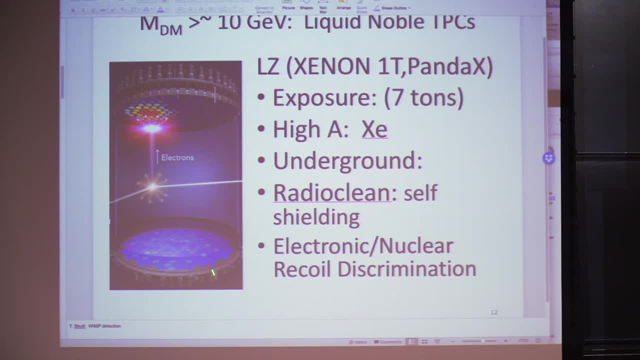 gets in, we can have it interact first with this outer layer of xenon. so we'll never get to this inner fiducial volume where we're going to look for a signal. so we're going to self shield or experiment and protect ourselves from stuff that's outside that produces radiogenic part events with 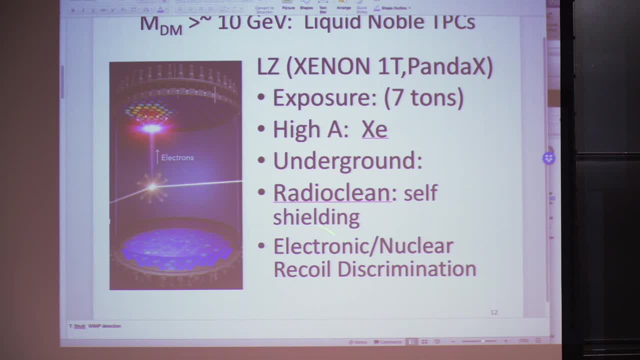 xenon itself. so it's self shields. and then finally it has electron recoil, nuclear recoil, discrimination and the idea. there is, as we measure, two different signals. so when this particle comes and interacts, it does two things. so first it immediately produces some scintillation photons and those bounce. 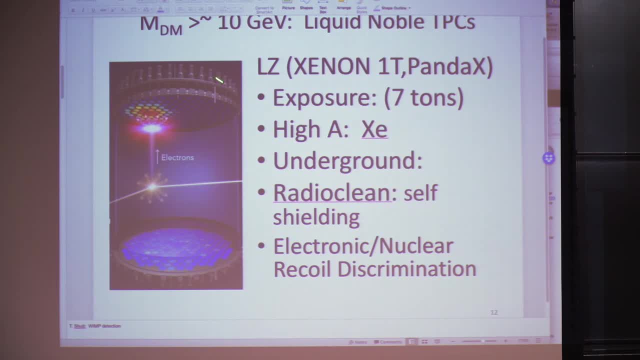 around and and they eventually end up in either the top or bottom PMT sensors. almost all of them actually end up in the bottom in the s1. so secondly, it produces some ionization and if you put a huge e field across this system, then the those electrons are going to drift and they're going to drift up to where. 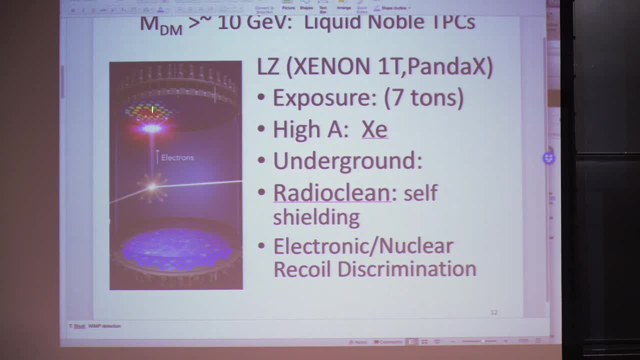 they get to right here and in this region we're going to have a little bit of a gas gap. so we're going to have, you know, a centimeter or two of xenon gas with a high e field across it, and when that electron gets into the xenon gas now, it can accelerate very. 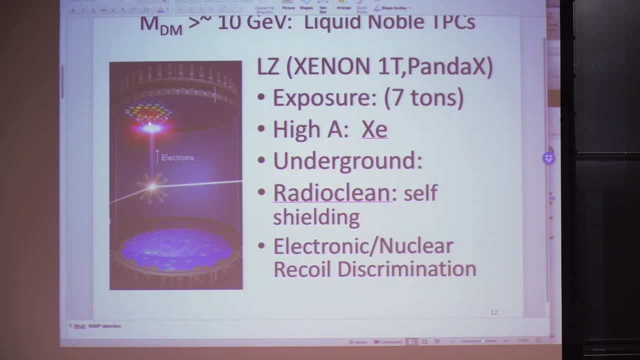 rapidly and get the very high kinetic energies and then when it hits one of those xenon gas particles it'll shoot off lots of scintillation. so you're, you're taking the kinetic energy and that kinetic energy of that particle and you're converting it into into scintillation right up here. so and 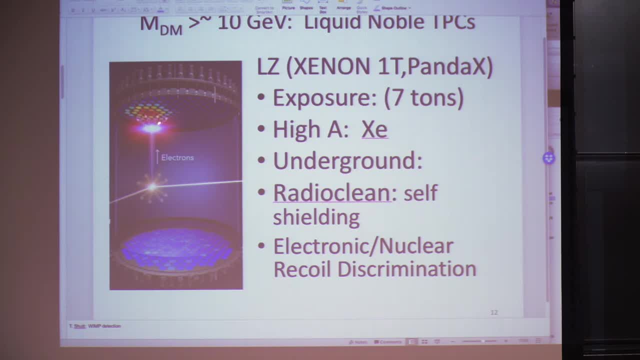 so you're basically converting the number of electrons you see into scintillation, which is a second pulse, so you get these two different pulses. they're separated by time so you can figure out exactly how much scintillation one produces and how much ionization one produces, and it turns out that electron 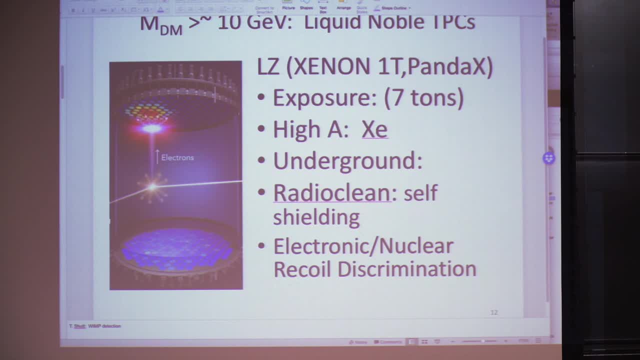 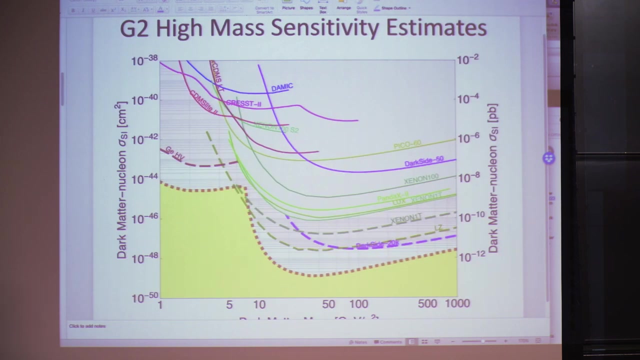 recoils and nuclear recoils produce different ratios of those, and you can pick it out. so I think what we just saw was we saw that it was amazing how perfectly this detector matched our design drivers, and you see that here. so over the last, you know, 20 years, we've 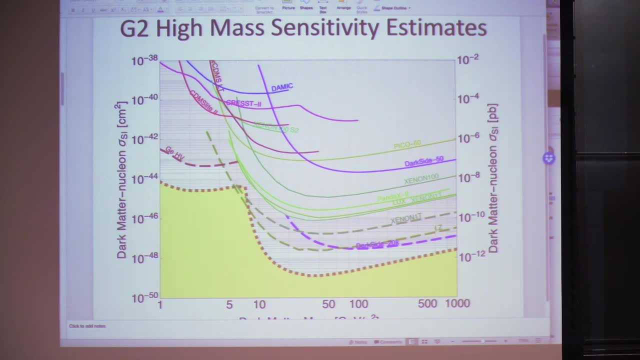 been searching for, for WIMPs and something like you know. every five years we get another factor of 10, which is an enormous amount of sensitivity boost. it really has been an exciting time and we're about ready to get another one of those five factors of many boost as we go from this. 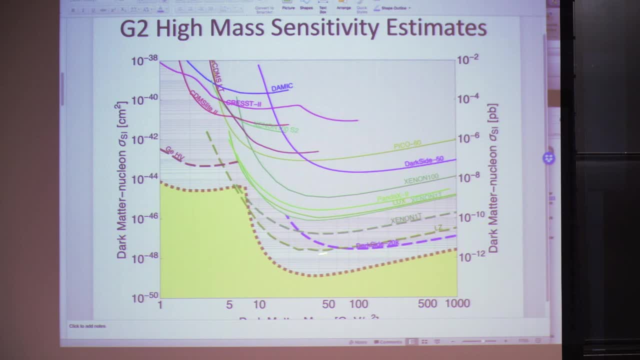 age of lux, xenon, one ton and panda, and we bump up to LZ, which will be coming on in 2020. so we should see this factor of you know something like 20 to 40 improvement in sensitivity over now in the next two to three years. so the x. 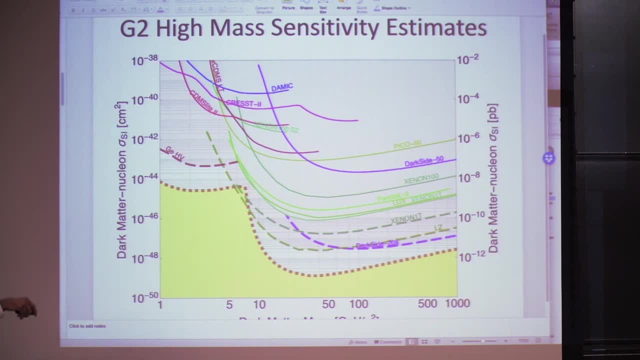 axis. here is- I'm sorry, yeah, you can't see it because my slides cut off. the x axis is mass, so we have one to a thousand. so you see, this works very well above this 10gb threshold. and so, finally, a few more points. this yellow. 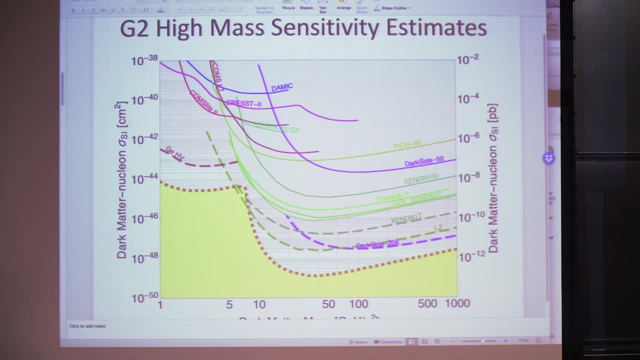 here is a neutrinos from the Sun. so you know. so we have neutrinos coming in coherently, scattering off of nuclei, the same nuclei. so it's a nuclear scatter, so it looks just like a dark matter scatter and that's going to set the floor. 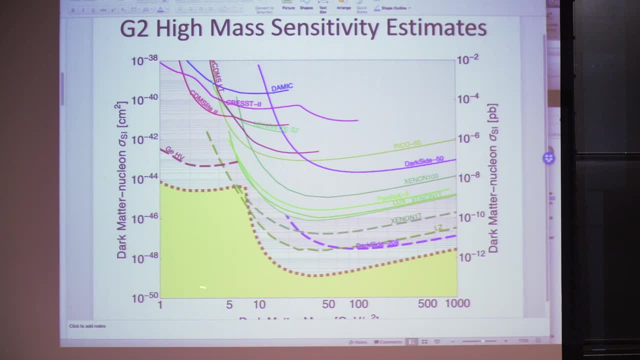 throughout this entire process. uh, up here these are neutrinos created by the atmosphere. here this is boron-8, which are neutrinos from the Sun in this range. so that sets the floor, basically, for these limits. now there are all. there are people who suggest that we 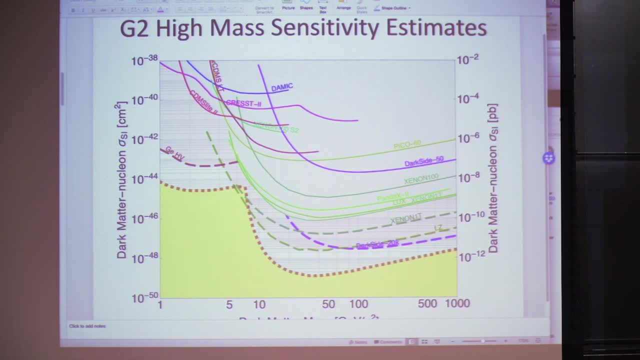 can go below the floor using directionality. I won't talk about that today. that's definitely challenging. I here let's concentrate just about getting this another, you know two or three orders of magnitude from where we are today to this range here, and that's certainly accessible. 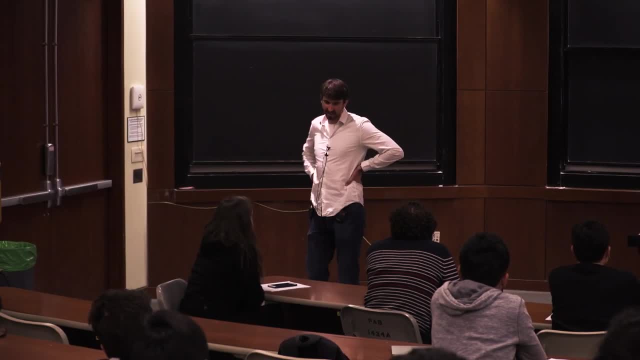 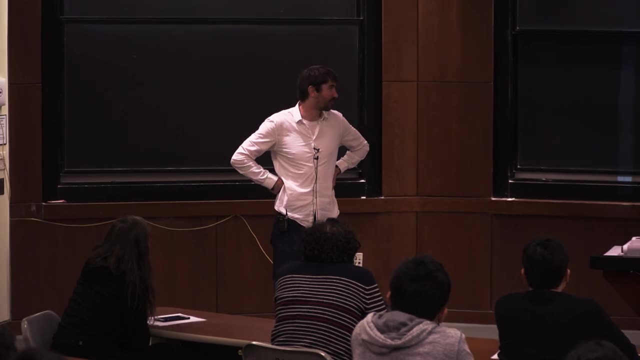 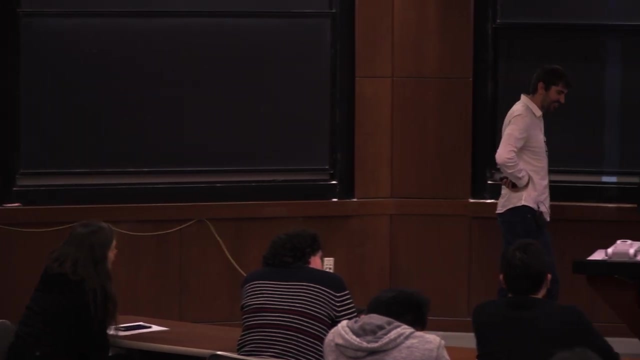 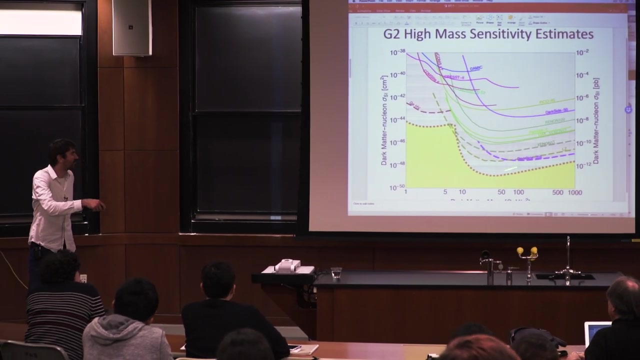 yeah, yes, yeah, yeah. below that, you have to somehow come up with a technique to separate nuclear scatters from dark matter, from nuclear scatters from neutrinos. so so when certainly are not dead, oh, yes, yeah, yeah, yeah. so the question was: what sets this floor? and it's. 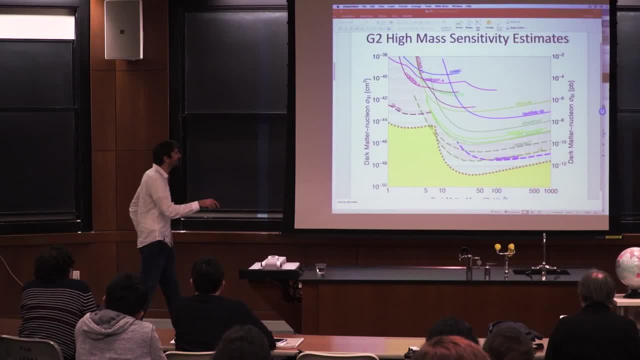 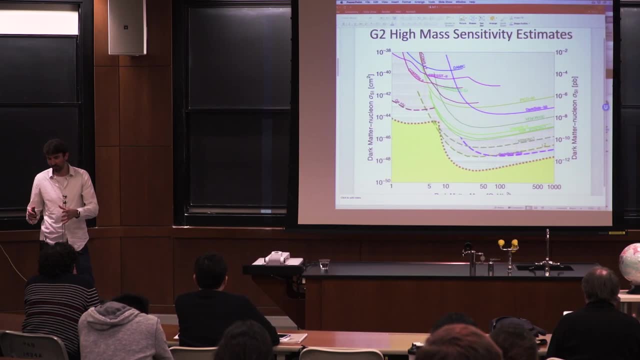 purely an experimental floor. we would love to keep on going down and mass and you know, in some sense xenon is just a big, giant vat. so with enough money one could just make these things bigger and bigger in theory, and so potentially that would be possible to. 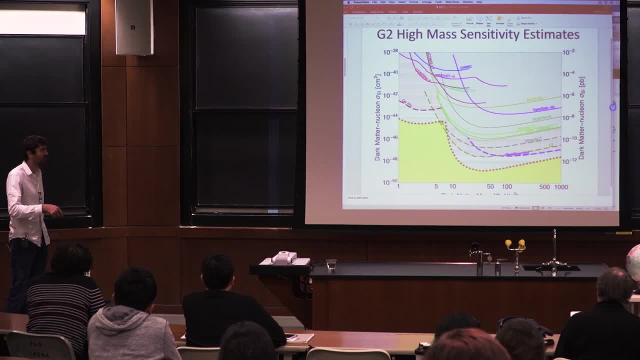 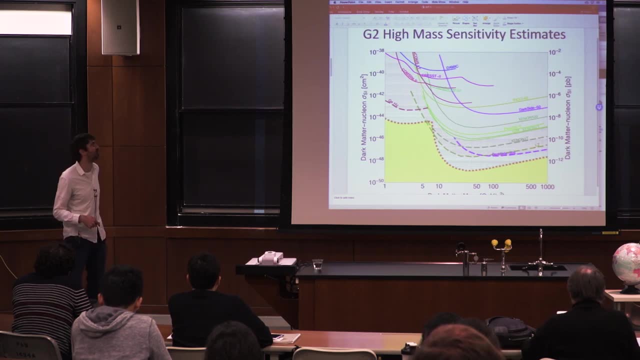 keep on going down. the problem is, we have this fundamental neutrino background and one has to come up with schemes to separate those two out. and you can't. you just use electron recoil, nuclear recoil, rejection, And you can't shield them because of course neutrinos go through everything. 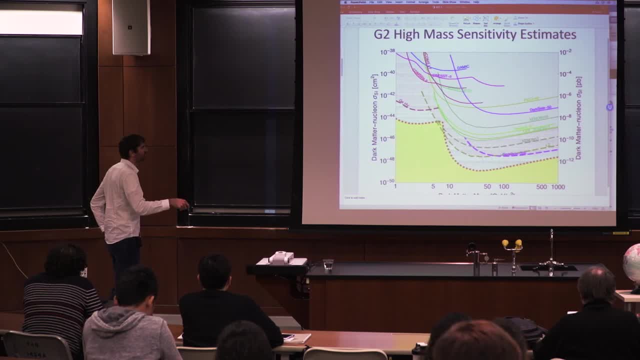 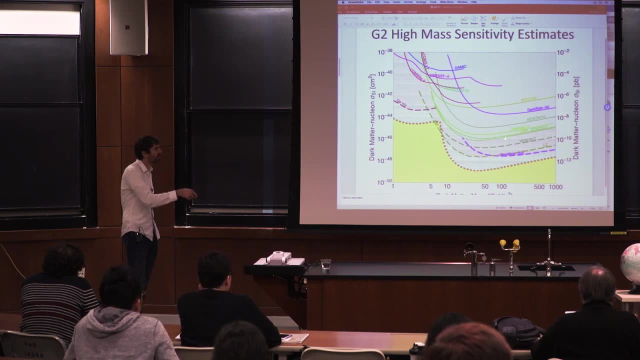 So that is a challenging region, but we still have this huge range of, you know, something like three orders of magnitude from where we are right now to this range here. So it's yep. I'd like just to make a remark. 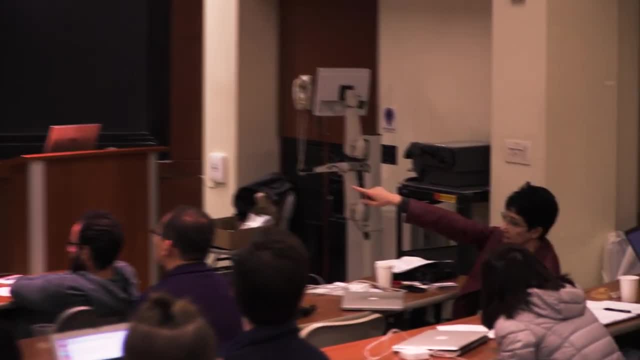 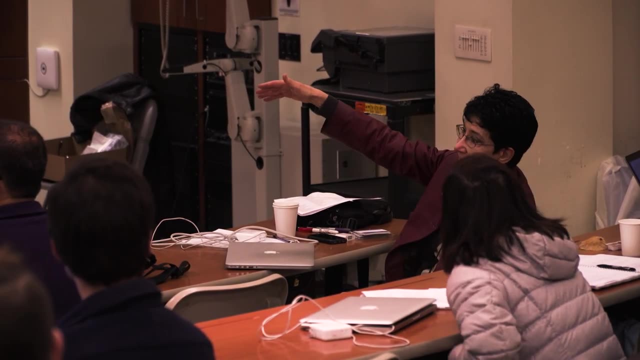 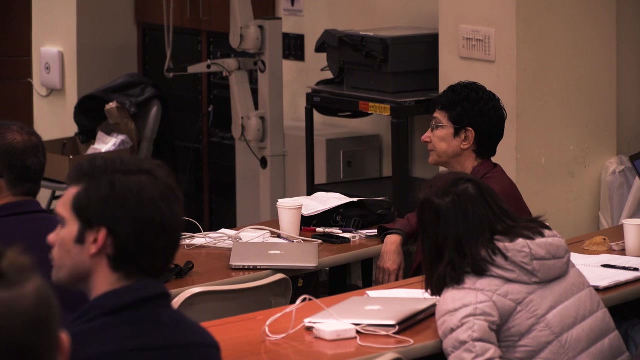 As you say, this is for spin-independent interactions. The degree of degeneracy with neutrinos of course depends on the type of interactions of the dark matter. So this is for spin-independent. Sure, sure, But of course No. but you of course pay like the vast. 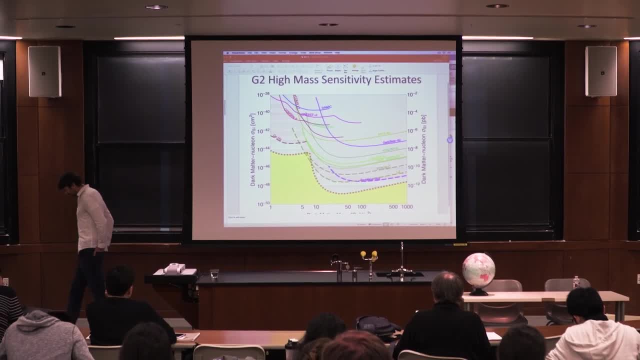 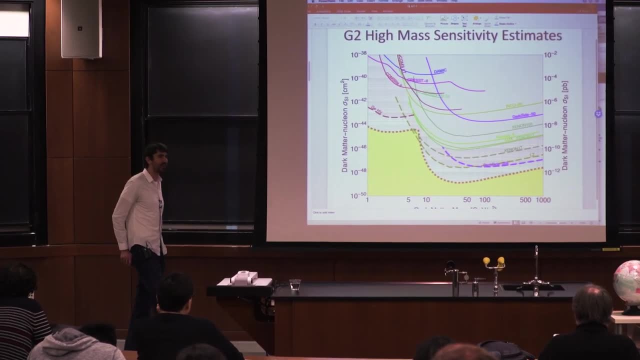 It will have a background. Yeah, yeah, How difficult it will be depends on the type of interaction. Yeah, no, and also, I mean, the reason why we go to spin-independent in the first place is because we have this nice coherent rate enhancement right. 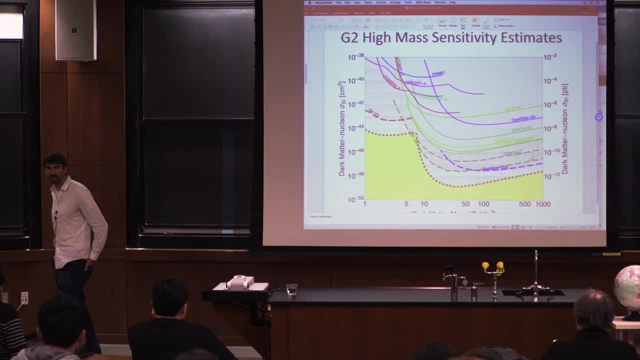 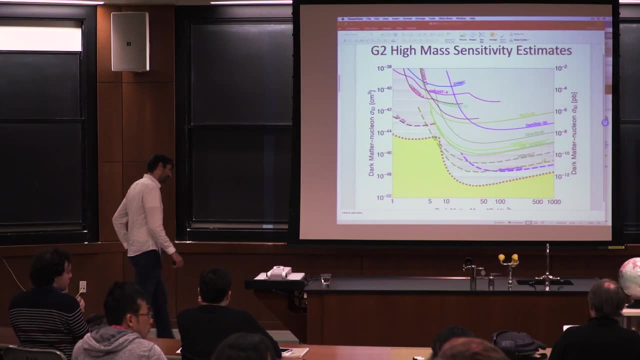 And so when you get away- when you get away from spin-independent, you go to spin-dependent and other effects- you always pay a rate penalty that's pretty vast. For example, if you have something much more exotic than that, you could have a coupling through a dipole moment. 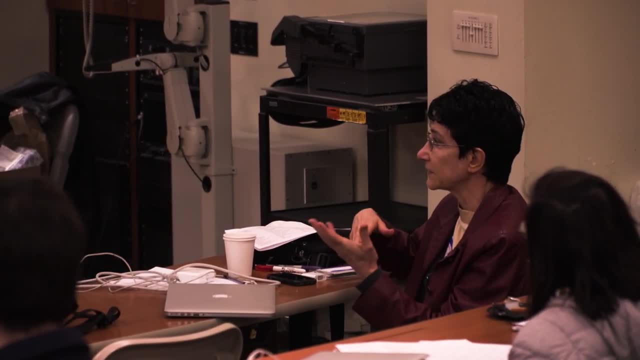 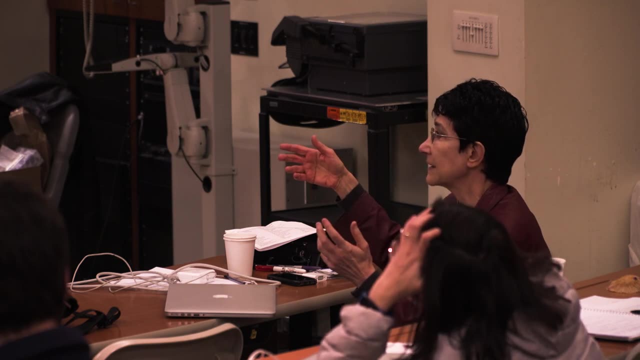 for example. And then you will have a partial you are coupled to the charge. Partially you are coupled to the magnetic moment of the nucleus. Yes, The spectrum is different, It looks different, Yep. So you don't have any longer degeneracies. 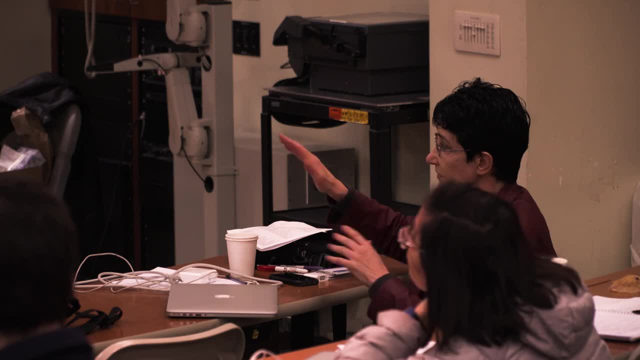 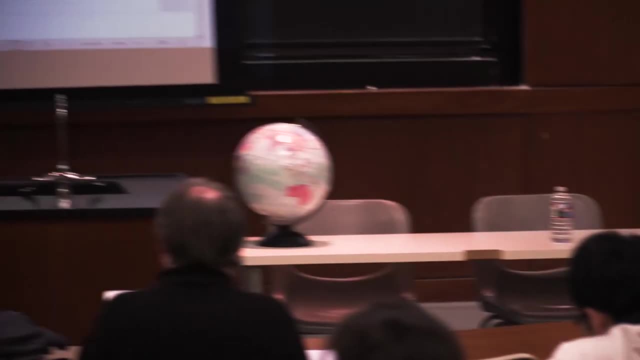 with some of these interactions. In any case, if you're going to go there, then we can discuss. Yeah, yeah, yeah, I'm not going there, But yeah, and I think all those experiments are really getting challenging because you are going below 1. 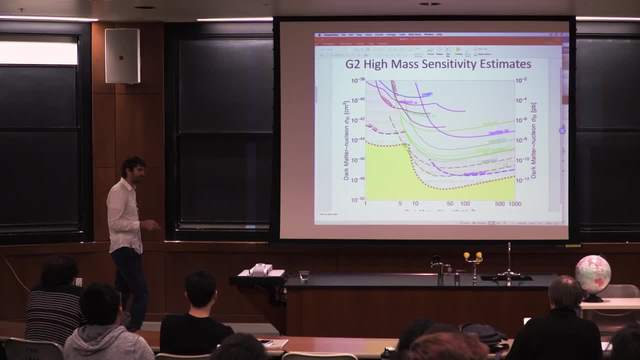 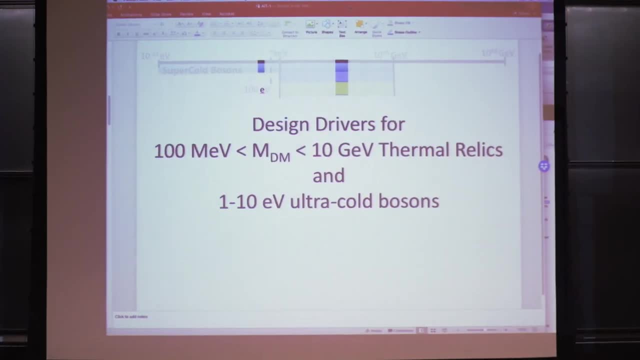 e to the minus 48, right, So like, but we can talk about that later. OK, so now we're going to go down in mass And we're going to look at that: 10 GeV to 100 MeV. 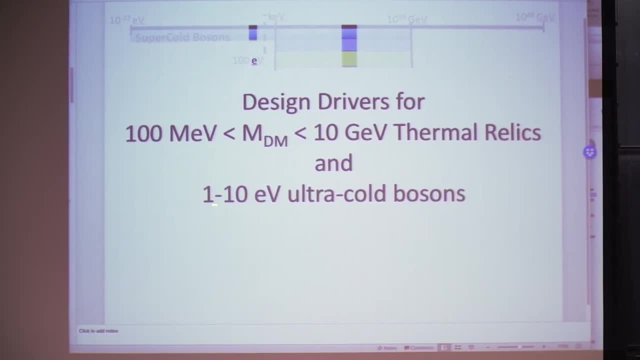 And at the same time we're going to pick up, because the energy scales are similar for nuclear recoil scattering and for absorption. The same experiment can be used for 1 to 10 eV ultracold bosons, where we absorb onto the system. 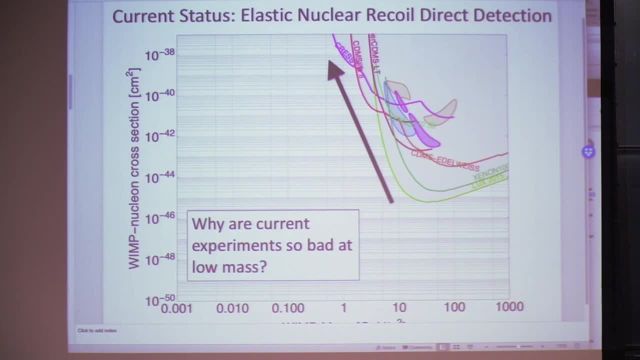 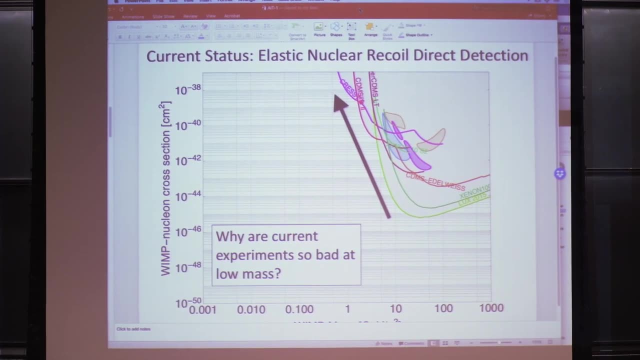 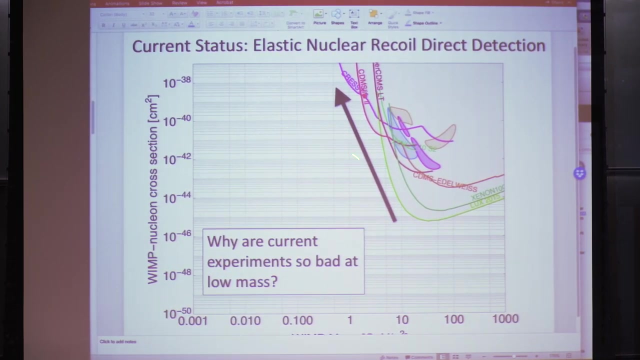 So in this range, let's think about what happens. So here are basically all of those current experiments that we make, And what we see here Is that none of those experiments have any sensitivity to dark matter in this range, And we can just ask why. 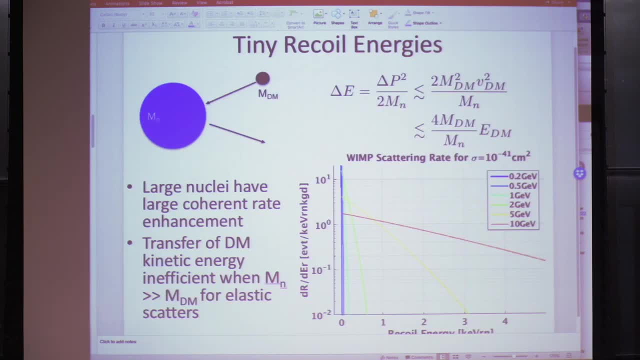 And the answer is: it's pretty simple. We have this giant nucleus here And we have this very tiny dark matter particle which has much less mass in the nucleus And it's elastic. so it's literally like throwing a bouncy ball against a wall. 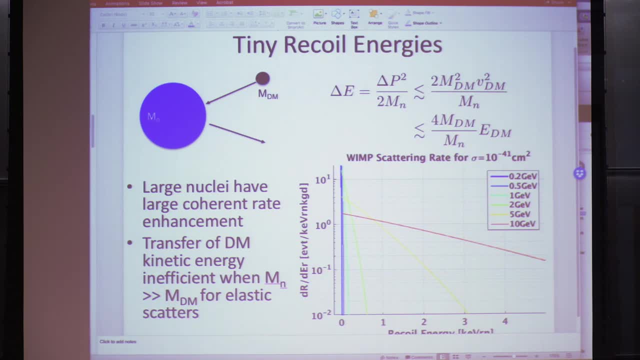 So the wall is much more massive than the bouncy ball. So you toss it against and almost all the kinetic energy stays with the ball And very little is transferred to the wall. To have maximum transfer, you want to have the masses exactly the same. 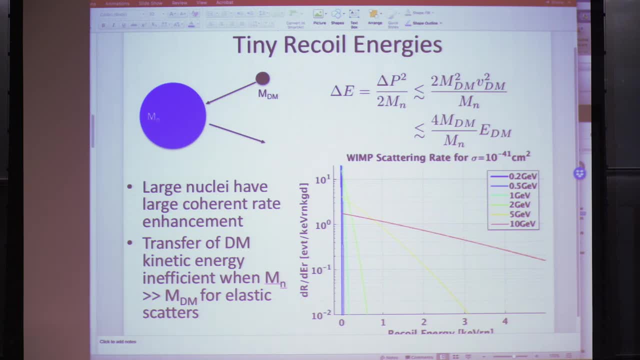 So this mass will go in, hit this one and it'll bounce off. So this kinematic mismatch between these, we can actually see what is the characteristic recoil energy scale for transfer, And that's delta E is just going to be the recoil energy of this nucleus. 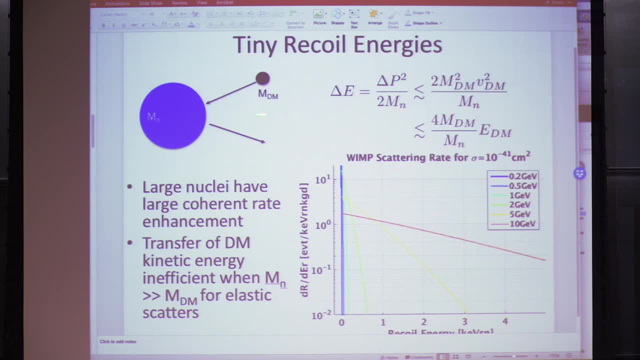 will be approximately the momentum transferred between the two particles. So that's just delta P, And if the particle is going in this direction and it kicks back or in this direction, that's approximately just 2 times the original momentum of the dark matter. 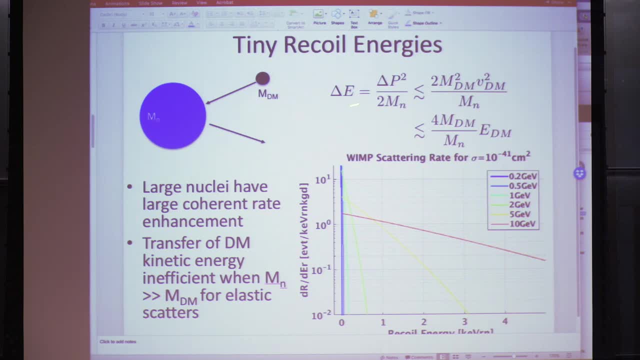 And then you have divided by 2 mn. So we see that the characteristic recoil energy scale goes as m squared of the dark matter. And then we have turned that down to m squared. So that means that as we drop down in magnitude we go down in characteristic recoil energy scale. 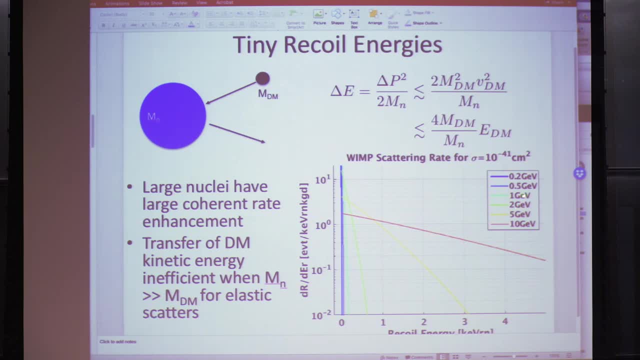 by two orders of magnitude, right. So here we have, like I don't know, a 1 GeV particle. This is the recoil energy scale And that's giving you in germanium, it's give you something like a 100 eV of recoil energy. 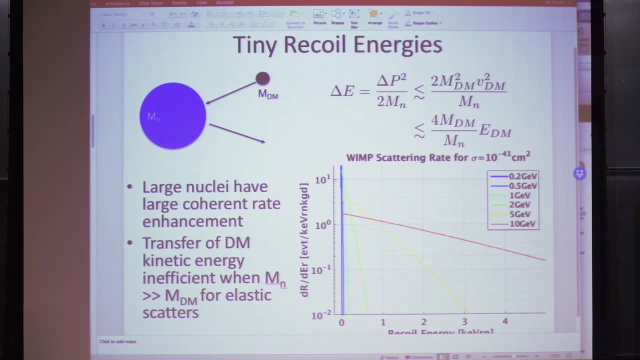 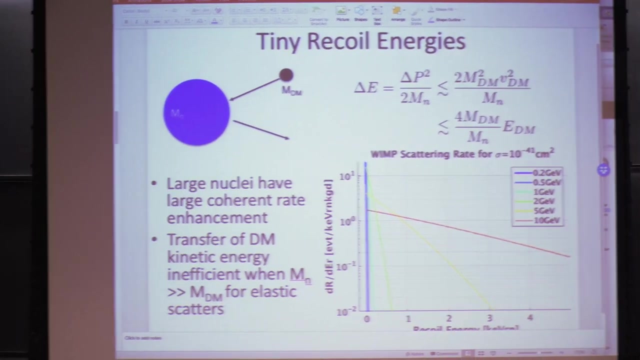 down to 0.1 GV, so 100 MeV. I lose a factor of two orders of magnitude and I'm now at something like 10 mEV. Yeah, Can you extend this off by going to the inelastic scatter? 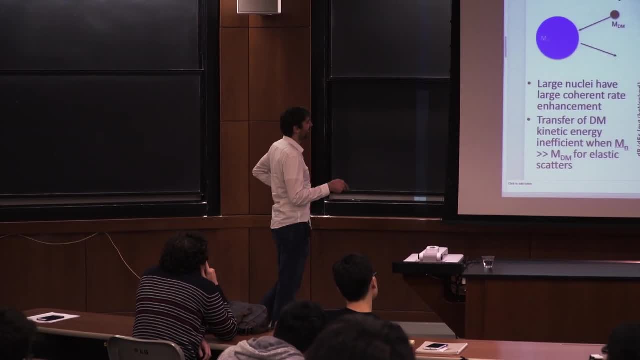 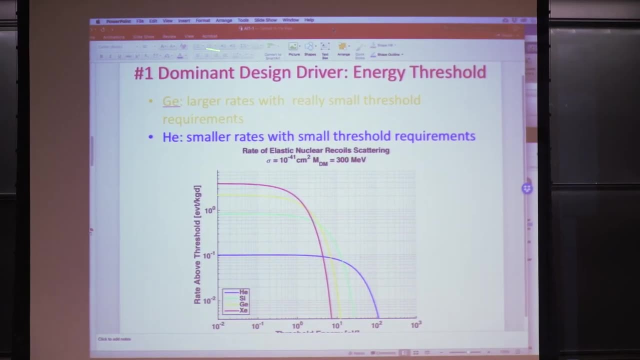 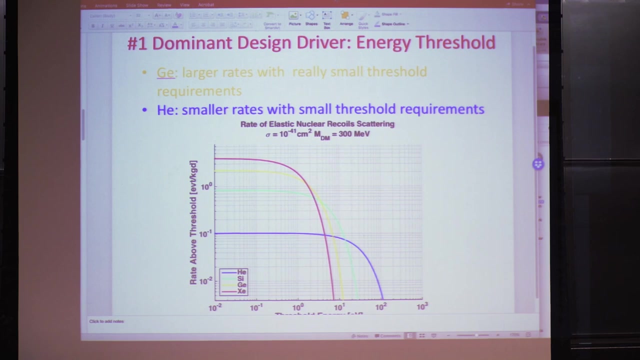 I can, yeah, So we'll talk about that in a bit. So the moral here is that for this range really, the dominant design driver is energy threshold. So this is in contrast to in the high mass range, where we found that the dominant design driver was really just. 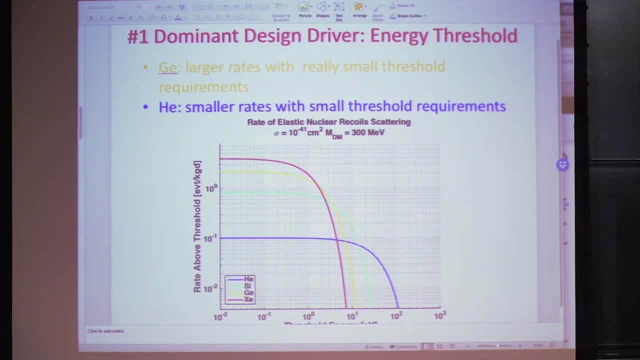 you needed to have a big thing right. You needed to have a huge detector Here. you don't need to have that. The real key is you just need to have a really excellent energy threshold, And now we can play with two different nuclei. 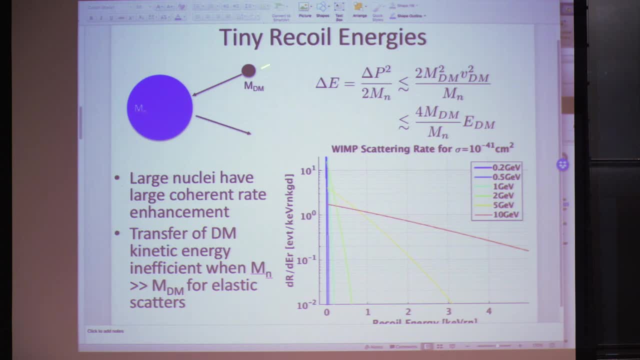 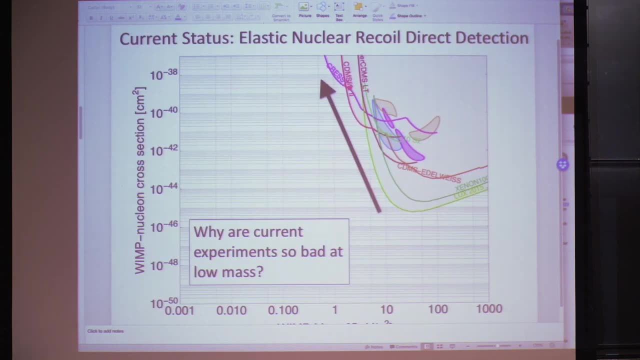 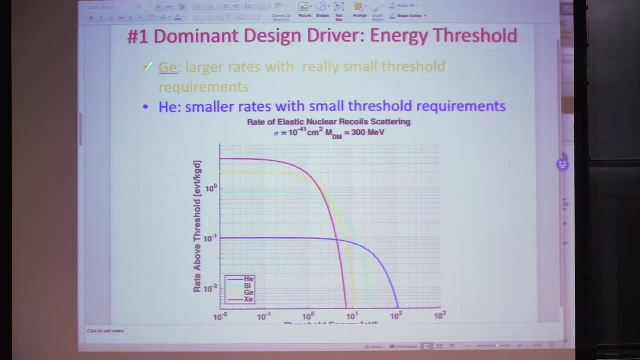 So here we have this Mn, So the kinematic mismatch: the bigger the nuclei, the bigger the kinematic mismatch. So we can sort of play back and forth with this, And so we can play back and forth with that and we can say that germanium has a bigger a squared. 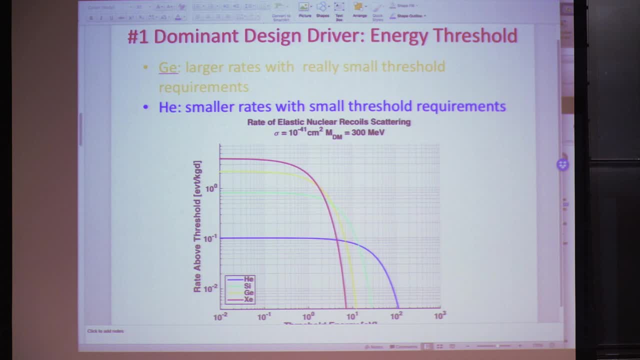 so a bigger, coherent- It's a coherent- rate enhancement, But the kinematic mismatch is going to be much more vast. So you're going to have, if you have really small threshold requirements, you can have larger rates, And with helium, on the other hand, 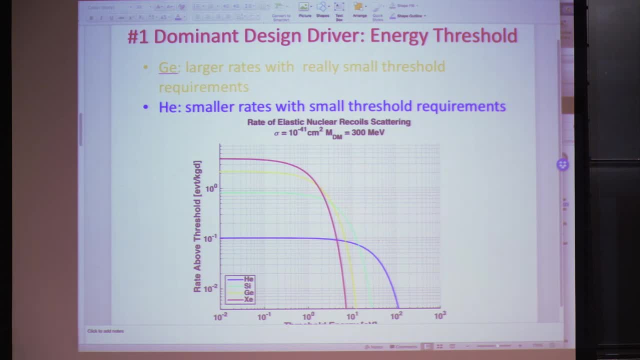 it's on the opposite end of the spectrum, right. So there, your a is 4.. So there you are going to have smaller rates because you don't have the coherent rate enhancement. That's here in blue. But your kinematic mismatch isn't as bad. 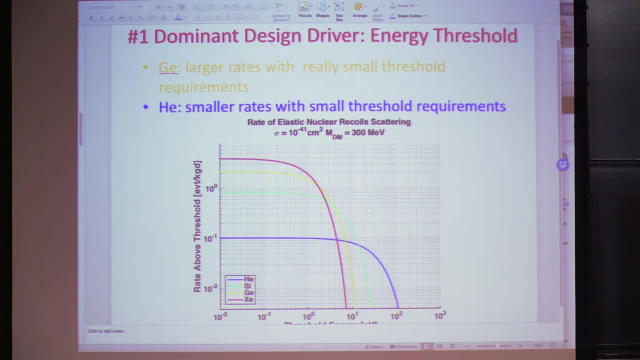 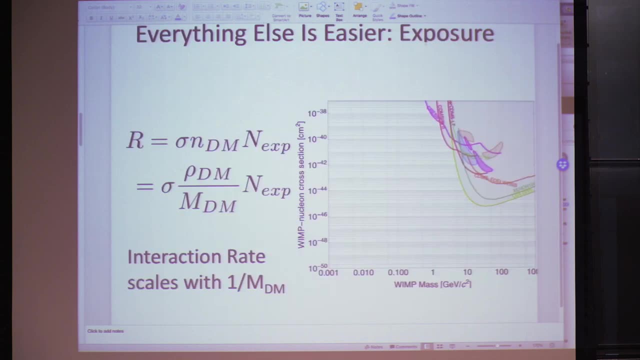 So you're going to have higher kinetic energies. So that's sort of, You can play the rate enhancement versus the energy threshold back and forth, So everything else is easier, right? So here is that exact same idea of the rate that we had previously. 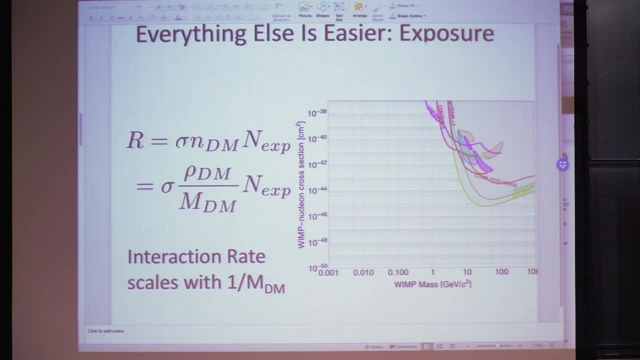 And because it scales- so it's sigma- the cross section times the number density of dark matter times by the n exposure And because this scales as the mass density divided by m, we see that the interaction rate scales as 1 over mdm. 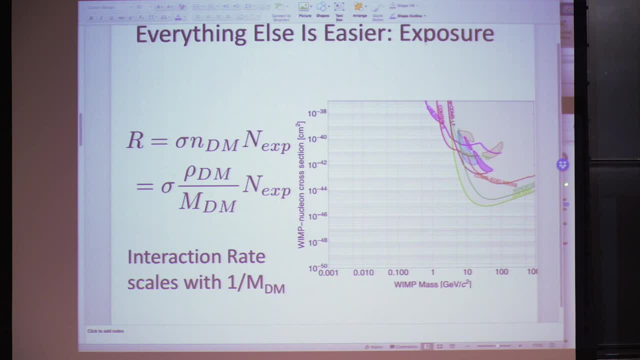 And you actually see that in this plot right here, of all of our dark matter limits from, let's say, LZ and stuff, They have this 1 over m dependence that as long as you are still sensitive to all of the particles, all the interactions that are going, 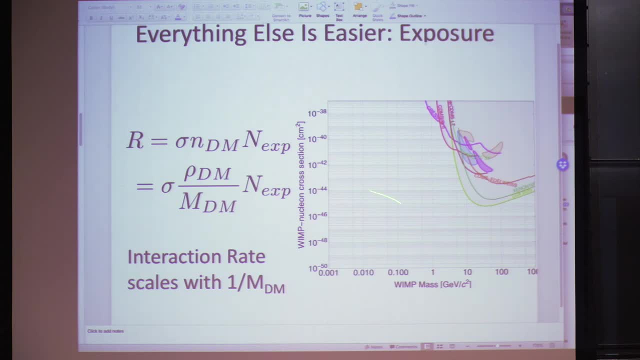 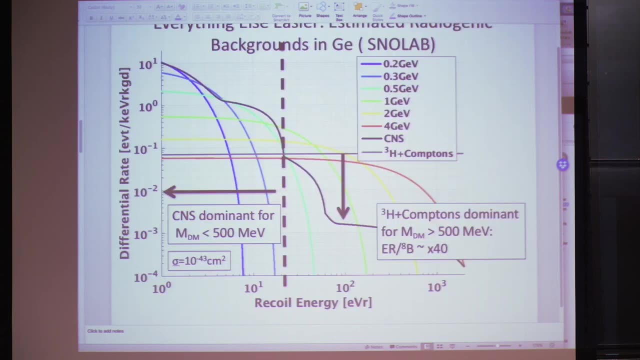 this has a 1 over m scale, So as we go lower it gets easier for us to see things for a given size experiment. So that's awesome. Secondly, let's talk about backgrounds. So that third design driver that we had for LZ was backgrounds. 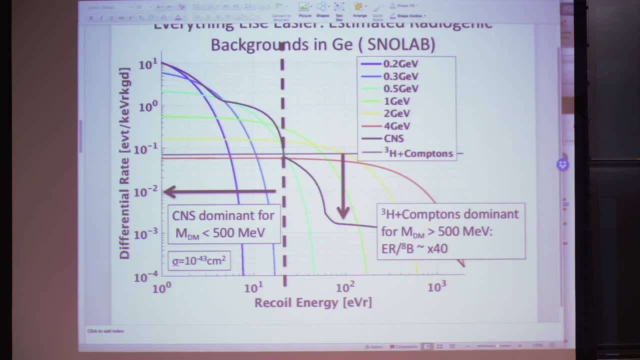 We had to somehow minimize backgrounds. So let's think about how that happens here. So here it's a little bit of a messy plot, but let's see what it means. So here is that Compton background rate. This is the electron recoil background rate right here. 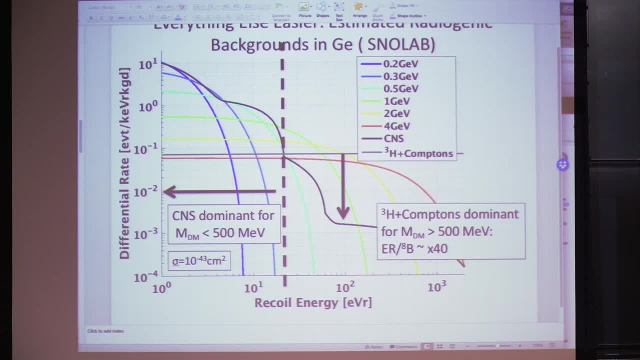 And it's something like at 0.1 DRU. so 0.1 event per kV per kilogram day For germanium in basically a pretty good cryostat. that's been carefully done, but not extraordinarily so. And here then is this coherent neutrino scattering floor. 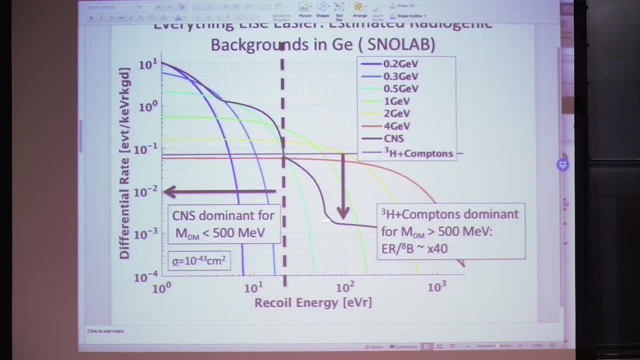 that we see This right here is our boron-8 floor from neutrinos, from boron-8 in the sun, And you can see that to go from here to here it's something like a factor of 40. So that means to do the ultimate experiment in this range. 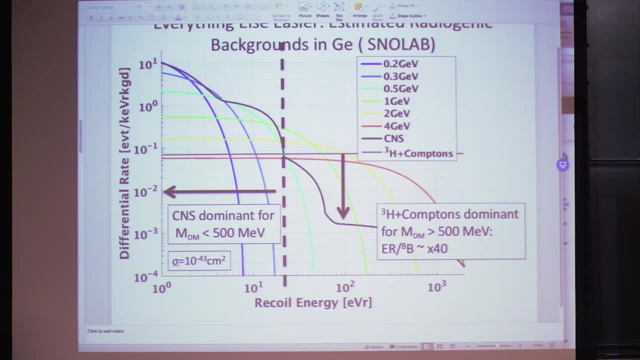 from 100 MeV to 6 GeV dark matter one just needs. if you use germanium, one just needs something like times 40, electron recoil, nuclear recoil, discrimination, And in colors. by the way, here these are just some spectrum for various mass: 0.2 through 4 GeV. 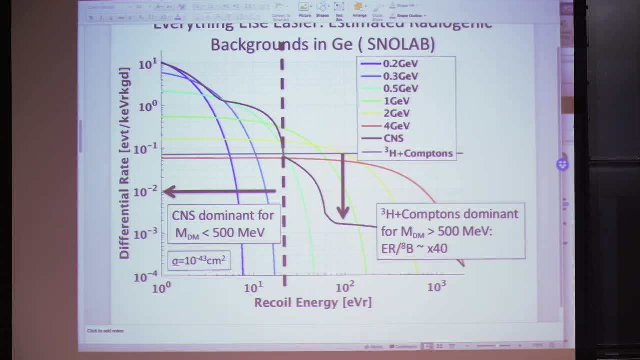 And you can see that, And you can see where this cross-over occurs. OK, So that means that roughly in that region. so let's just look. So right here, the cyan is where you actually see the cross-over between the neutrino background. 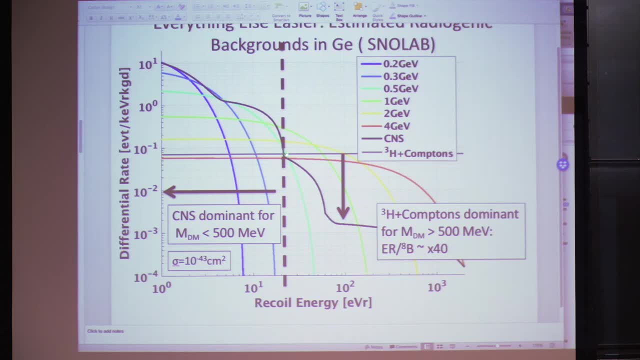 from coherent neutrinos from the sun and the Compton. So above this cyan, so above 0.5 GeV, you're basically going to need some amount of electron recoil and nuclear recoil discrimination to hit that floor, the neutrino floor. 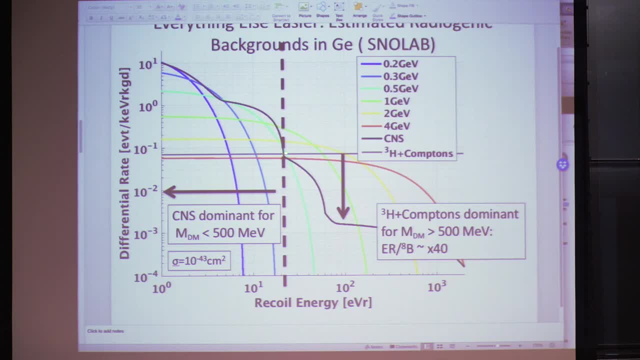 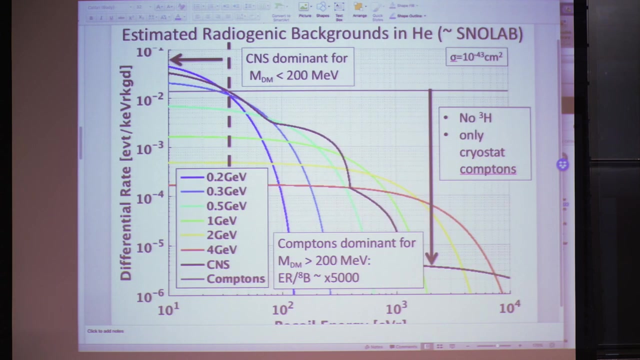 OK, All right, We've talked about this before. Above, below, something like 500 MeV. you don't need any discrimination at all. You'll just hit the floor automatically. That's your fundamental background. OK, So now we're going to do the exact same thing with helium. 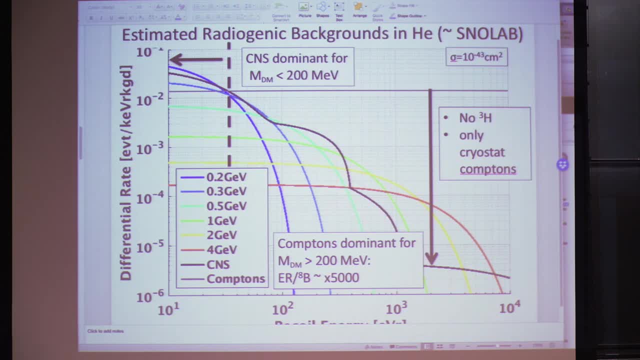 So we just talked about helium and we said that helium has less coherent rate enhancement. So that means: but the backgrounds are roughly the same because the Compton background just scales with the amount of electrons in your system. OK, So the amount of electrons, the amount of protons. 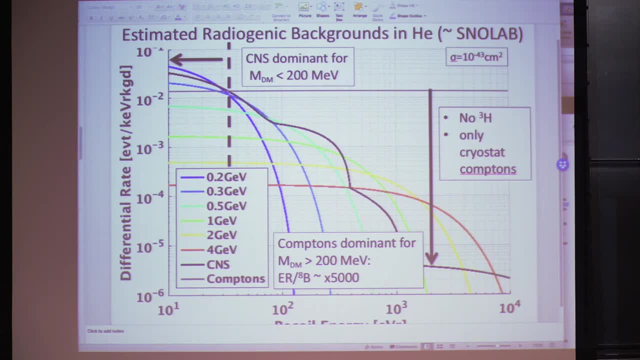 in your system. just scale with the mass, basically. So if I have a kilogram material, we have some number of electrons, if it's xenon or if it is helium- And actually I have more in helium- just because the proton-neutron ratio is slightly worse. 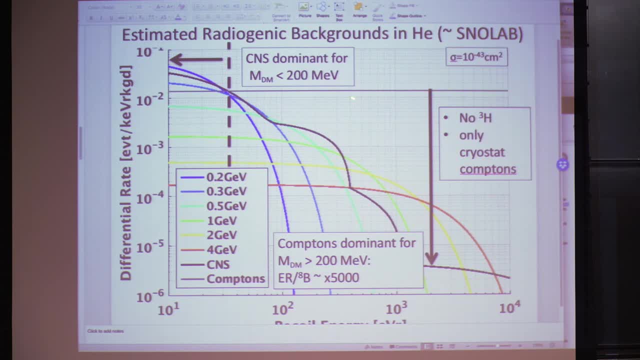 So that means that what we see here is my signal is suppressed, but my background is not. My background on a per-kilogram basis is roughly the same. It's actually slightly better because there's no tritium backgrounds, there's no beta backgrounds in helium. 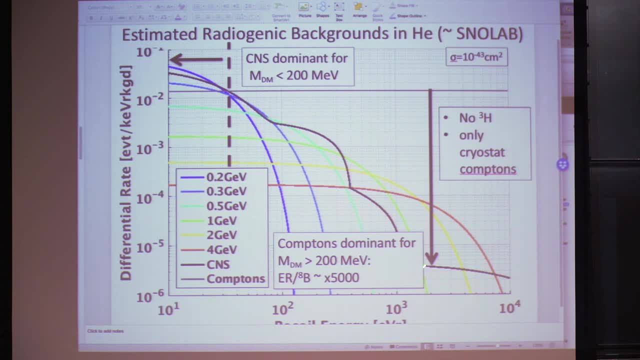 because we can make it so clean. It's a noble gas, But in helium that signal suppression means that to hit the boronate floor we're going to need a lot of electron recoil and nuclear recoil rejection. We're going to need something like times 5,000.. 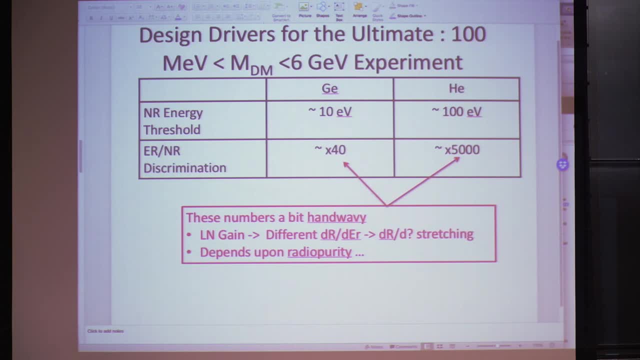 So that's the trade-off in this range that we're going to have for an ultimate experiment. So for the ultimate experiment we're going to have to have something like a nuclear recoil If it's out of germanium or out of any kind of high-energy. 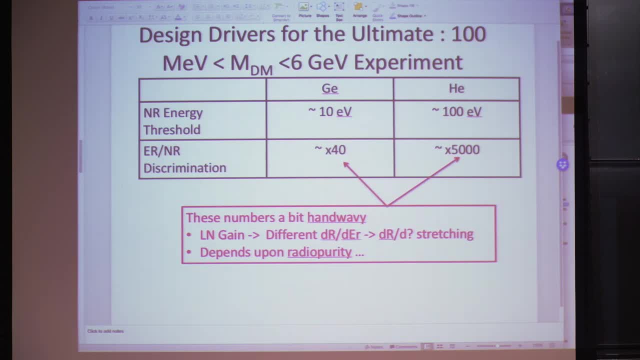 material, you're going to have to have a really low nuclear recoil energy threshold. But you won't need that much ERNR discrimination If it's out of helium. by contrast, you can have a much. your energy threshold can be much higher. 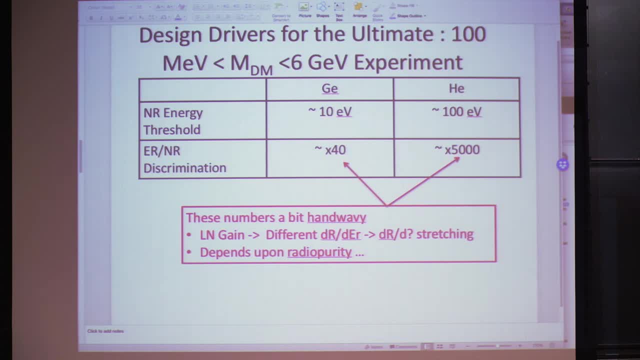 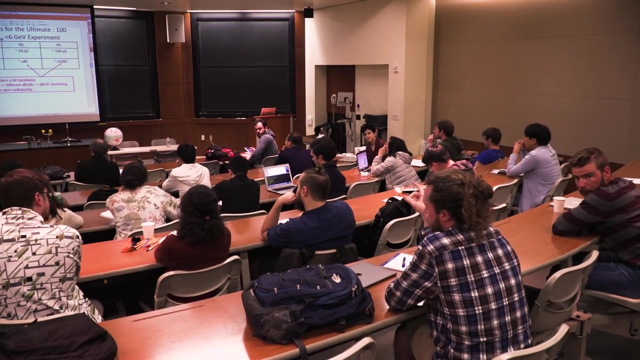 But you're going to need a lot more nuclear recoil, electron recoil discrimination. This is hand-wavy for reasons we'll talk about in the next lecture. So this is basically taking a lux-style detector and just switching xenon for helium. Yes, 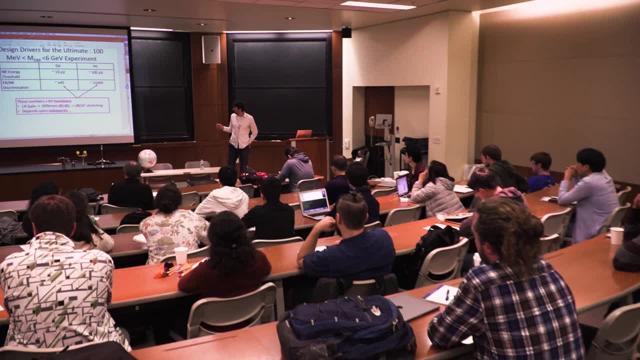 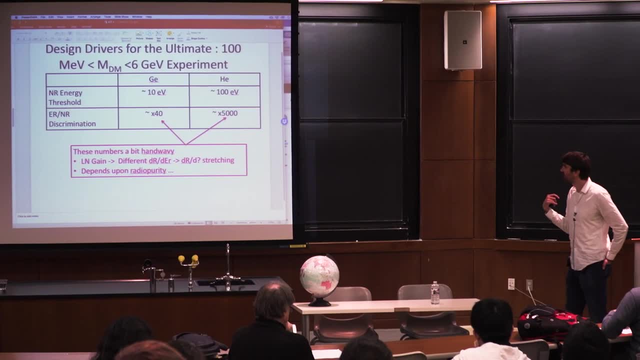 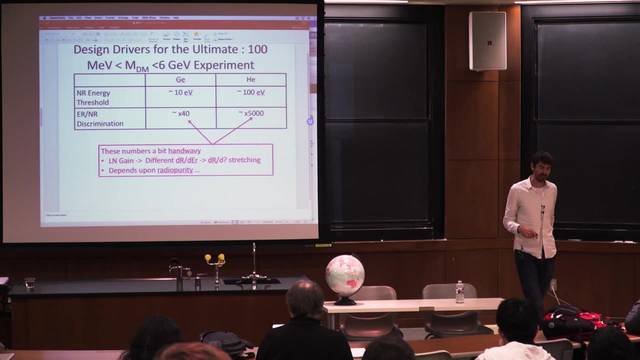 So the question is how one would do that. We're going to actually talk about exactly what this detector would look like in a little bit, in the next talk. There's a few different theories. The first one is exactly what you just said, which is: 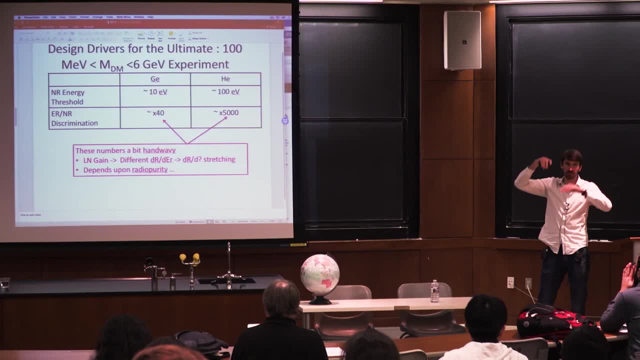 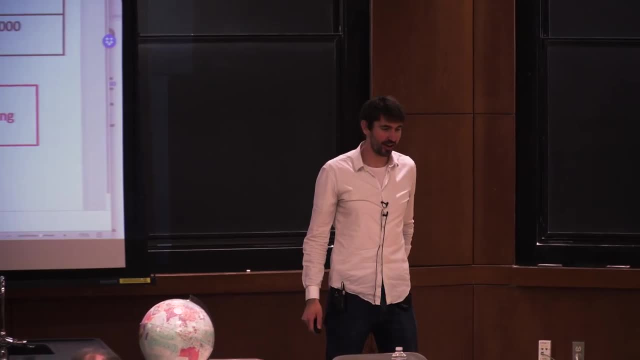 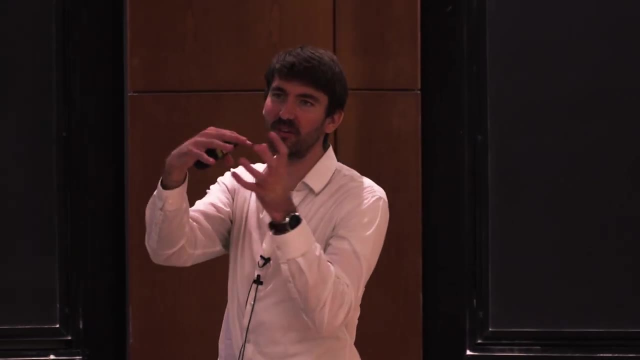 let's take lux, swap it out for helium and put a huge E field across. Turns out that's actually really challenging to do, And the reason why is because electrons have very poor mobility in helium. They basically glob on to a bunch of other heliums. 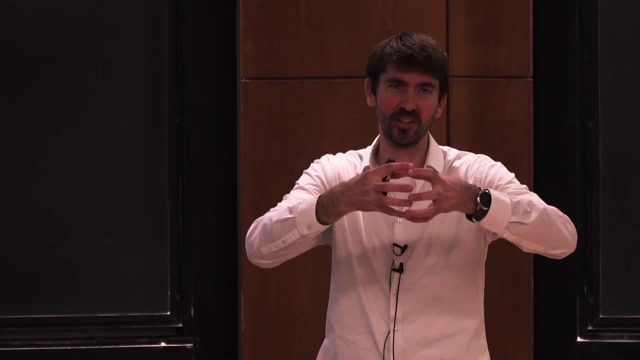 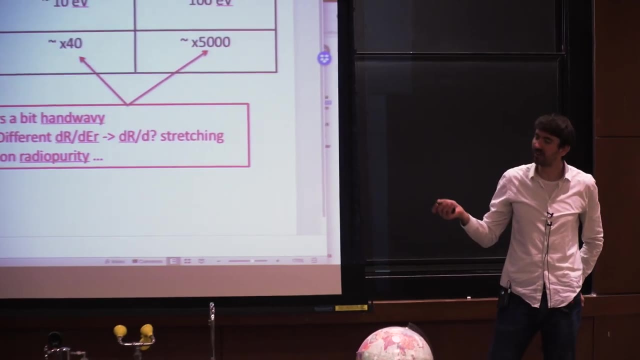 So it's not an electron that flies across. It's like an electron with a bunch of helium going with it across. So it's very challenging to do electron transport in helium. But there are other techniques which are going to be basically using rotons. 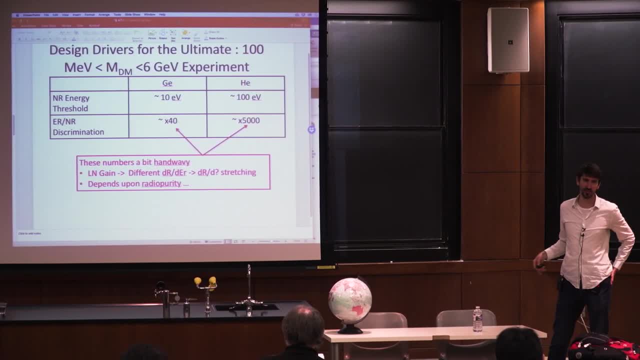 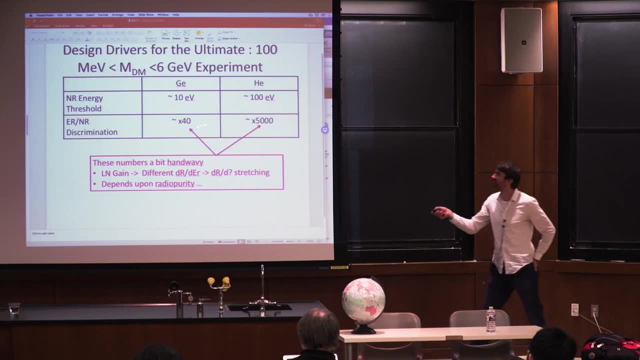 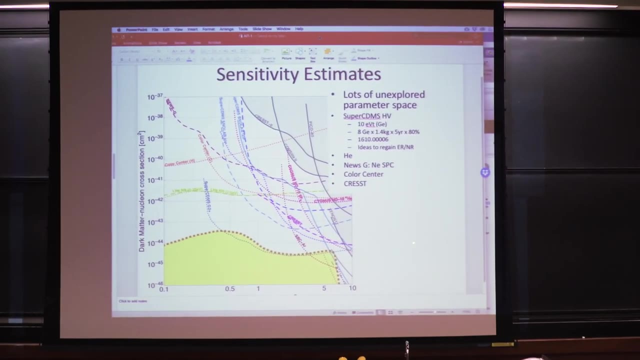 And it'll look somewhat more like supersedium-s is basically, but just with a liquid helium rather than a crystal. But that's roughly the scale And this is what you need in those two. So here are some sensitivity estimates in this range. 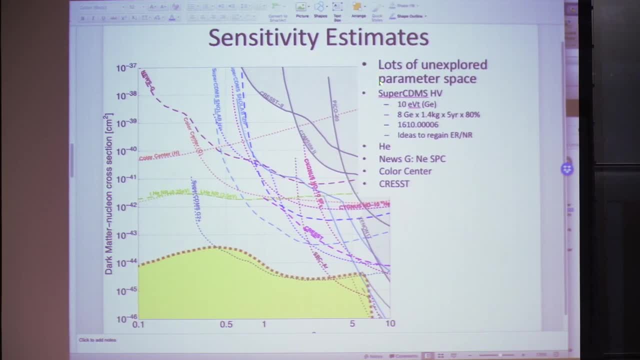 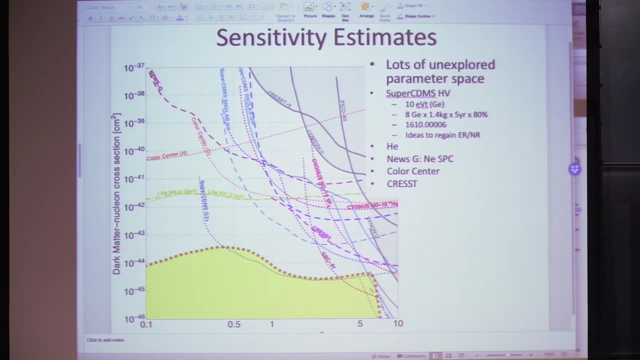 You can see there's a lot of them. So one of the things is I just gave you the ultimate experiment which needs to have this electron recoil and nuclear recoil discrimination. If you don't have the ultimate, you can say, oh, I can still. 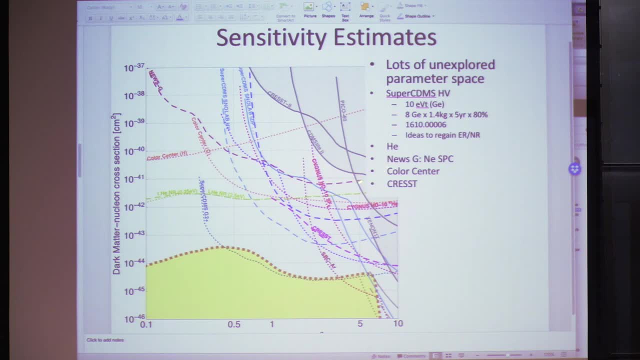 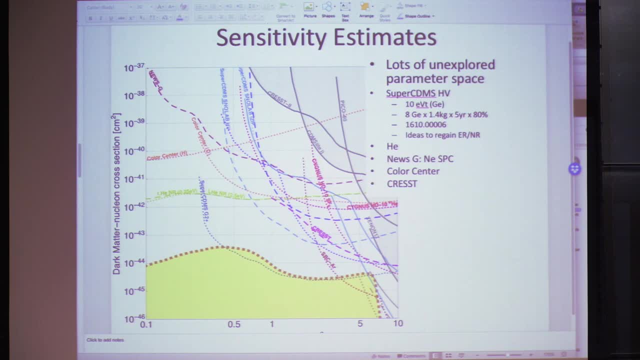 And you're looking for ionization of neon. So it's only a single signal, just the ionization, And they believe that they can do many orders of magnitude better than current experiments. CREST- here is a calorimeter that we'll talk about in depth. 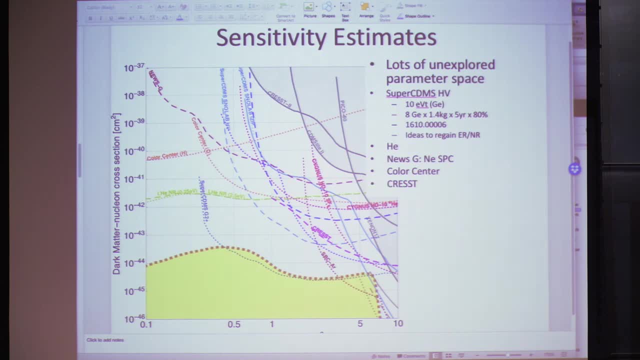 in the next lecture. SuperCDMS is my experiment And it is funded, And it is these lines right here for our first generation which does not have ERNR discrimination. And then we have two other ideas which we will talk about in the next lecture as well: liquid helium and color centers. 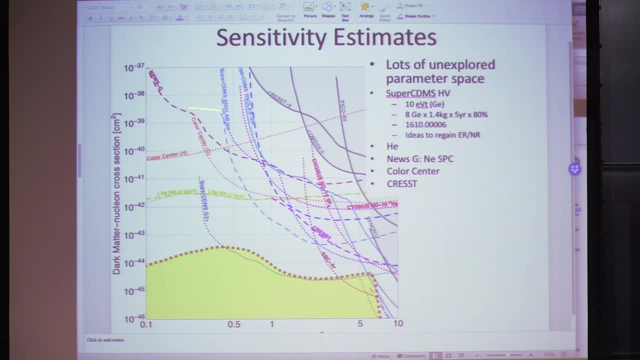 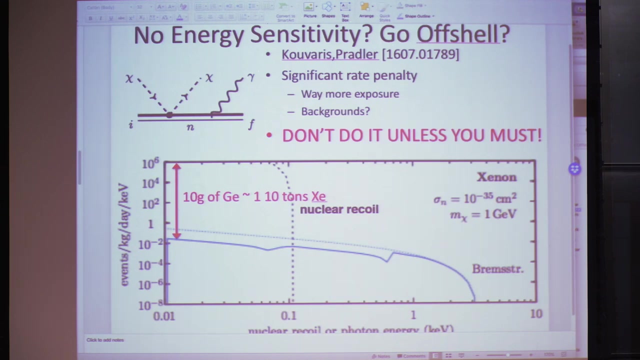 So that's this range. Right now, none of them are really proposing an ultimate experiment that will hit this neutrino 4.. But we should all be thinking about that for subsequent generations. So I want to talk a little bit about this idea. 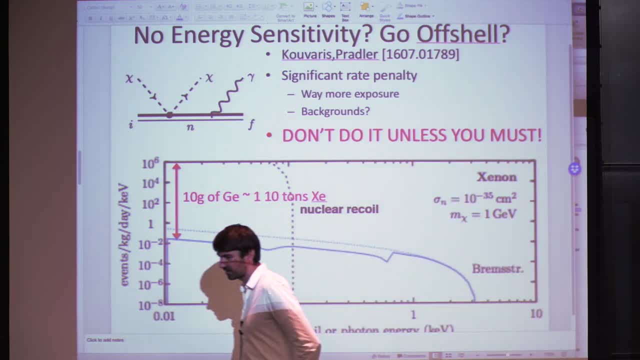 But so far all the design drivers were based upon this idea of elastic nuclear recoil scatters. And the question is: why hold yourself just to simple elastic nuclear recoils? Why not go off shell? Why not make the interaction more complex? So here's a paper that actually talks about this. 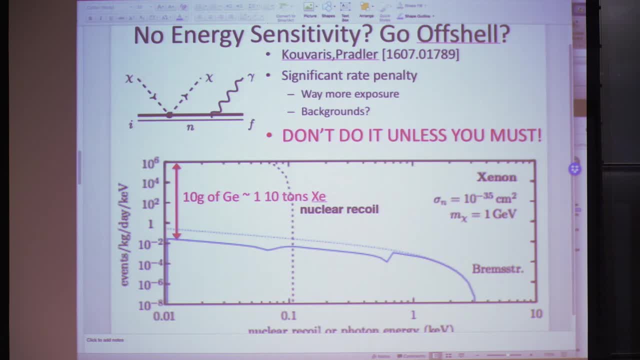 The idea is: dark matter comes in, It hits the nucleus, The nucleus goes off. But rather than the nucleus going off and immediately being on shell and conserving energy momentum, here you instead don't conserve energy momentum, You pay a rate penalty. 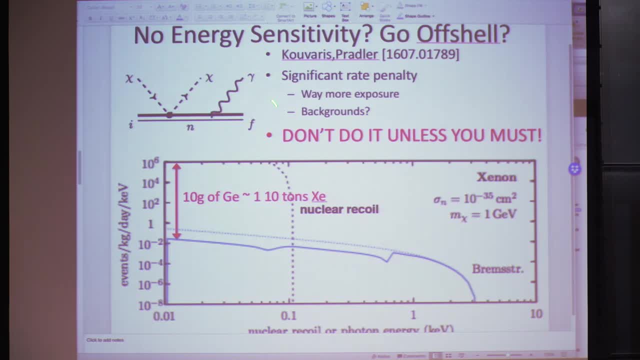 And you throw off a photon And then you conserve momentum here in the entire system. So now it's sort of a three-body process, right? You have a wimp coming in, a nucleus coming in And then coming out is the wimp, the nucleus and a photon. 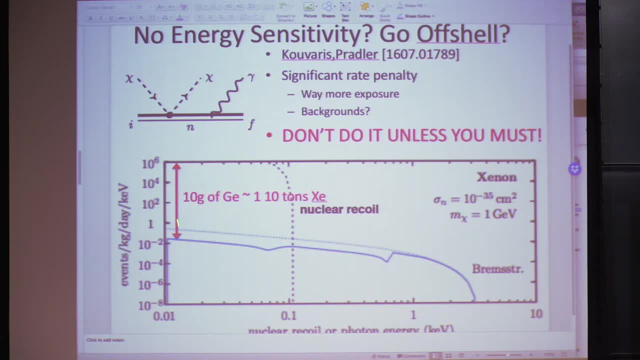 So the problem is you pay a rate penalty, And here actually is that rate penalty. It's something like integrated over the system. It's something like 10 to the minus 6.. So this works if you have a giant 10 ton of xenon laying. 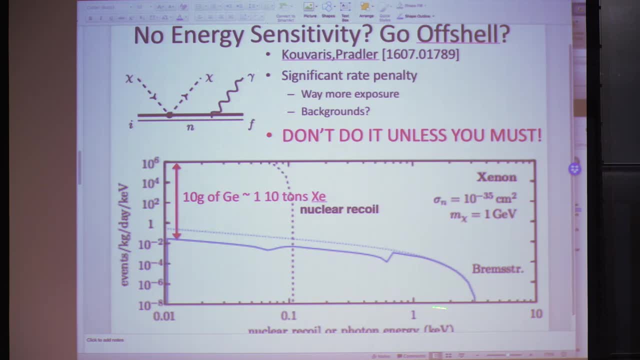 around. You would totally look for the signal because it allows you to extend your search down to something like 100 MeV. But on the other hand, this 10 to the minus 6 penalty is vast right. It means that 10 grams of germanium is 10 tons of xenon. 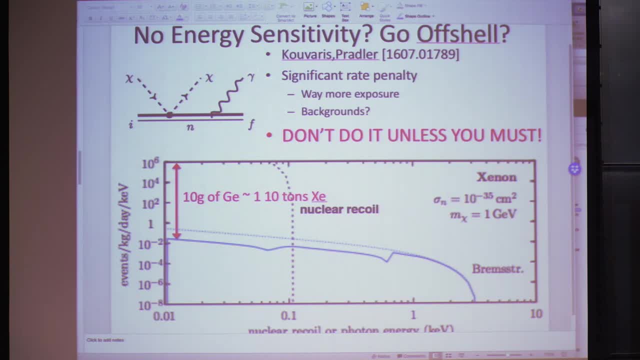 And 10 tons of xenon is an experiment that requires an enormous number of people and $100 million, And a single 10 gram crystal with huge sensitivity could be done in the lab by one group. So we really should think about this idea of the rate penalty. 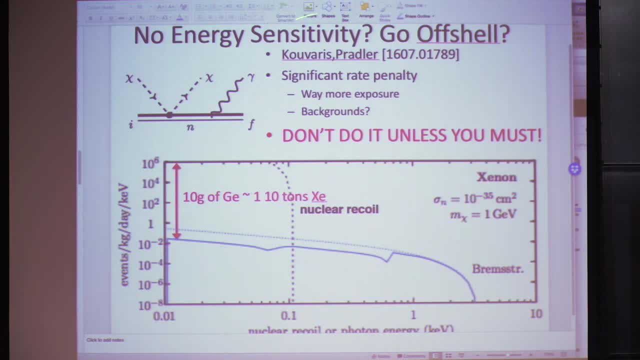 And I guess I would argue that you shouldn't do it unless you must. So if you have that laying around, you should go down that path and you should of course look at it to see if you can see it. But on the other hand, 10 to the minus 6 is a big rate penalty to pay. 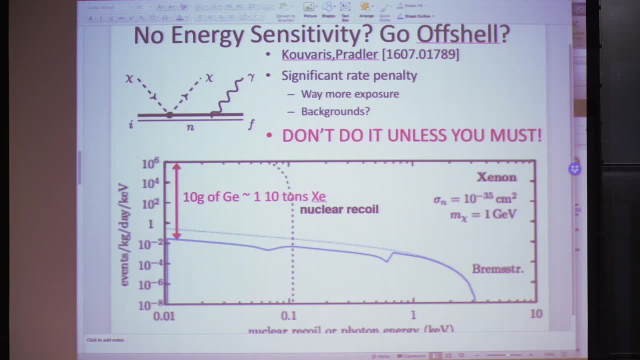 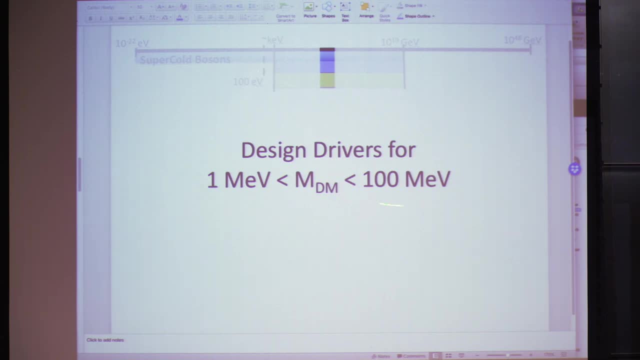 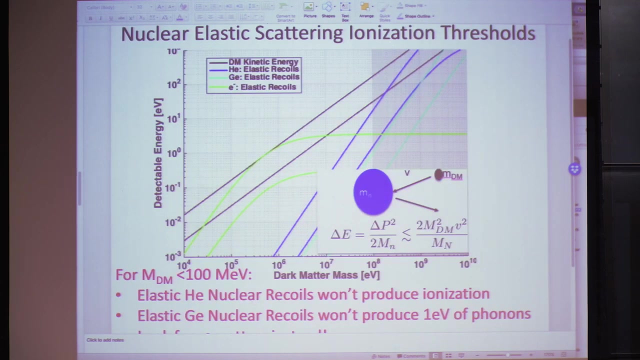 So we should be careful and not go off shell unless we have to. OK, so now we're going to go down further And we're going to go from 100 MeV to 1 MeV, So OK. So so far here. let's see what we have here. 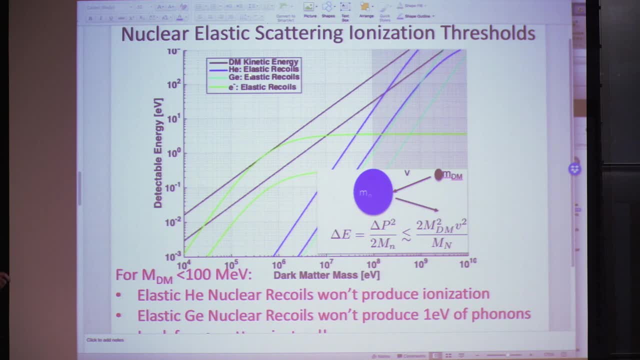 So these are some in cyan and blue. these are little bands here of basically the recoil energies for elastic recoil scatters, for helium and cyan, And what I've done is I've used V escape for our galaxy and V average for some dark matter. 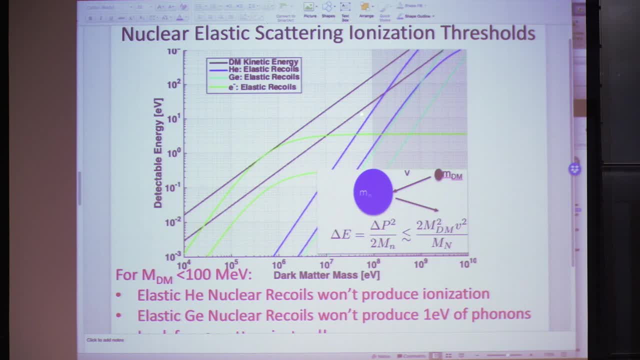 halo. So that's what So V escape would be the highest velocity we would expect, And this would be something like the average, just to set the scale of what kind of recoil energies we could see. And we see this: M squared, dependence 1 over M squared. 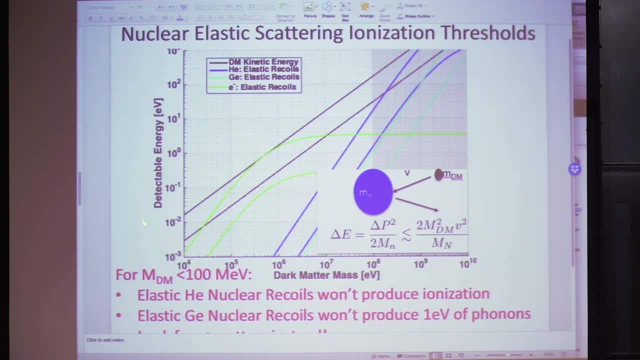 So as we go down in dark matter mass the recoil energy for elastic nuclear recoil scatters goes as 1 over M squared. By contrast, the kinetic energy in the detector in the dark matter particle just goes as 1 over M. So it's much less sharp. 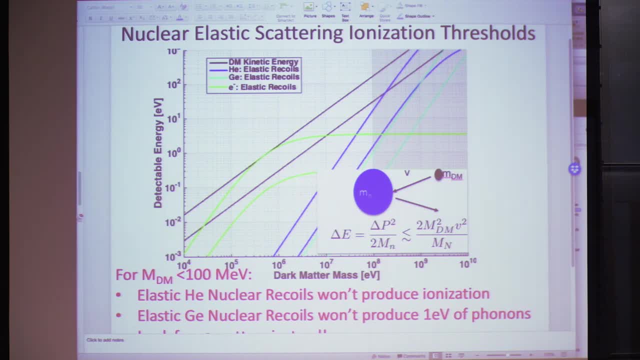 So what we can see in this range, so something like: so where does it get difficult for us to see any kind of like, let's say, an ionization signal on helium, well, or neon that sets basically at 100 MeV? 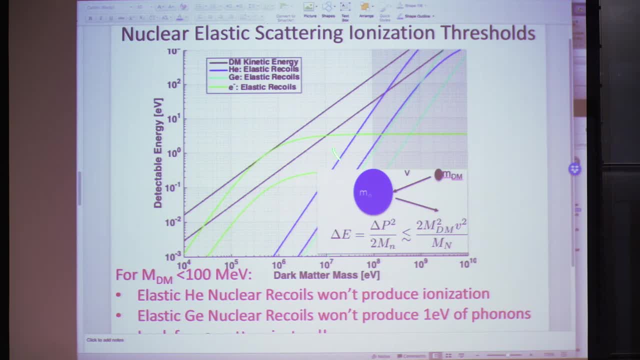 So the best detector you can get is a 100 MeV. OK, So the best detectors you could think of are going to have problems with ionization at something like the 100 MeV scale And, if you want to look at, like nuclear recoils in terms of heat, as in germanium. 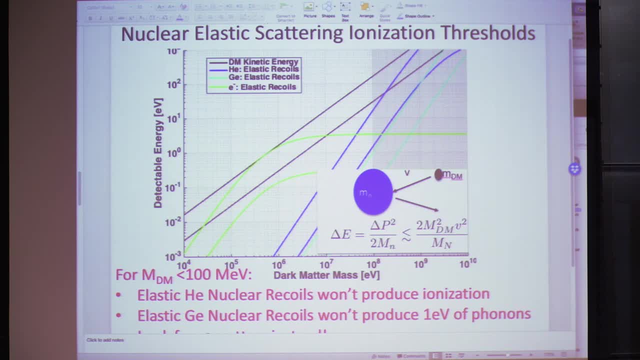 you know that's going to be something like 1 MeV of energy. So you're going to go below 1 MeV of energy. if you want to search for those signatures, And so you know the moral is, maybe there's something else we can do. 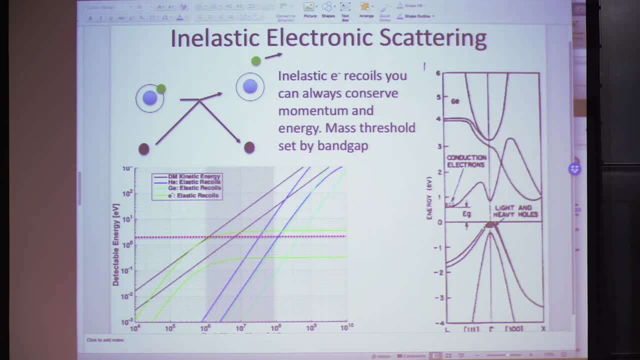 And So the idea that was tossed out there by Reuven- and I think I have the citation down here, unfortunately, which you can't see- but by Tomor Wolanski and Reuven Essig and their groups, was: let's actually look for inelastic electron scatters. 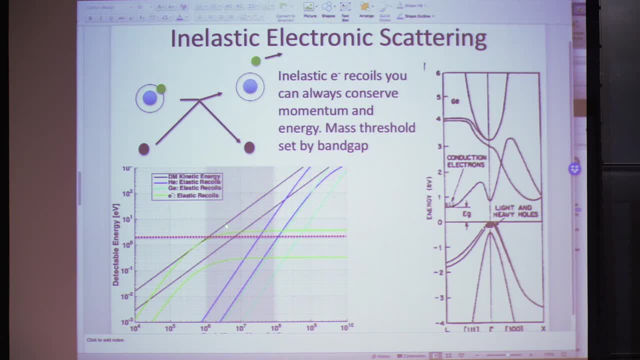 So an electron is just better band-matched in this area, right? If you're looking for 1 MeV dark matter, an electron is a natural thing to look because it basically has 1 MeV of rest mass energy. So it's going to be close. 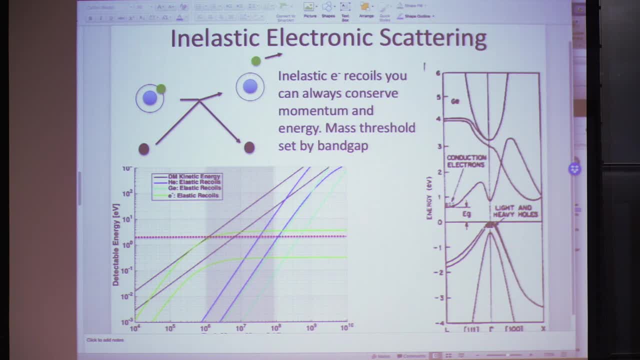 It's kinematically matched very well. So that's a check, But actually it's even better, right? So it turns out that if I think of like all my electrons are going to be like in a nucleus, a dark matter product comes in, bangs up against a nucleus, it kicks out an. 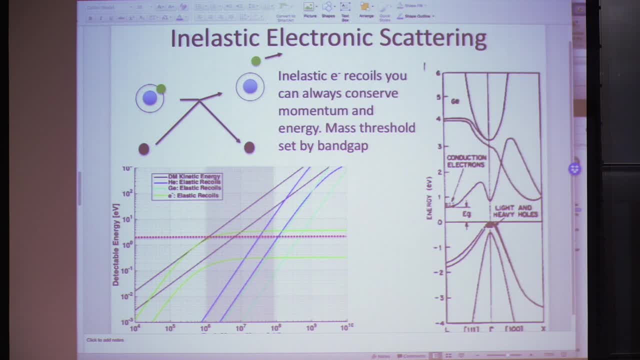 electron, So we can always conserve energy, momentum, Because, yeah, this is, And we can think of it in a few ways, But really the best is the Yeah, Yeah, The kinetic energy and momentum- it's The full momentum- can be conserved. 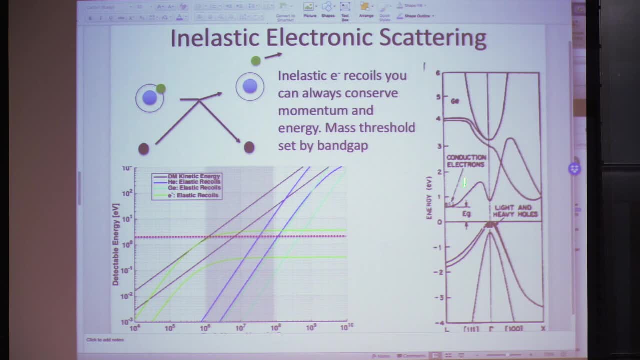 So here is a case where we see that. So here this is actually a band diagram for germanium. So what we can do is we can actually just take a bunch of particles here and we bring dark matter in, hit scatter off of it. 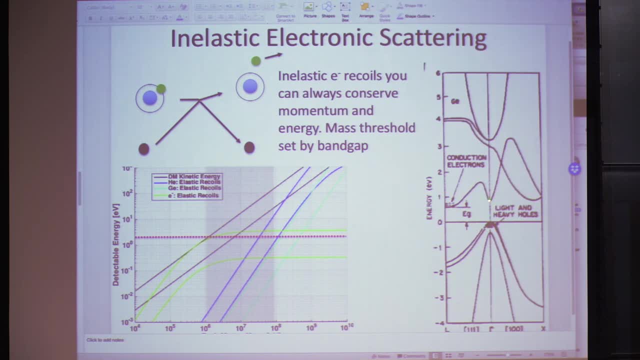 It kicks an electron from the valence band up into the conduction band And we can conserve for momentum. We can conserve k and energy in that process. So the threshold of this process is going to be set by the band gap. So if we use, germanium has a band gap of something like 1 eV, then we could go down. 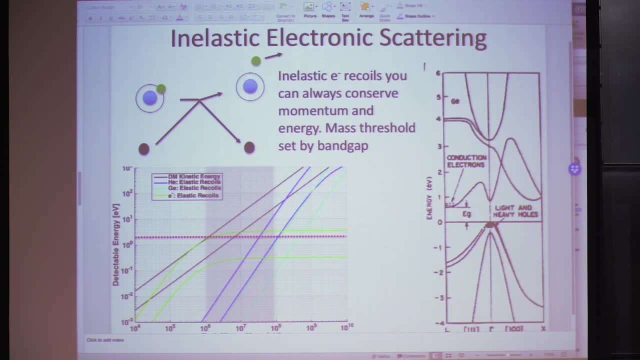 to something like 1 m eV. So we exactly see what sets this range over which we can look for inelastic electron scattering, And that's germanium. That's just this range below nuclear recoils And something like 1 eV for ionization, which is the lowest semiconductor we see. 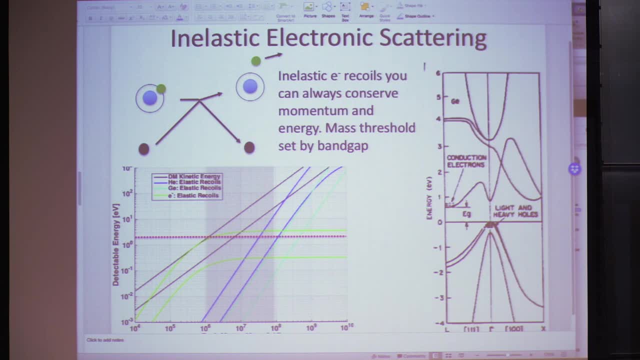 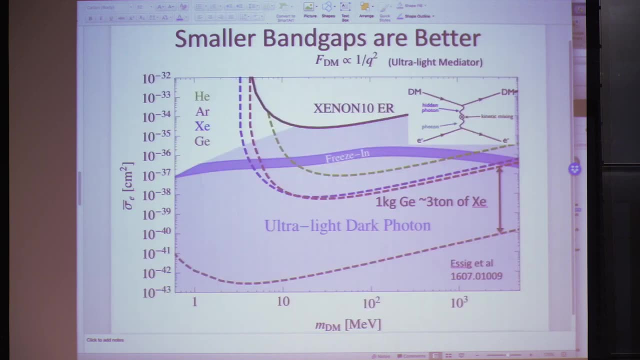 Of course, if we're using xenon, there, the band gap is bigger, And so we're going to necessarily have a higher threshold. So let's actually see that here in this plot by Ruben and Tomer. Yeah, Yeah, Yeah. 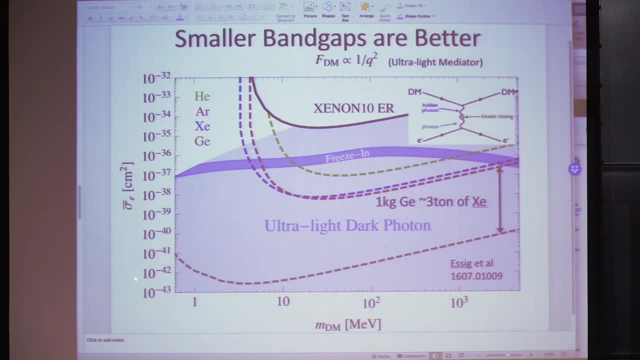 In which we can actually see a few things. So here is that threshold idea. So this is again experimental cross section. All of these are for one kilogram year of material, And this here is the germanium line Here. this is xenon, argon and helium. 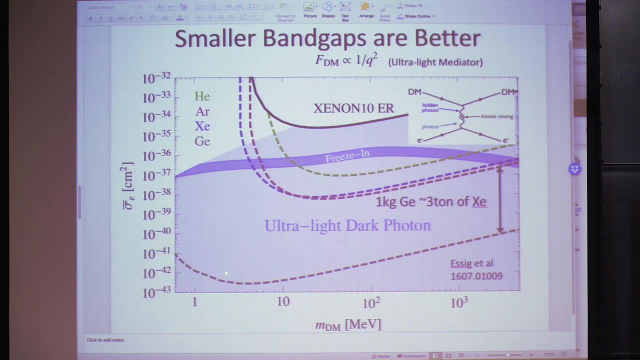 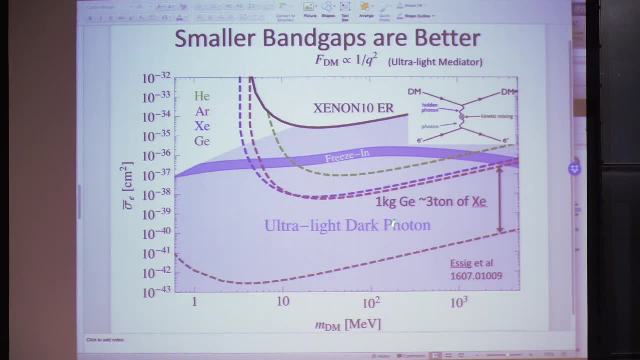 Yeah, Yeah, Yeah, Yeah, Yeah, Yeah. So you get huge improvements in this range, But you also get a change here. So the lower the band gap by far, the bigger the scattering rate, And it's something like 10 to the, I guess, 3,000.. 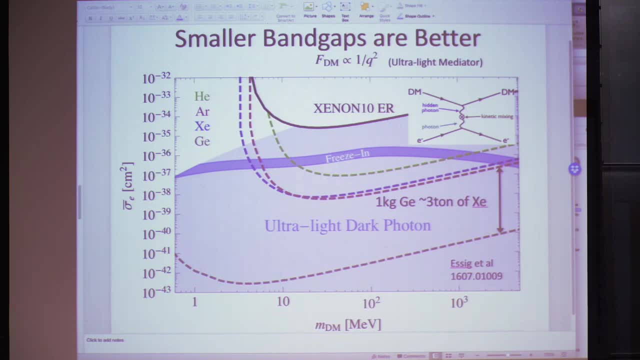 So something like a factor of 3,000 between germanium and xenon. So what does that tell you? Again, it just sets the scale of these right. So one kilogram of germanium is worth 3.3.. It's worth 3 tons of xenon. due to this fact, 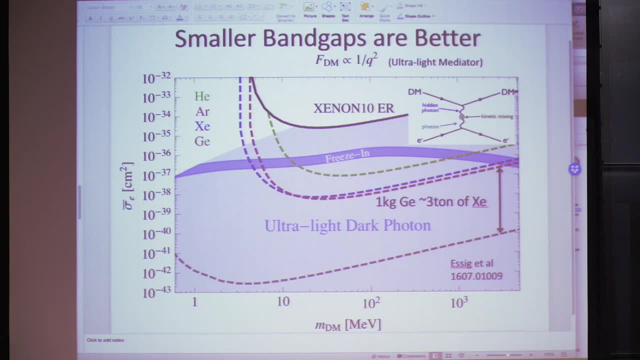 And if you're an experimentalist and you're saying, which way do I want to go? well, it's a lot easier to instrument one kilogram of germanium. So that's one of these things of this design grant. So one of the design drivers we're going to think about in this range is: we want to have 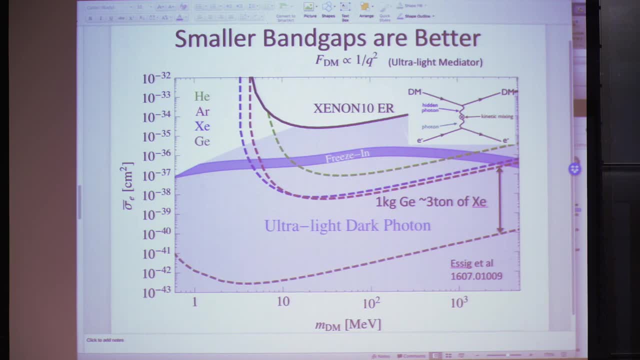 very small band gaps. So here actually is the one experiment that's so far been done, And it's actually by experiment, By a xenon experiment, where they looked for single electron, two electron, three electron peaks, And we'll talk about this in depth as to why they got stuck here and why they couldn't. 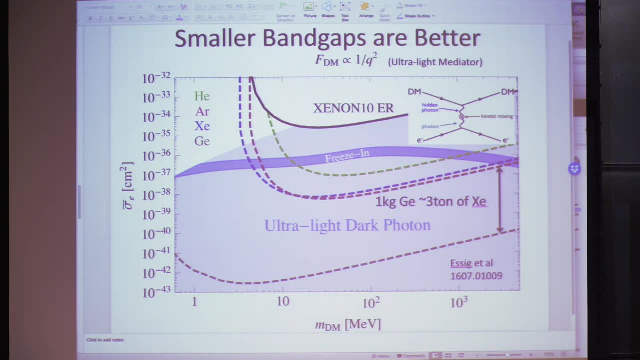 go much further down, Because you know this is 10 kilograms of xenon. Why weren't they able to get into this range? Because this is just one kilogram here, right there. So they were, you know, over three orders of magnitude off the expected sensitivity. 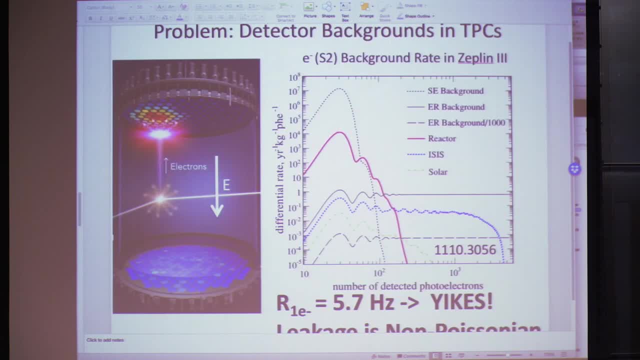 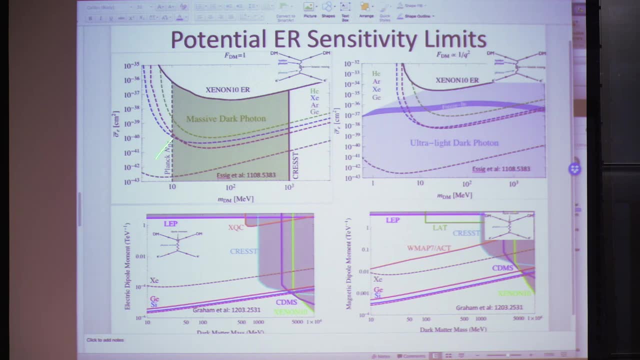 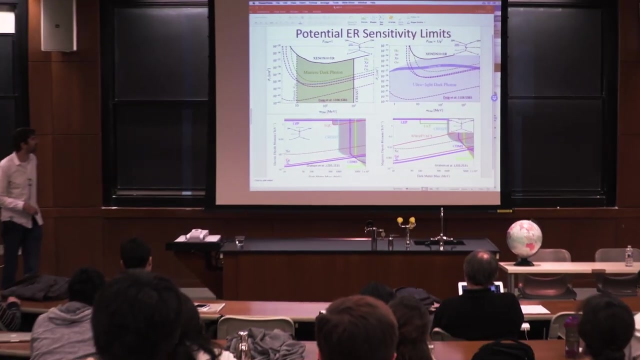 of this device. looking at this plot. OK, So here are a bunch of different models. In every one of these models, in terms of sensitivity estimates, you see this same concept. You see that basically, for So in the previous slide, when you were using the band gap of germanium, what is the natural? 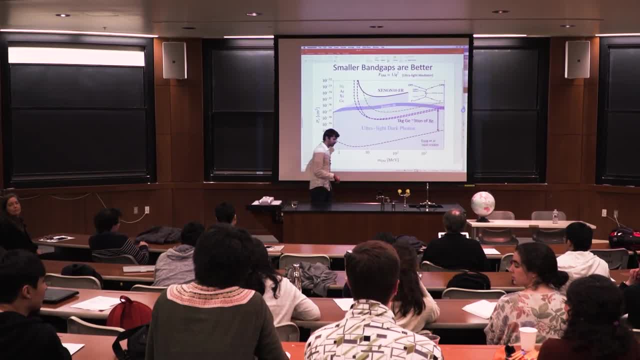 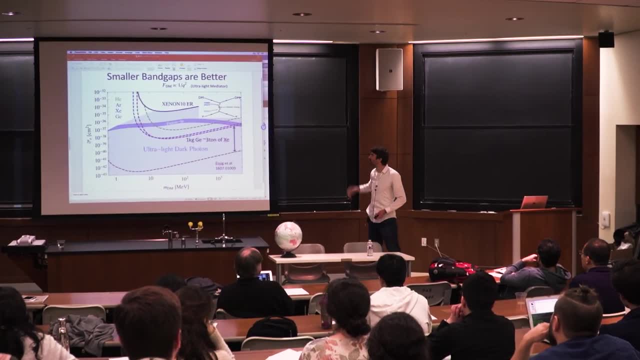 background? Is that the thermal excitation of the electrons above, for example? Yeah, Yeah, Yeah, Yeah, No. So we'll actually talk about these detector backgrounds. Oh, yes Again, Yeah, Yeah, Yeah. So the question was: what are the backgrounds for these signatures? 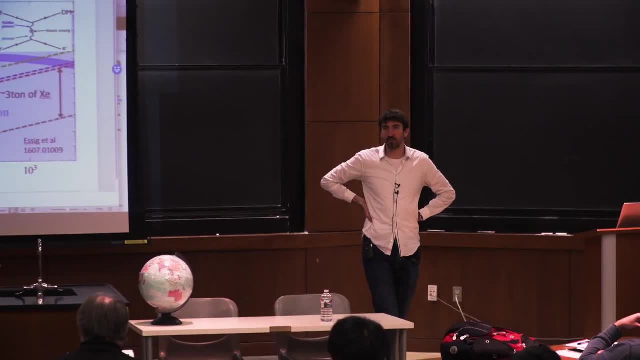 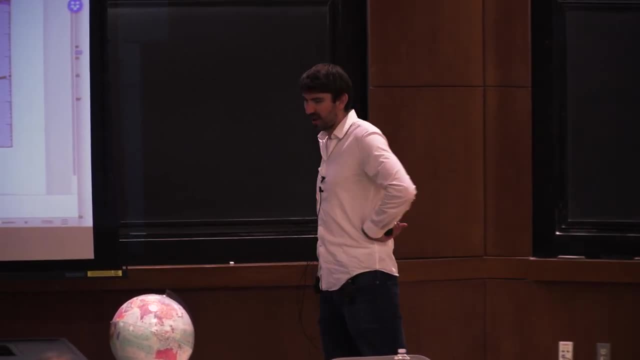 So we just talked about the fact that the radiogenic backgrounds weren't that big of a deal. right, As we go lower in mass, the radiogenic backgrounds are just not as big of a problem, And that's because the radiogenic backgrounds scale. you know, Comptons are basically uniform. 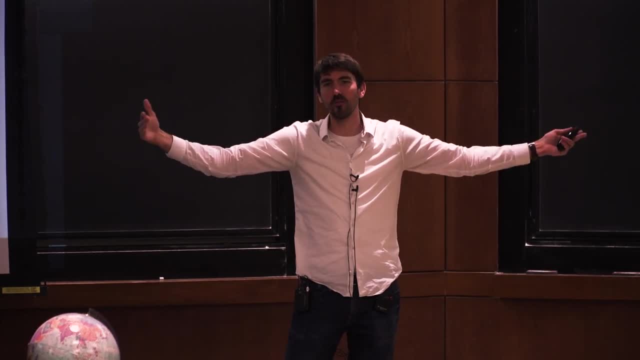 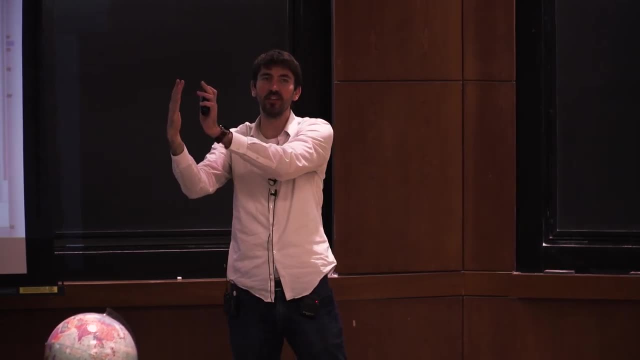 from 0 to 200 kV. So the overlap of that, So the overlap of that with your signal, is big when you're looking at signals that are 10 kV. But when your signal is just in eV, 10 eV, then the overlap with that big Compton spectrum. 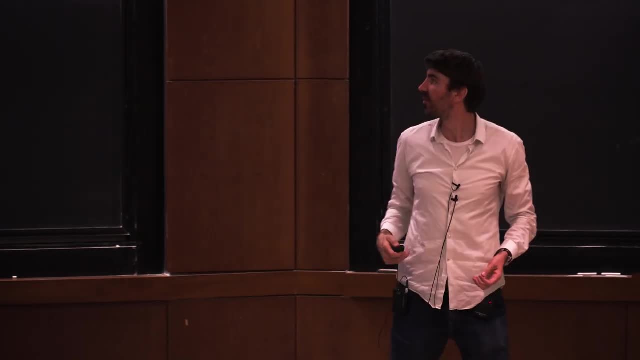 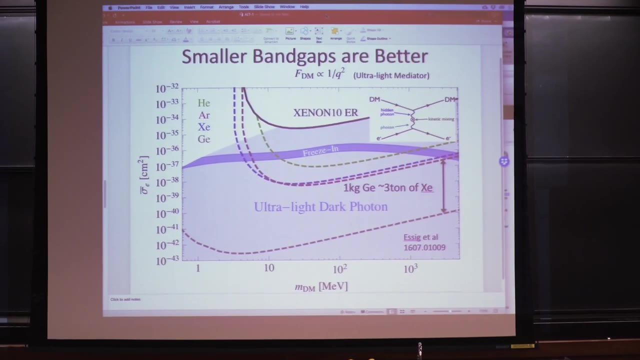 is very tiny, So you're just not seeing the overlap. So the actual background in these experiments is going to be detector physics, It's going to be dark counts. So we'll see that in two slides. Okay, So a bunch of models. 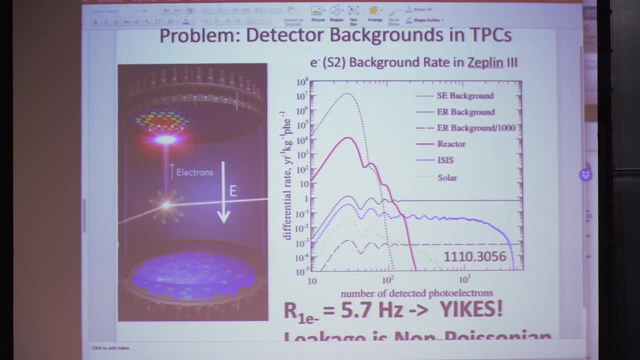 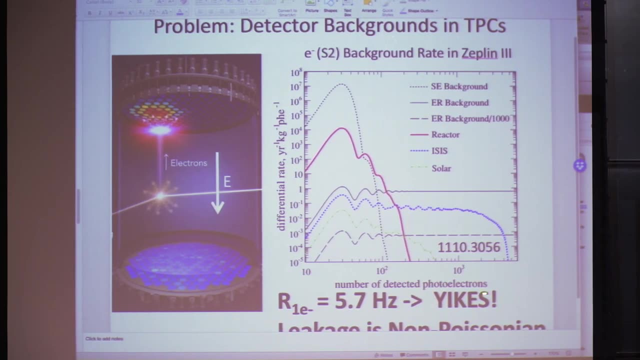 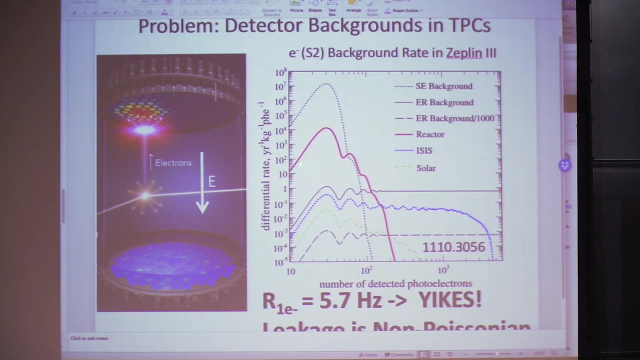 And here is the slide Let's talk about. So here is actually basically that detector, So this is a xenon TPC And here is a plot of Zeppelin III. So it was one of the xenon TPCs And this is the rate of single electrons that are being read out by the experiment. 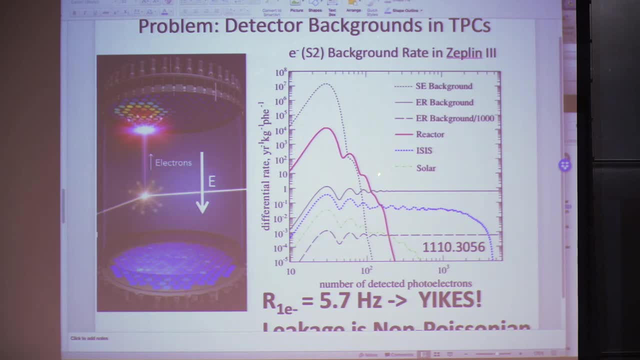 So they had single electron sensitivity. Here's one electron, Here's two electron, Here's three electrons. And this is their rate of single electrons: It was 5.7 Hertz. So they had a huge background of single electron events. 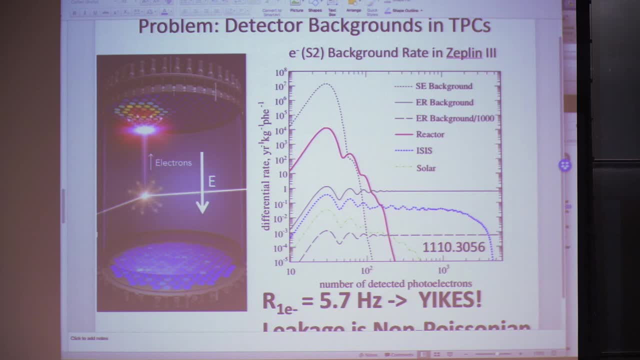 That's going to make it really challenging to see a dark matter signal, And this is not fundamental. This isn't particles banging your detector. This is something happening intrinsically in the detector, So let's actually ask what it is we believe is happening here. 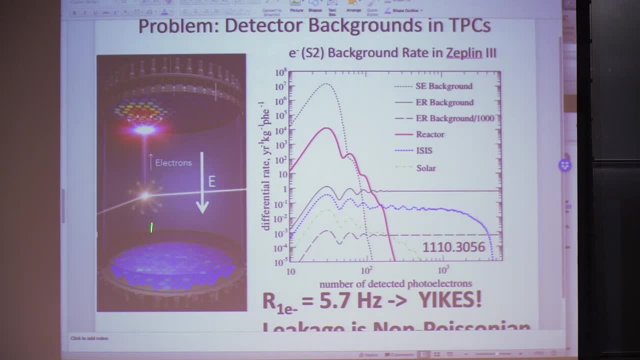 So a few things could happen. Remember, we have this very high eField in this TPC, right, So we're charged at something. It's something like a kilovolt per centimeter. eFields are what we're putting on here, So maybe we just have tunneling of an electron off of the metal grid. 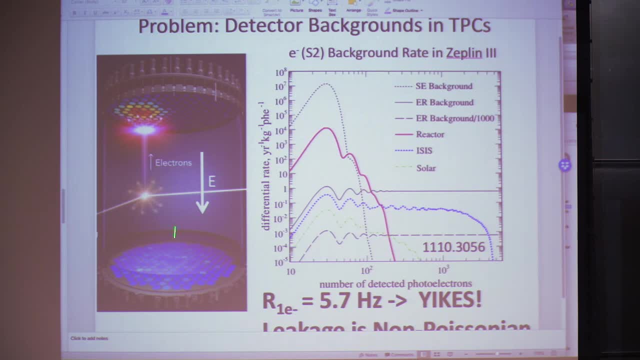 So we have a huge eField. An electron can tunnel off the electron grid and fly across. So that's one possibility. Another possibility is that we had this interface between xenon gas and xenon liquid And maybe electrons are getting stuck at that interface. 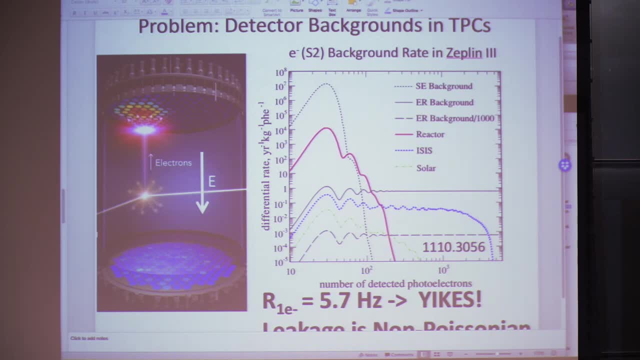 And they're just sitting there- And we know actually some of them are- because they believe that something like only two-thirds of the electrons are actually getting across into the gas. So one-third of your electrons are getting stuck right at that interface And maybe those electrons then also tunnel out and then kick up and give you a single. 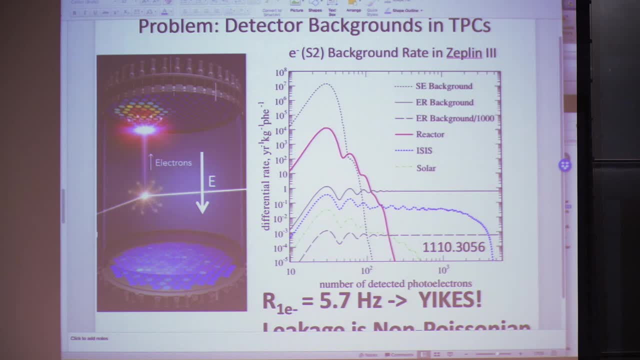 electron signal. So these are all single electron signals which aren't fundamental. They're not particles hitting, They're just your detector, Yourself. You see this fundamental background And this is not just seen in this detector, This is also seen in PMTs, right. 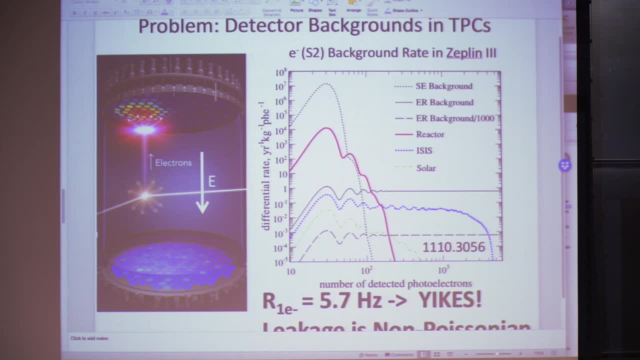 So if you guys have ever used photomultipliers, you know photomultipliers have dark count rates. And again, why does a photomultiplier have a dark count rate? It's a non-equilibrium process, right? You have this huge eField to generate your amplification. 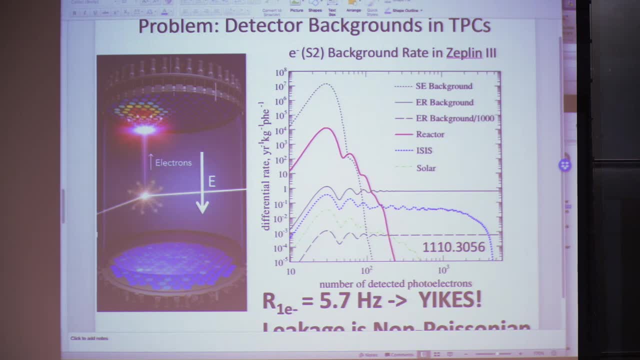 And that huge eField will give you some tunneling, And so this is one of the problems- Is that all of these, All of these experiments that are going to look for single electron and two electron and three electron signals, are going to have to worry about these detector backgrounds. 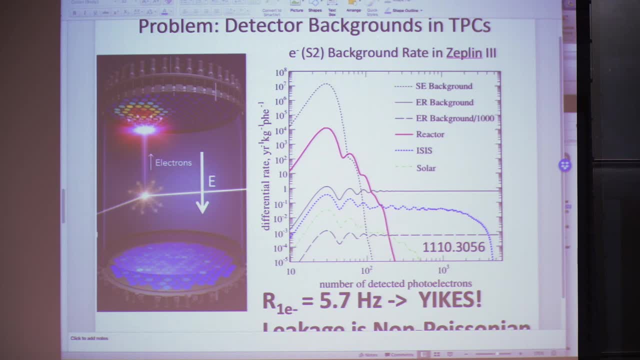 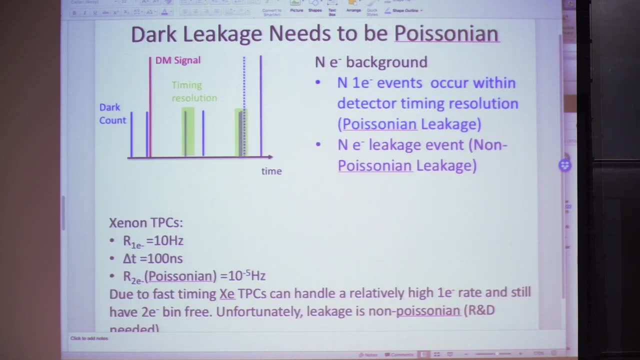 And that is what dominated Xenon 10.. It wasn't radiogenic backgrounds, It was totally detector backgrounds. So I want to talk a little bit more about that, in which- well, in both of those two scenarios I just gave you right, 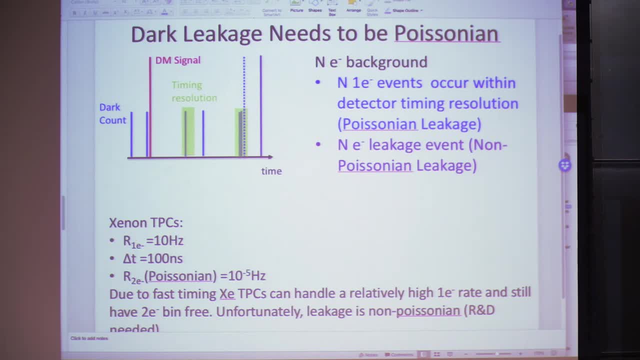 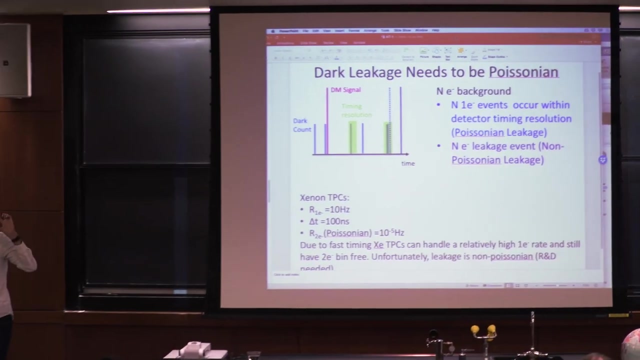 You had. You had a single electron tunneled out of the metal surface. You had a single electron tunneling off of the gas electron interface. So you're like: ah, that's going to hurt my single electron band, But my two electron hole region of interest, my signal, that should still be okay. 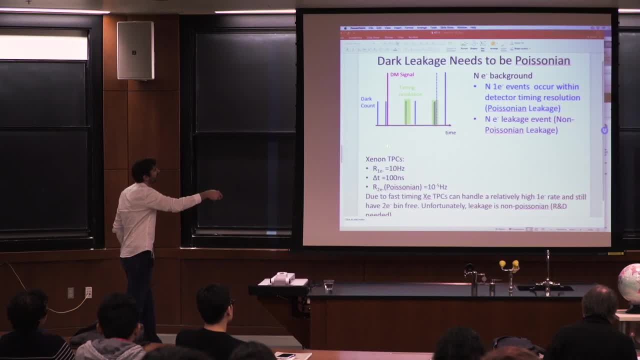 So if the dark matter particle comes in and gives me two electron event, Gives me an event that produces two electrons, I should be able to distinguish that from all the dark counts. So maybe the dark count rate will only kill my one electron bin but not my two. 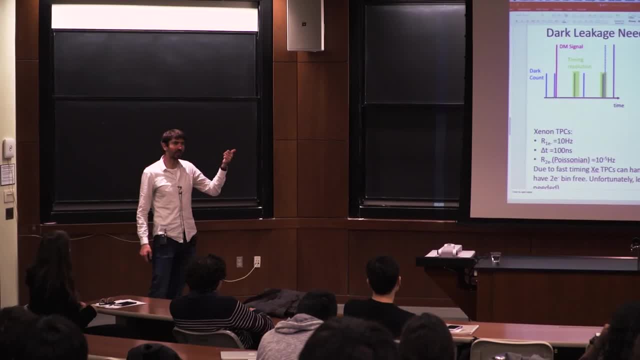 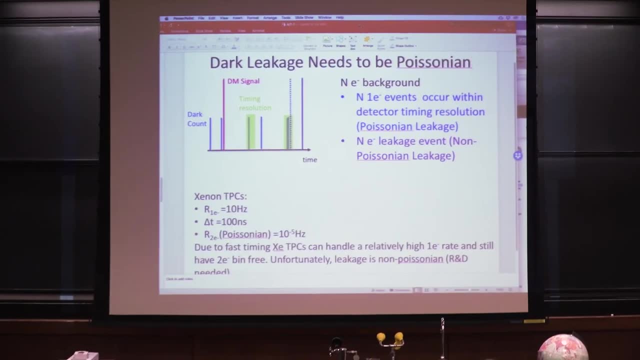 No, because you said the frequency is crazy. right, Well, but at 5.7 hertz. let's actually just go through the math. I have the math right here, So let's just toss the math down at 10 hertz. 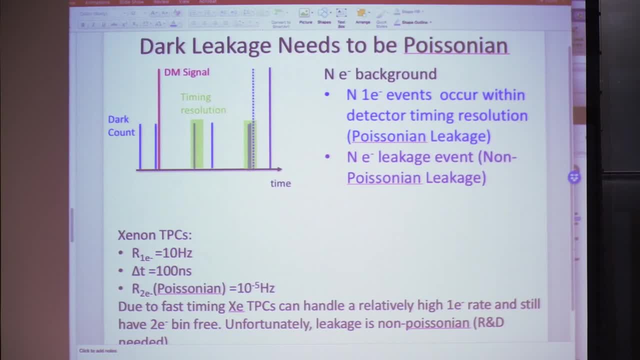 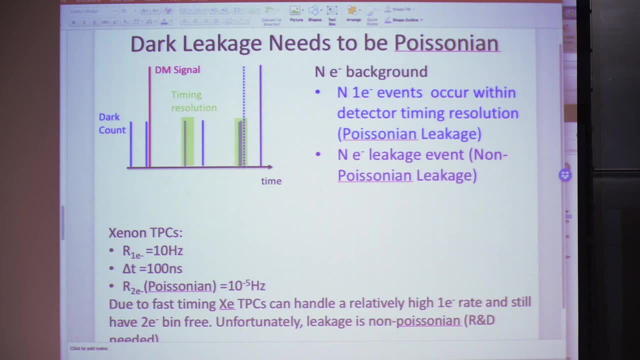 So it turns out that a Xenon TPC- I don't know if you guys know PMTs well, but a PMT- has roughly 100 nanoseconds resolution. Yeah, You can get better PMTs faster. The standard PMTs that all the Xenon TPCs use are something like 100 nanoseconds. 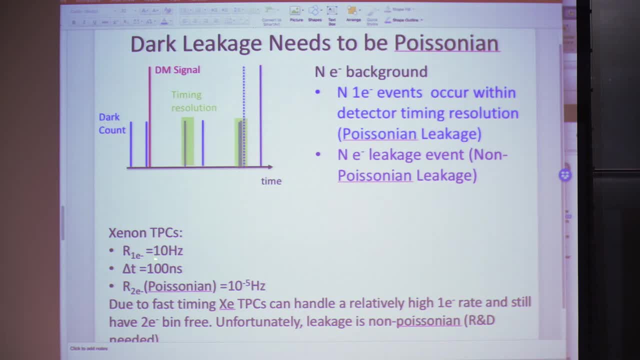 So that means let's just say what are the odds if your rate is 10 hertz? what are the odds that two events are going to actually come within the timing resolution of your detector if it's Poissonian? So by Poissonian I mean that the events are randomly distributed in time. 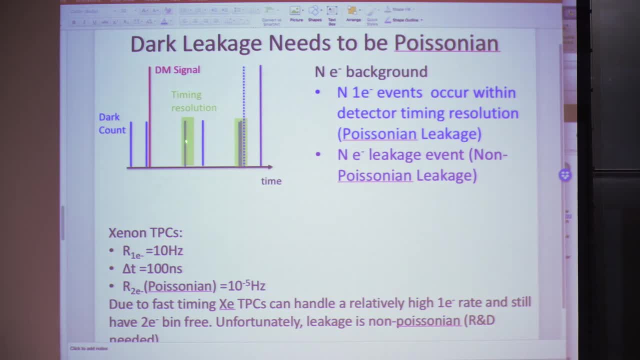 So I have some dark count here, a dark count here, And then Uh, And then finally, here I have two that are within 100 nanoseconds of each other. So what are the odds of that? Well, I can just do that math. 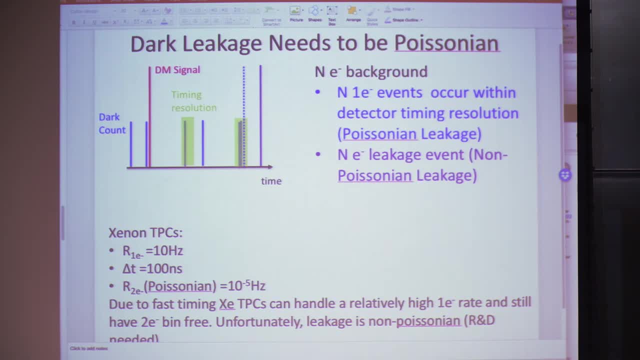 I don't even have to go through the Poissonian statistics. I can say on average, if particles come in every 10 hertz and I have 100 nanoseconds resolution, this is like 0.1 hertz. So a particle comes every 0.1 hertz, 100 nanoseconds, that's one. e to the minus seven, that's one. 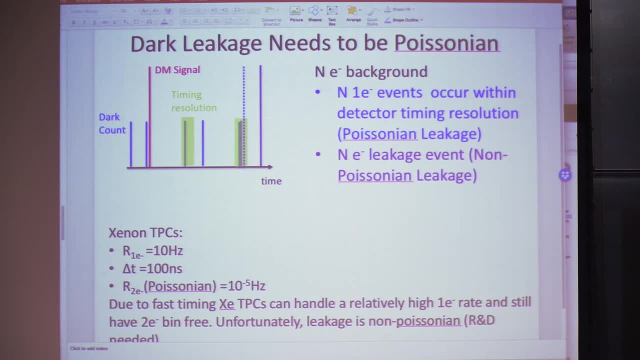 e to the minus six, So one Of every one million leakage currents, I would expect two of them to be so close to zero together that I couldn't distinguish them from one event. And if that was the only background Xenon 10 had, it would be great. 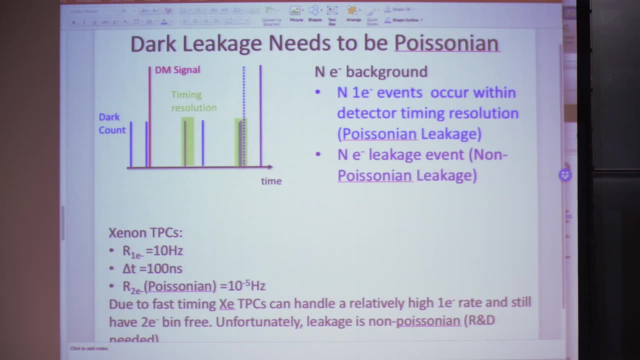 They could say I'm not going to look at the one electron signal, I'm going to look only at the two and three. I'm still going to have a world-leading experiment And they're going to have soon seven tons of material. 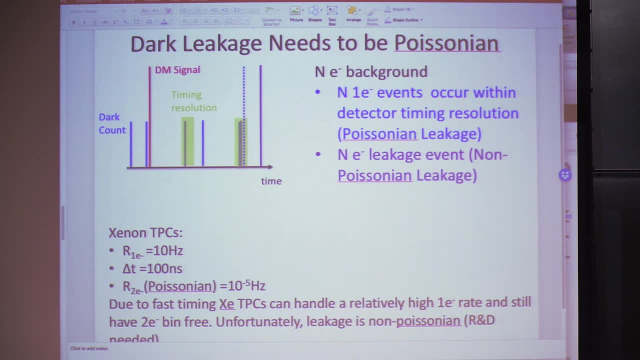 So you can do really, really well just looking at the two-electron thing. Okay, So the problem is is we have a non-Plaustonian leakage. So what they see is they see that the number of two-electron and three-electron events 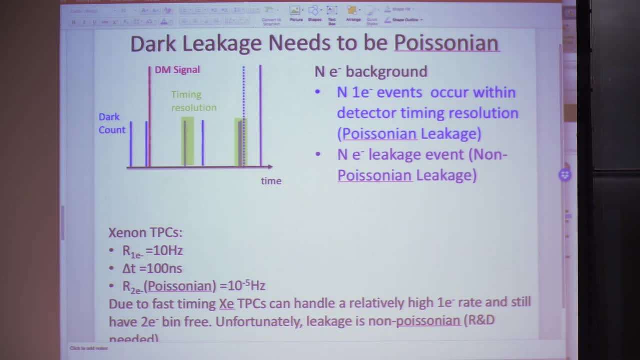 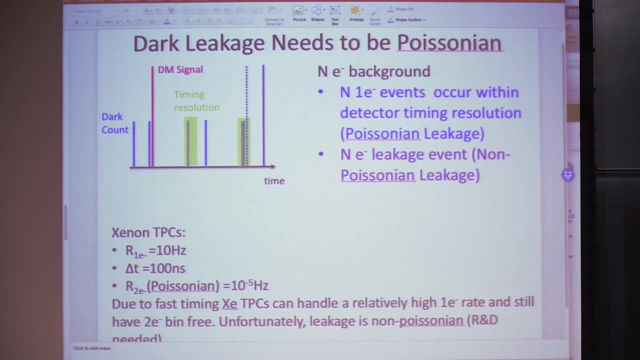 are way bigger than what one would expect from Paustonian leakage, And this is a problem. So let's think about how we could get this, And this is a. There's a bunch of R&D going on at Lawrence Livermore right now for this. 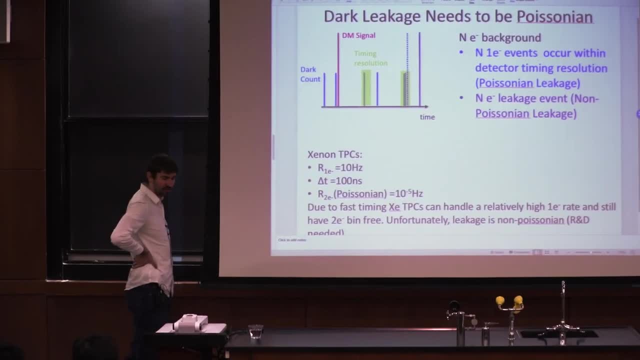 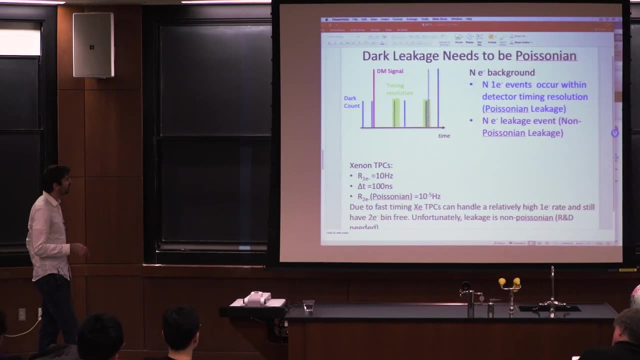 Also, Peter Sorensen at LBL is playing around with this a lot, trying to figure out what's happening and why they're getting these non-Plaustonian leakages. But the basic idea is here. So let's say I have. 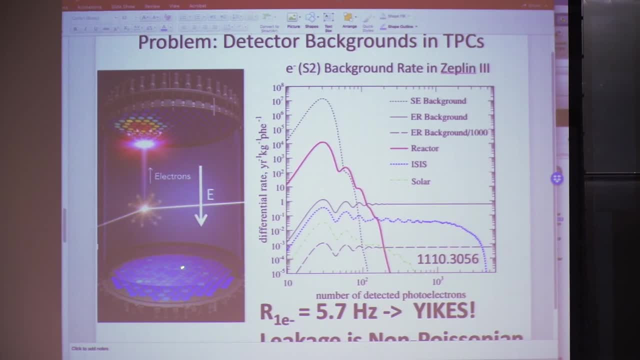 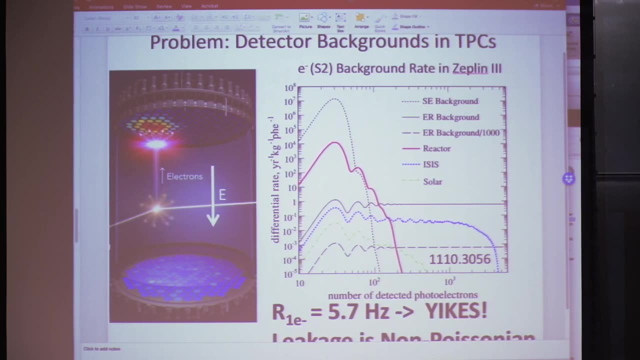 Let's start out with a process where I have a single-electron tunnel out of here, flies across, kicks up here and makes a bunch of UV photons. right, That's how we're reading it out. Some of those UV photons are going to get back into the xenon and then they're going. 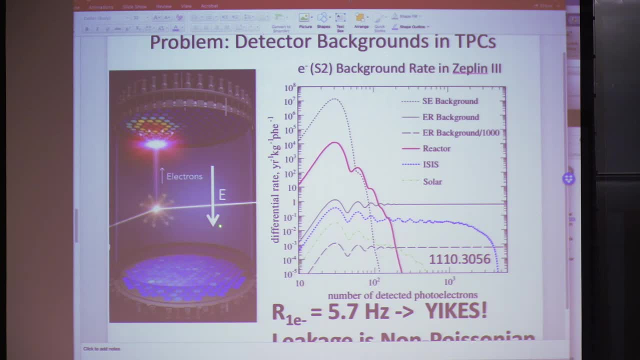 to be able to ionize an impurity. So we have a few impurities. We have an oxygen atom, We have something that's sitting in here. It has an electron sitting on it That UV light ionizes that impurity. That impurity then has an electron that flies across and it gives me another event. 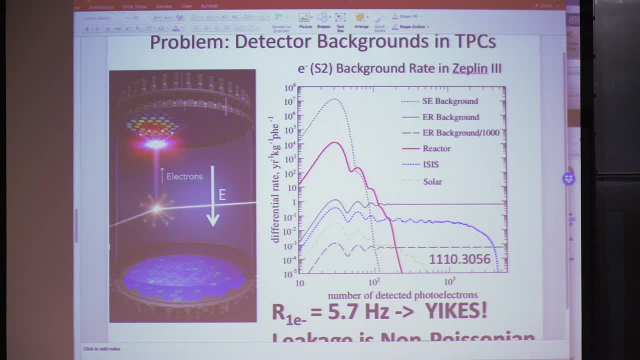 So things like this are ways that you can go non-Plaustonian and you can have a huge number of events. These events start occurring very, very quickly And you can start to get this non-Plaustonian background. 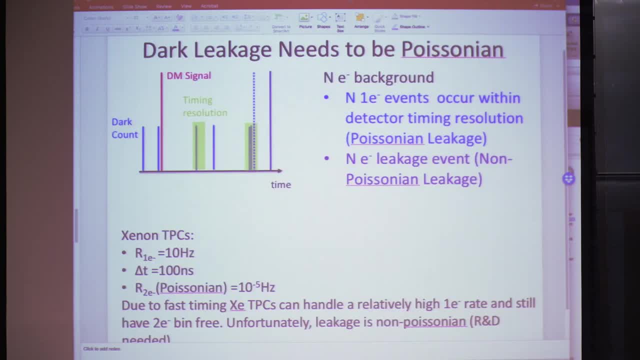 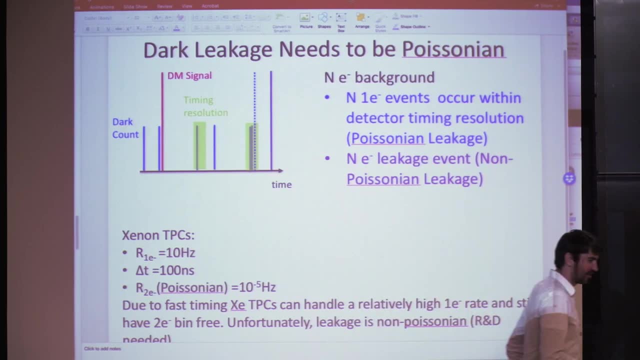 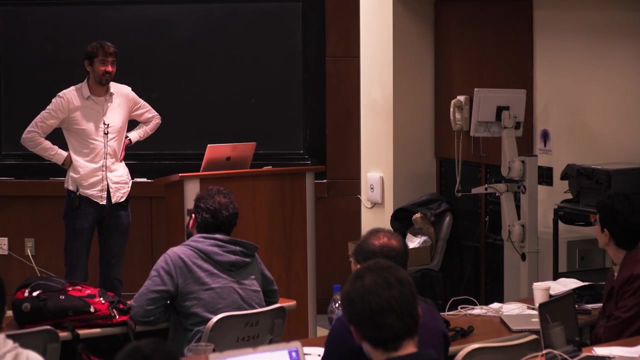 And so you have to somehow stop that chain. So what impurities are you talking about? What kind of impurities do you have in Xenon? You have lots of. I mean you have some oxygen. You have just lots of stuff that's getting in there. 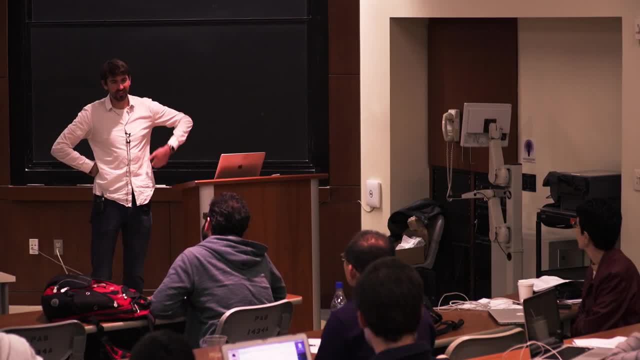 I know oxygen is one of the big ones, But I mean, you know it's hard to keep things out of. you know What's the level? We're talking about very, very small levels. Like I must say, I'm not a Xenon physicist, so I can't actually give you exactly the number. 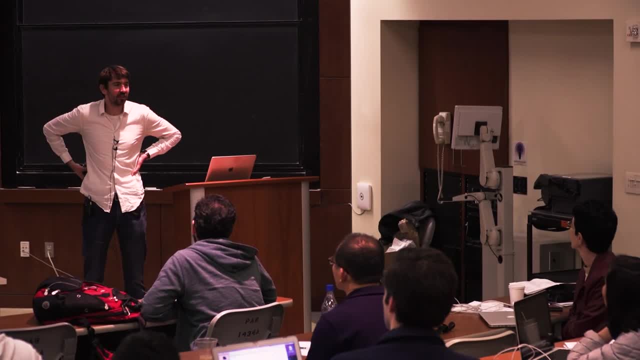 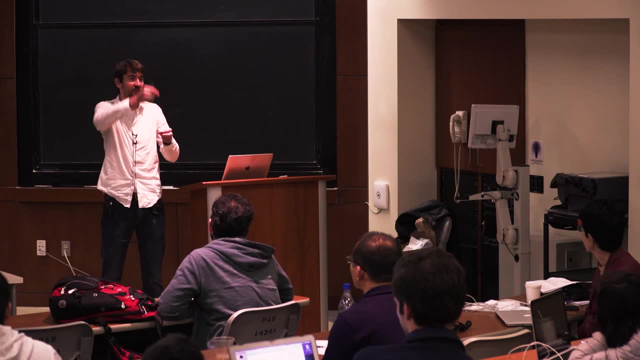 but there's enough that there are impurities in there And we know this because it takes them, for example, a while to purify their Xenon, right, So it takes months for them to purify the Xenon, so that they can just get a drifting length. 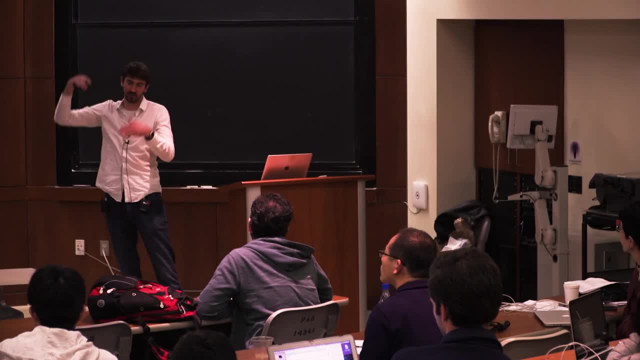 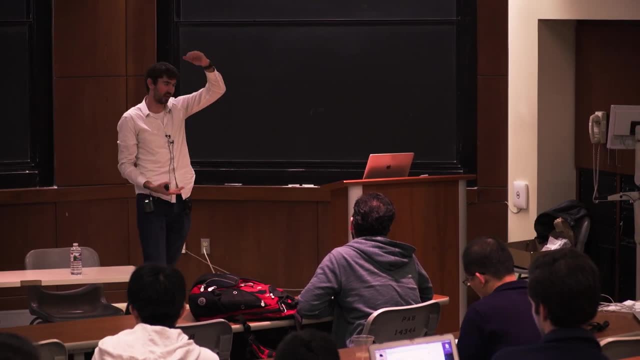 of what they need, which is the interaction chambers. So right, So Xenon, the next generation Xenon TPCs are about you know this, big or so. They're about a meter in size And they have to recirculate and constantly re-purify the Xenon for something like a month. 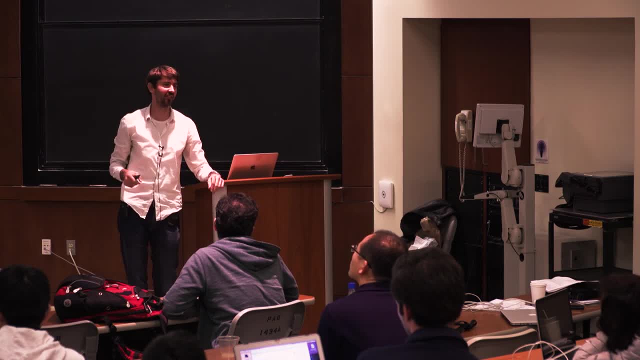 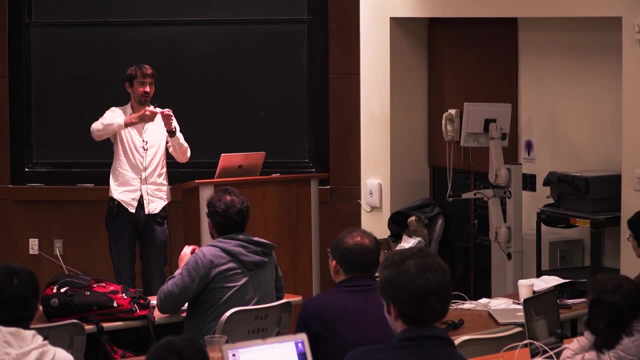 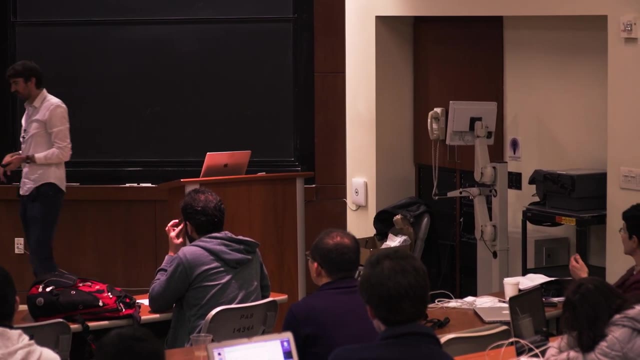 before they can make an electron travel across. So that right there sort of sets the scale that before cleaning for a month you need That electron which is drifting across will interact with an impurity in its little range. Yeah, So I think that's. 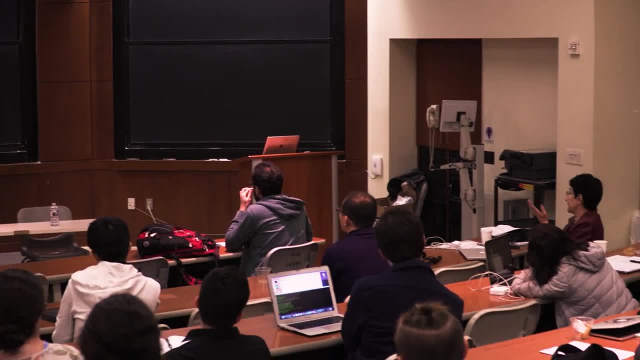 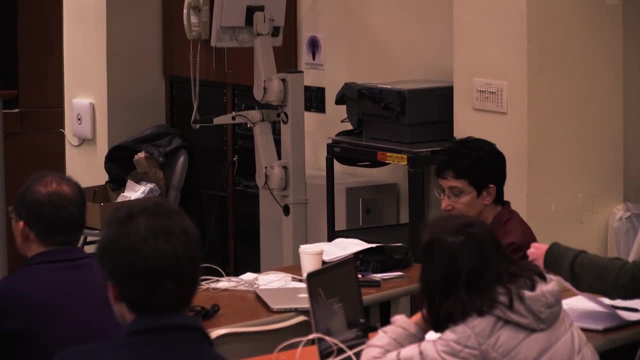 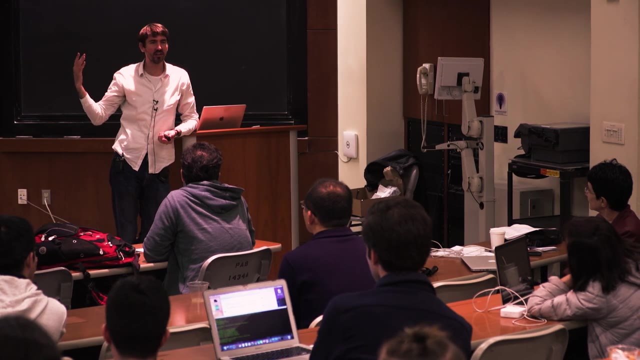 I thought it was really- I have no idea- but very small, very pure. Clearly it's giving them a background And I mean you need something like that, You need some interaction which will give you this secondary process, Because if not, it would work great. 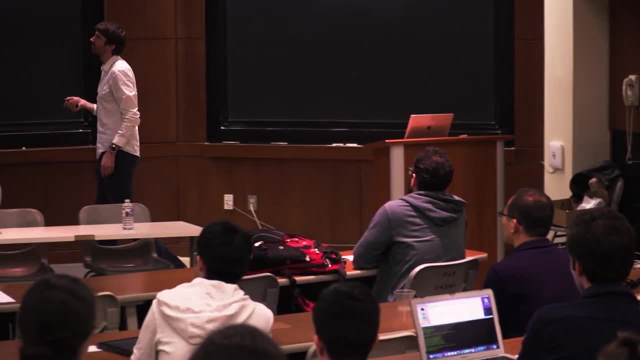 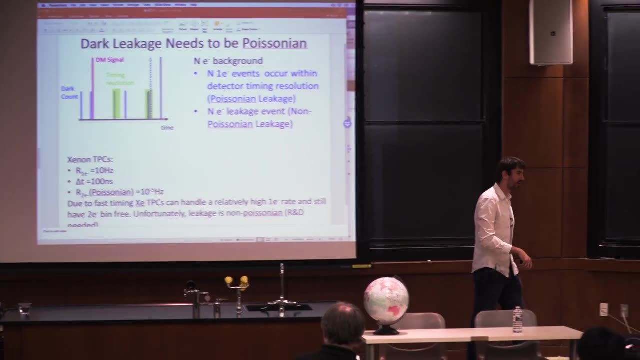 Like Xenon 10, has some kind of non-Ploisonian leakage event. It's not just two electrons piling up on top of each other. Do you know what I mean? I just wanted to ask, do you know? I must say I do not know this for argon. 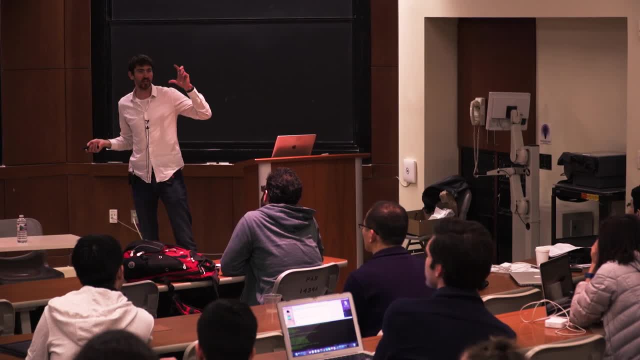 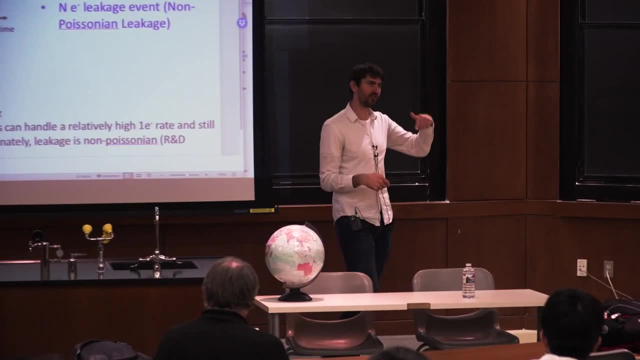 I will say that argon is a little more painful in that the rate penalty you pay. We talked about band gaps, So you are always paying this rate penalty and argon has a bigger band gap than Xenon, So you pay a rate penalty already for argon that's bigger than the one you pay for Xenon by a little bit. 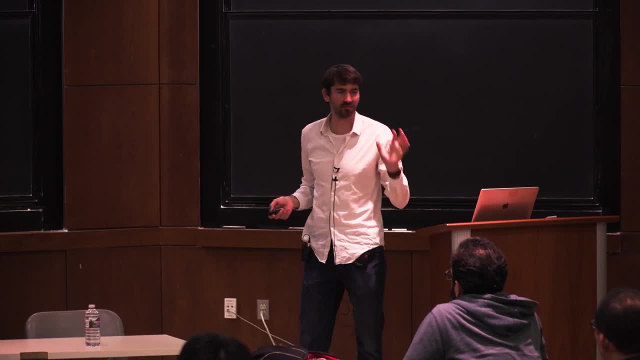 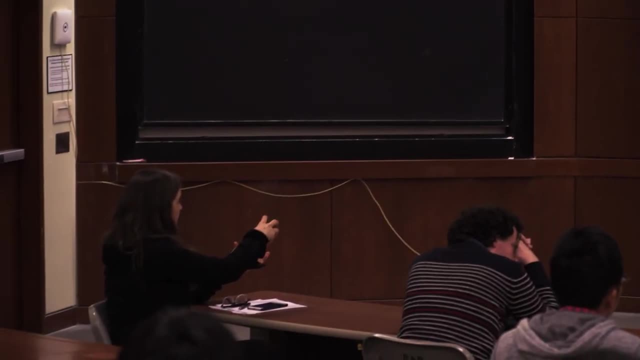 But I don't know about leakage currents in argon, I must admit. Yeah, Could you test this by running the experiment? with the dirty leaks you're on and just seeing are there tons more events than when it's like ultra-pure. 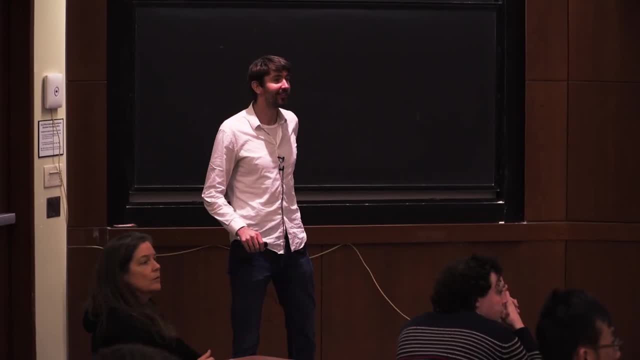 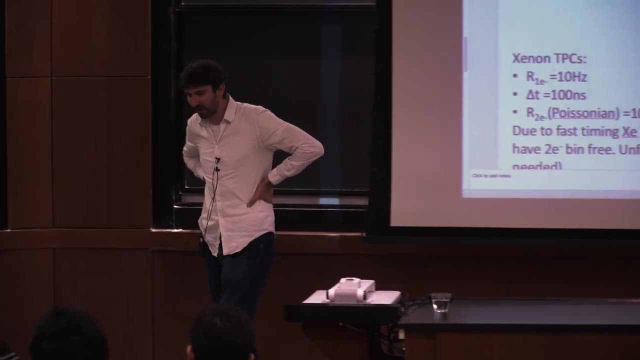 Yes, So they definitely are. Can you repeat the question? Oh, yes, yes, sure, Okay. so the question is: what are the experimental tricks you could figure out to figure out where these non-Ploisonian leakage events are coming from? 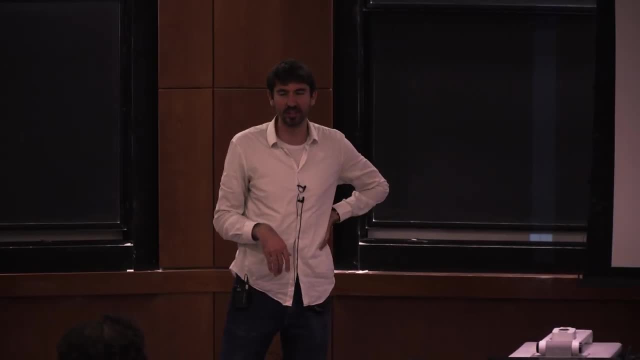 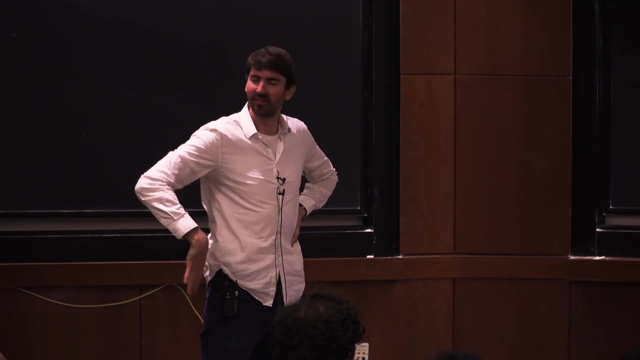 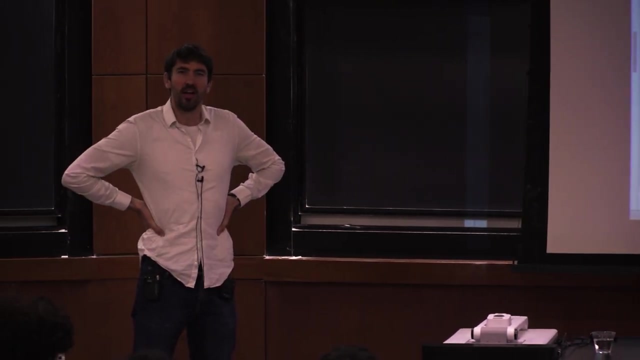 And one answer was: run it dirty, So leave some impurities. So I must say I haven't seen this one done, but it's a good idea. What I have seen done is: Let's see. so there is some discussion on if it's caused by Teflon. 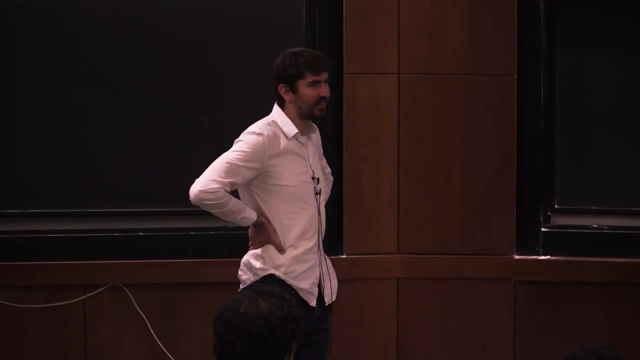 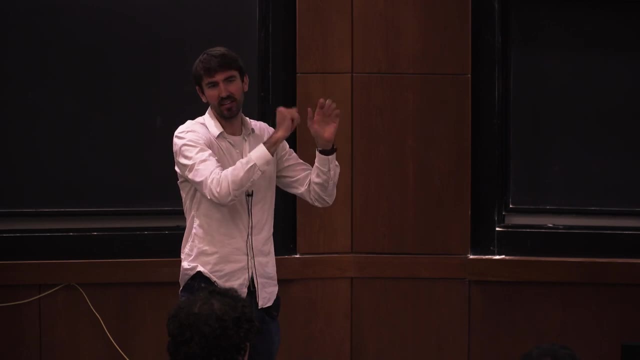 So another hypothesis is that it's Teflon, and Teflon is basically a glass. It's this really messy molecular thing and maybe it's storing energy and it de-excites and it'll shoot off a UV photon every now and then. 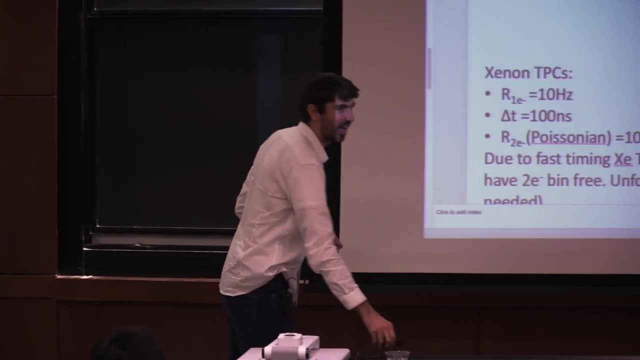 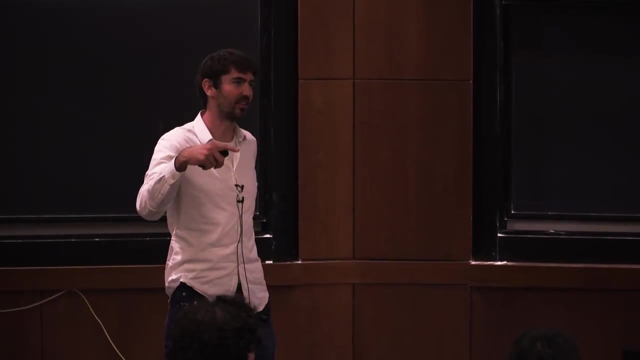 So this is actually seen as well. We know that Teflon has some is definitely giving you some scintillation, But still you need that scintillation then to come and give you an ionization. So maybe that's another scenario. 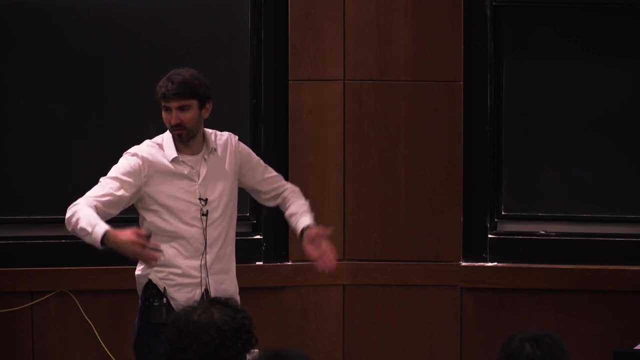 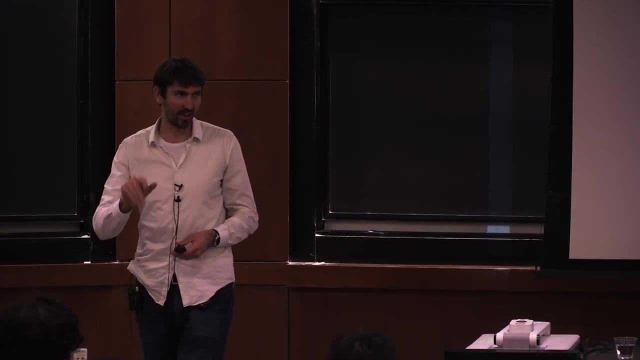 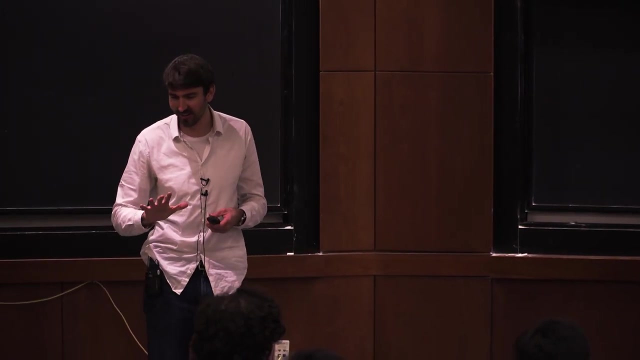 So I think people are planning on running without Teflon on the side walls. But then of course you lose your S1 signal. So you know you could just do a small experiment. that was a xenon TPC. It is definitely an area of intense R&D. 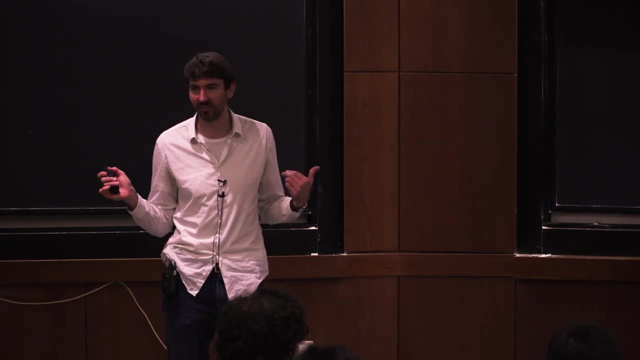 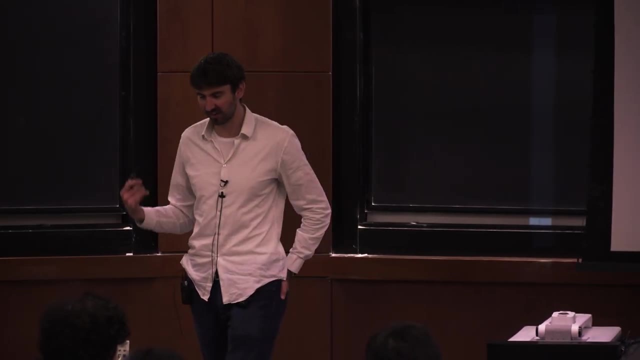 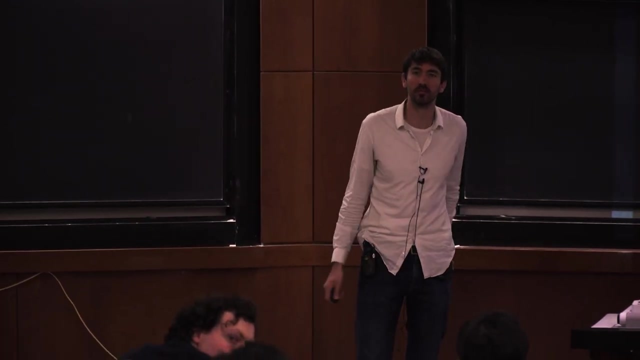 So it's not known as to what's actually the cause as of right now, But it's almost certainly at some scale. it has to be some kind of impurity states or something like that. Okay, Yeah, So actually you said the tiny resolution for the PMT. is about 100 nanoseconds. And if the second electron is caused by the UV ionization, is 100 nanoseconds enough for the electron to drift out to the next one? No, The drift time is a few microseconds. So yeah, depending on exactly where that occurs. 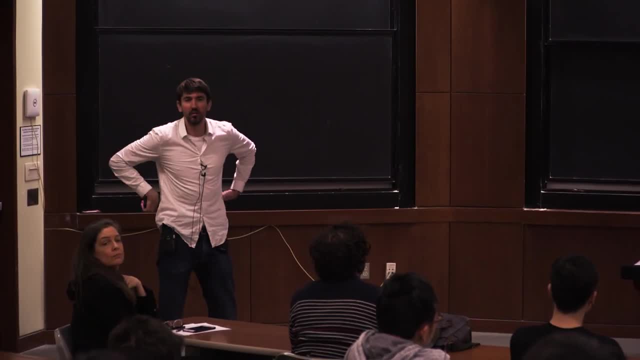 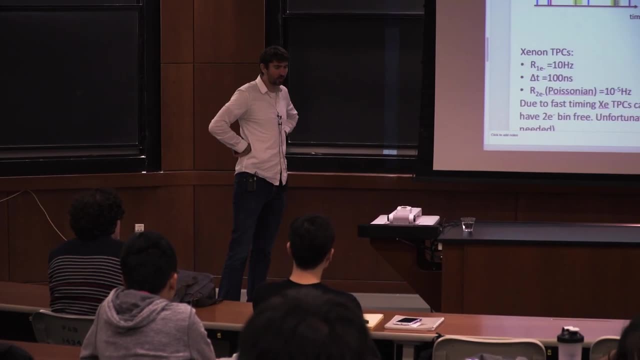 you may still be able to tag many of them, I see, But in that case wouldn't there be a timing, like a time correlation between the first event and the second event? Yeah, No, Yeah, So then only a certain percentage of them would pass your. 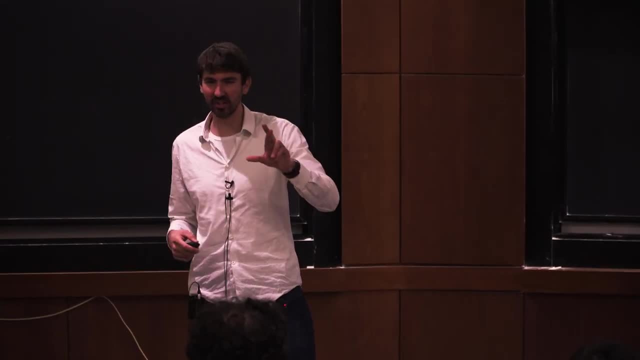 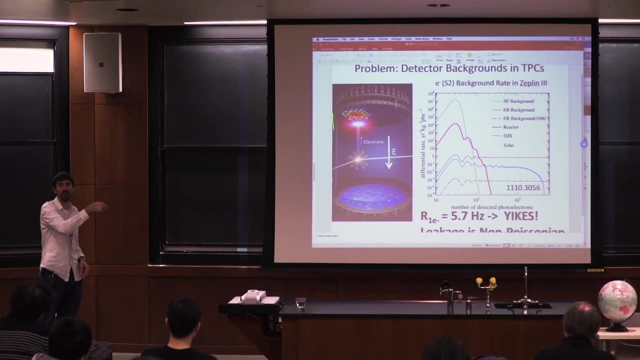 Yeah, So there it's. There would be a time correlation And the question is: is where in your xenon? If it occurs very near the top, then you can't distinguish. If it occurs down here, you could. So it's all about what that timing cut is. 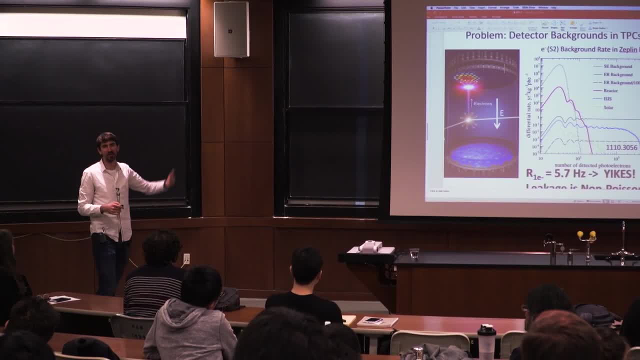 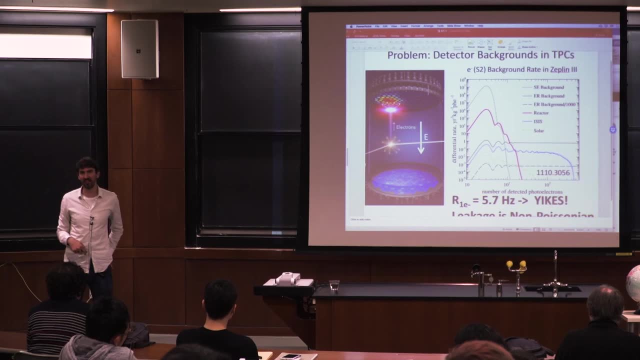 And yeah, so some fraction would be passed through. The fraction wouldn't be that 1e-6 fraction. right, That 1e-6 was set by us saying we had a 10 hertz background of single electrons with 100 nanosecond resolution. 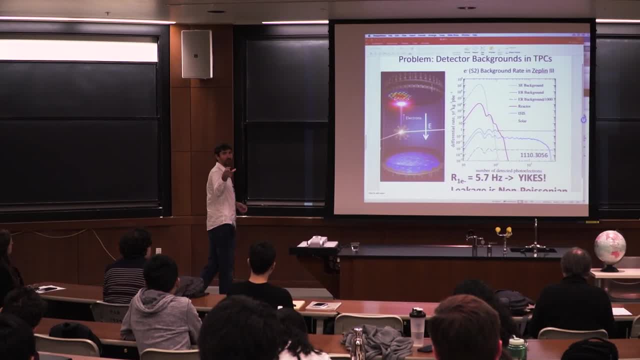 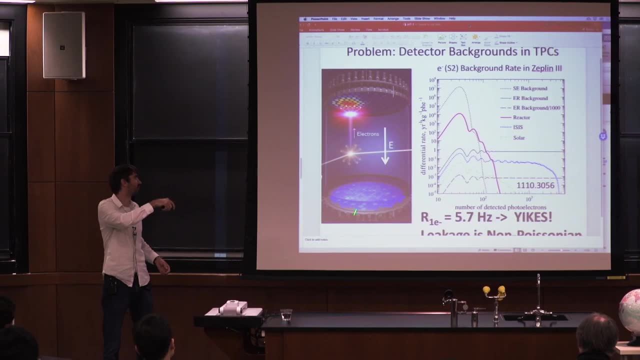 1e-6 of them would give us leakage If we had with this process. the one comes in. it gives us a second electron. I don't know. 10% of the time it gives you a second electron somewhere in the bulk. 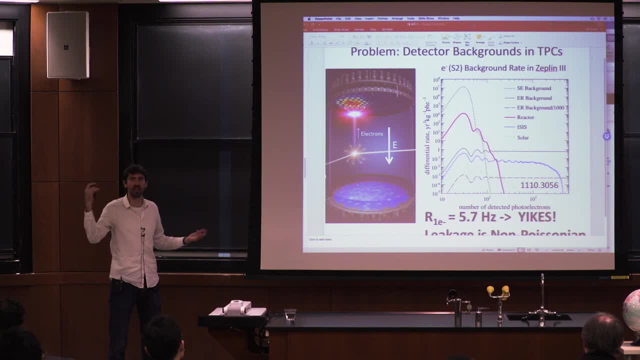 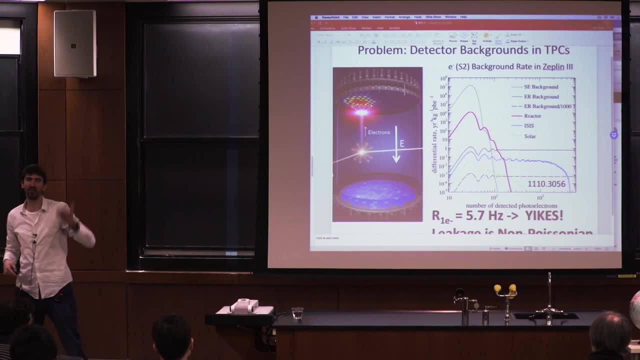 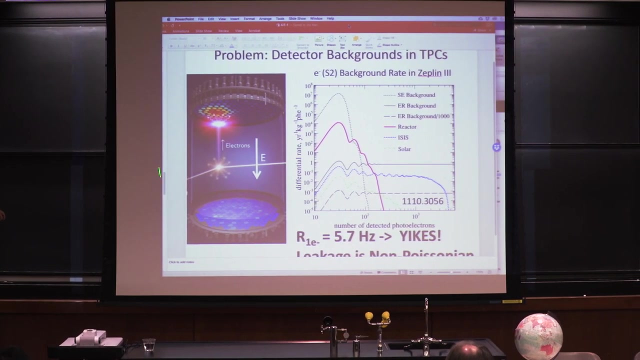 Then you ask: if the bulk drifting distance is 10 microseconds, then one hundredth of them. We'll pass your cut and you're still playing the game and you get hit again, right? So we really want to stop these multiplicative factors. 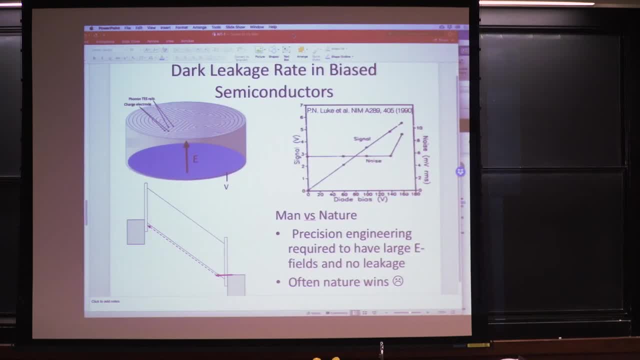 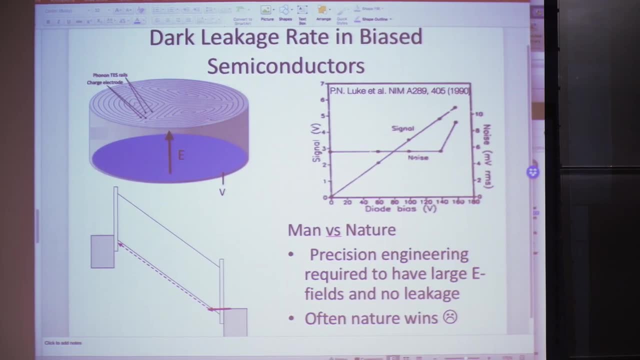 And we really need to get rid of this non-plussonian leakage. So this happens also in biased semiconductors. If we put an E field across a biased semiconductor, you get charge leakage. So this isn't just TPCs Any time, basically. 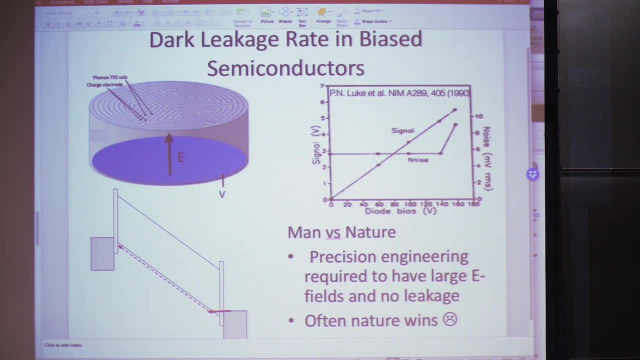 you put an E field across a system, you're putting it in a non-equilibrium state. So you're going to have some kind of tunneling rates. They want to be there And the key is you need to have precision engineering. So I'll talk about my experiment in the next talk. 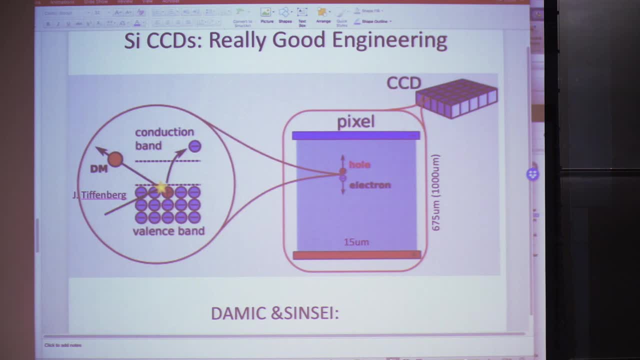 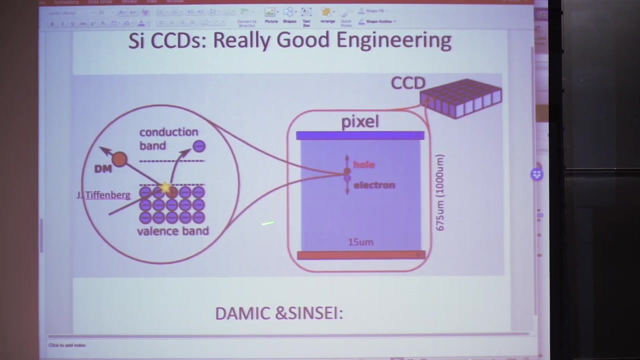 In this talk we'll talk about one place. we have precision engineering, and that's in silicon CCDs. We've spent many billions of dollars- probably DARPA- in developing this semiconductor technology, And so a silicon CCD is basically just again. 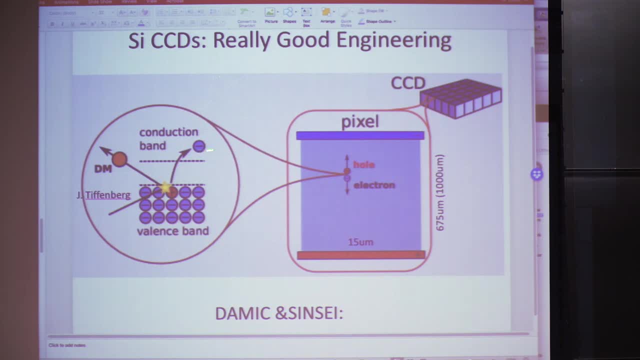 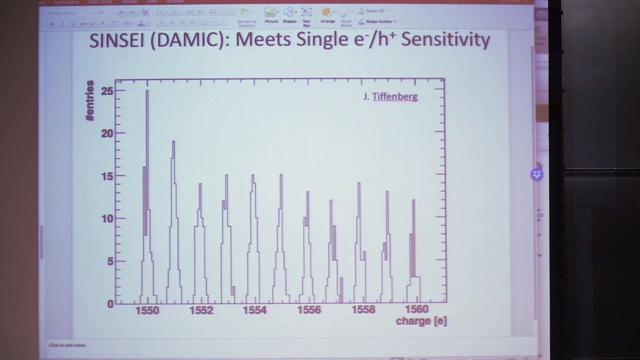 dark matter comes in, hits an electron, puts it up in the conduction band, the electron flies across, the hole flies across, and then we measure the ionization produced for the CCD, So CINSEI, which is basically the R&D arm of DOMIC. 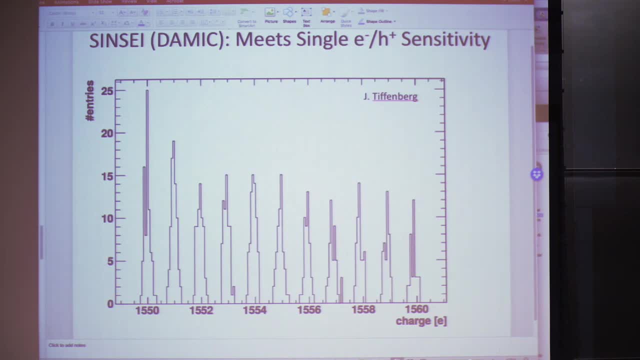 has actually just shown CCDs with single electron hole sensitivity shown here. So this is an event with 1,550 electron charges. Here's one with 1,551.. Oh, okay, so DOMIC and CINSEI are an experiment. 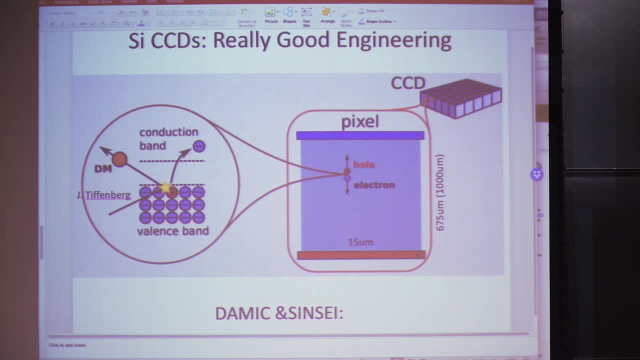 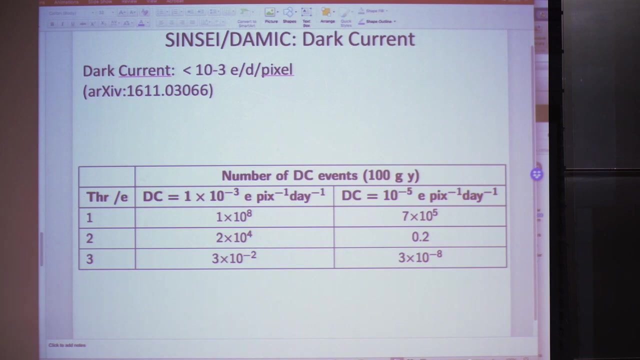 that use CCDs to search for electron-recoiled dark matter. So now we've just talked about this idea of charge leakage. and so what is the charge leakage rate that DOMIC sees? So they've only set an upper limit. It's 10 to the minus 3 electrons per day per pixel. 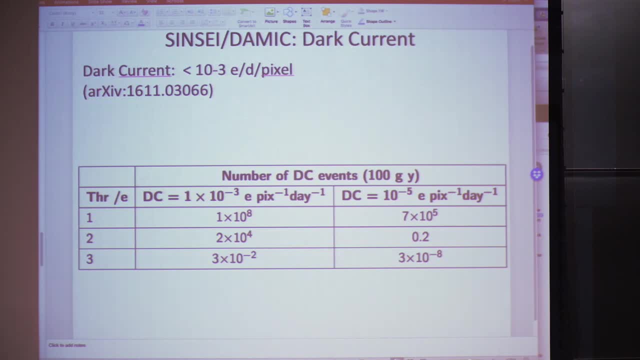 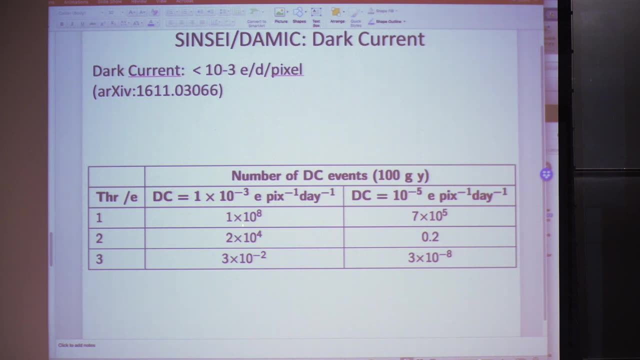 And if you put that through, the problem is that's pretty small, The pixels are pretty small, That's a pretty small number and you're like score. The problem, unfortunately, is that the readout time takes 3 hours. 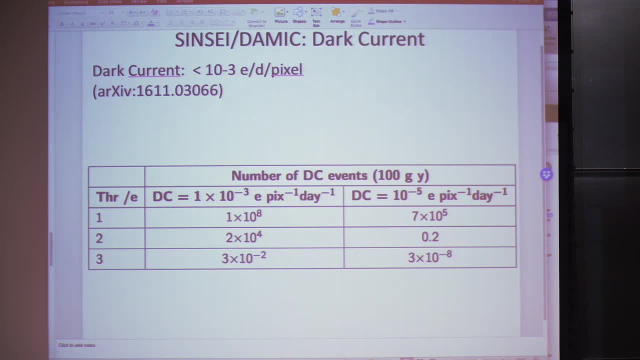 So with XENON, we were talking about 100-nanosecond timing sensitivity. With DOMIC and CINSEI, we're talking about 3-hour timing sensitivity. So you really have to ask the question: what are the odds of getting two single-electron leakage events? 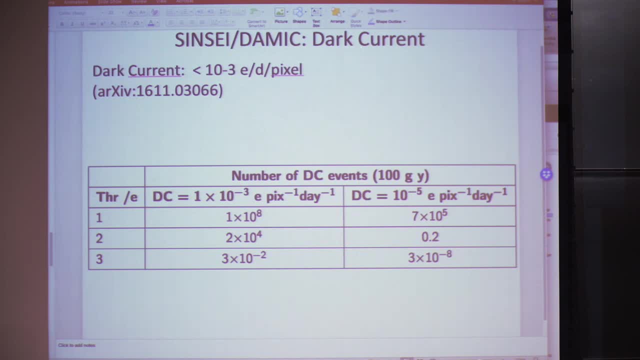 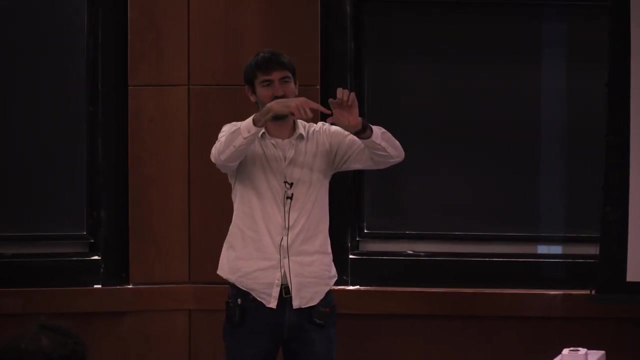 within a pixel in 3 hours. So that's your Poissonian rate. So do you guys know how CCDs work? CCDs are just little ionization detectors. It has a pixel. You produce, let's say, one electron-whole pair. 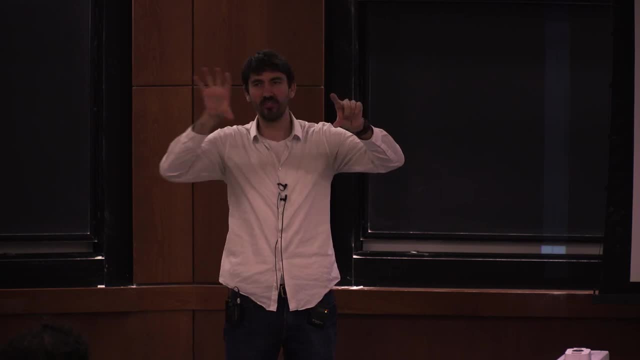 and an electron gets stuck here. So you have, let's say, 10 to the 6th of those pixels in an array And the pixel has pretty huge capacitance. charge capacitance, It's a big thing. Charge capacitance scales with area. 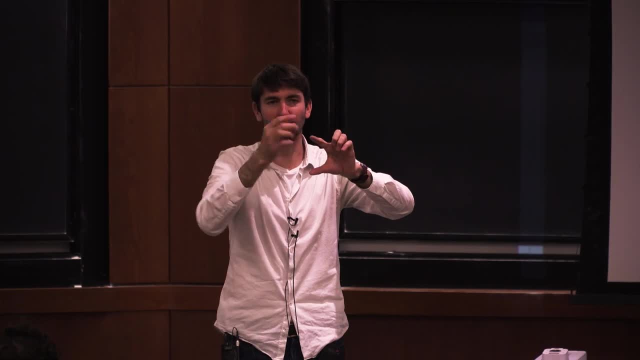 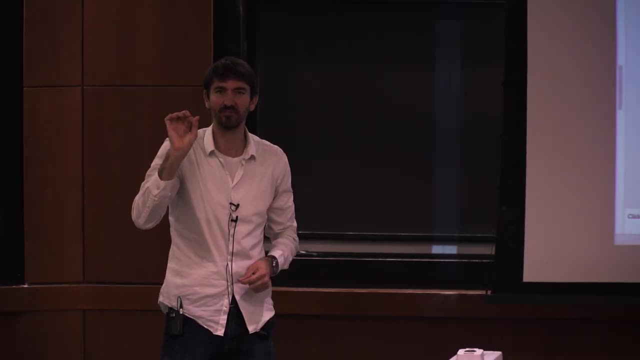 So you're like: uh-oh, So what you do is you actually transfer that energy from here to a small measuring device that has an incredibly small capacitance, And that's how you get the sensitivity. So you actually transfer this one single pixel. 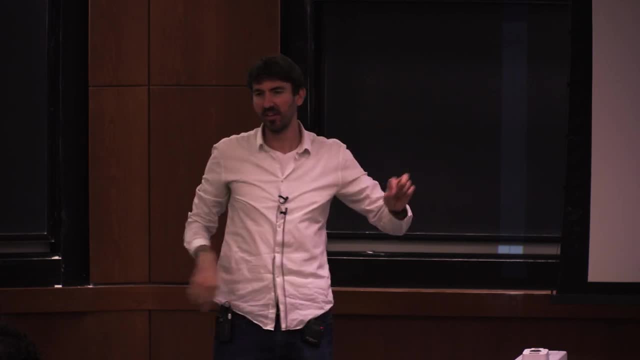 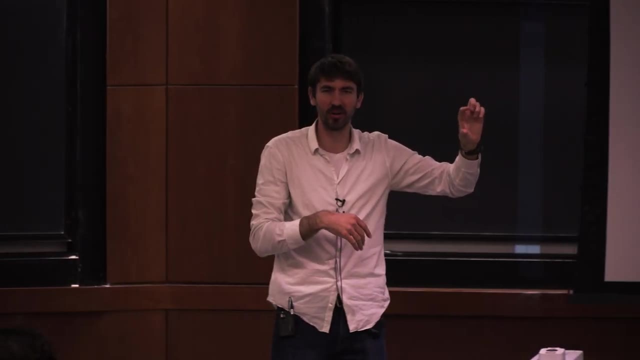 to a sensing pixel which has excellent sensitivity. It actually is even worse than that. It turns out that that sensing pixel still has 1 over f noise. All of electronics always have 1 over f noise And therefore they actually transfer it over. 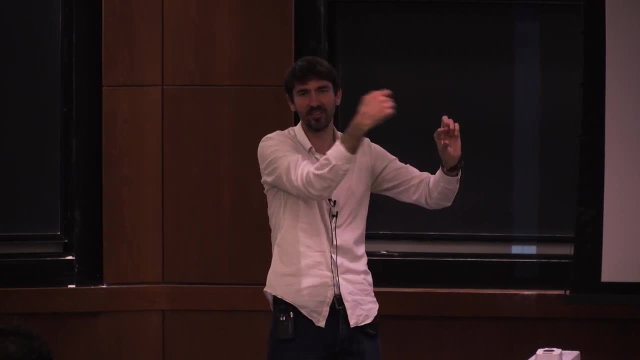 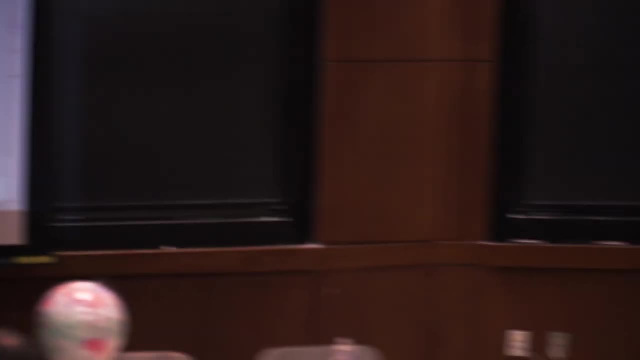 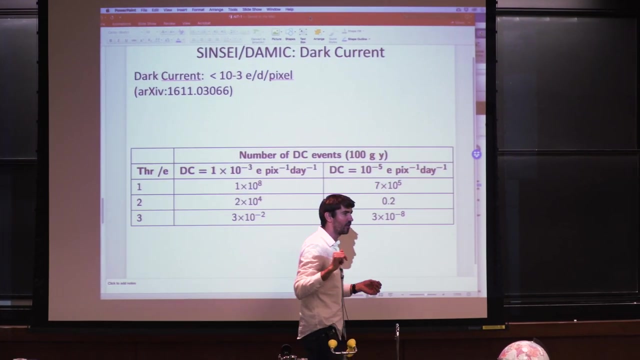 and take it off, and put it over and take it off multiple times to get to this single electron sensitivity. What about the frequencies? What is 1 over f noise? So 1 over f noise is just a lot of it. It comes from many, many different physical sources. 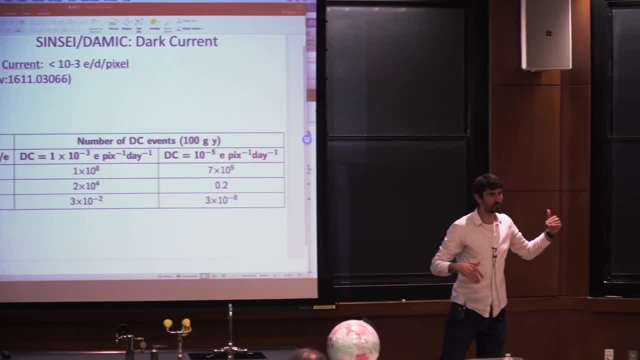 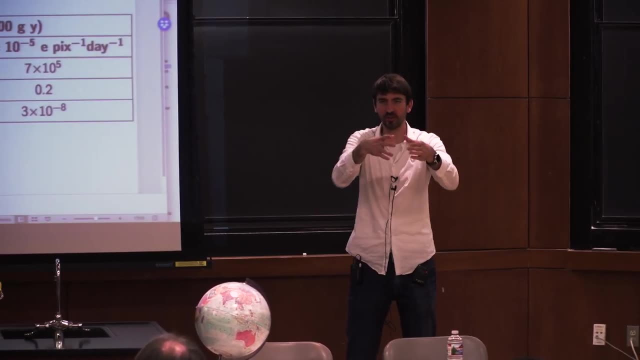 But it's a noise which gets bigger the lower in frequency you go. So that's why this is a DC measurement, So you can't just let it sit there. In some sense, if you let it sit there and you measure 1,000 times, 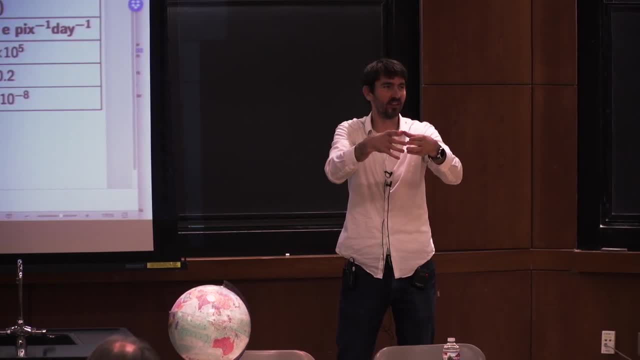 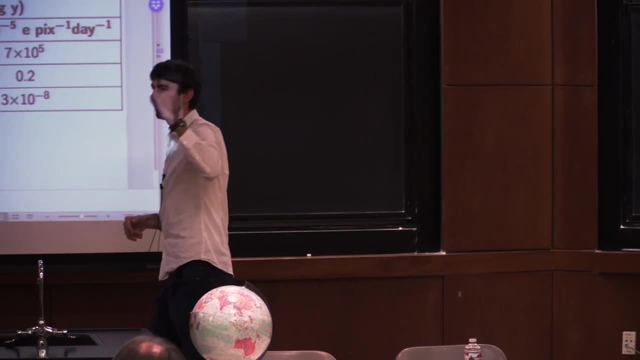 you would say, oh, I would improve my sensitivity significantly Because of 1 over f noise. it doesn't. Your DC noise is actually very, very big, So you have to somehow break that. So the way Domek and Sensei have broken this, 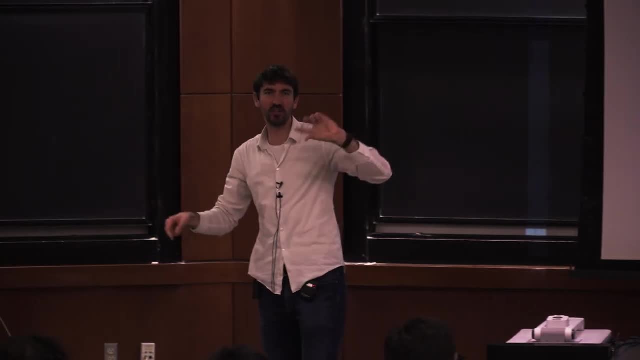 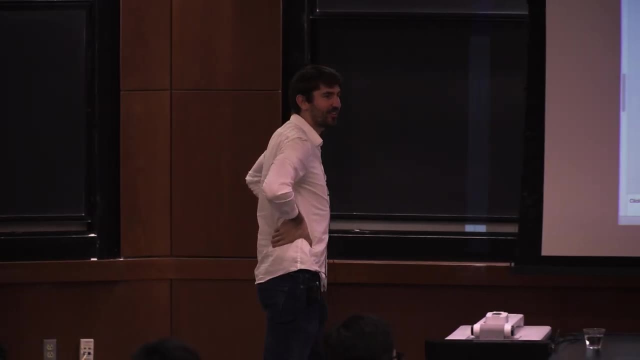 is they actually take it on and off. So your DC noise randomizes every time you take it on and off And then they can do the square-rhythm statistics. It's a very nice measurement. This is very. You know, CCDs don't usually have 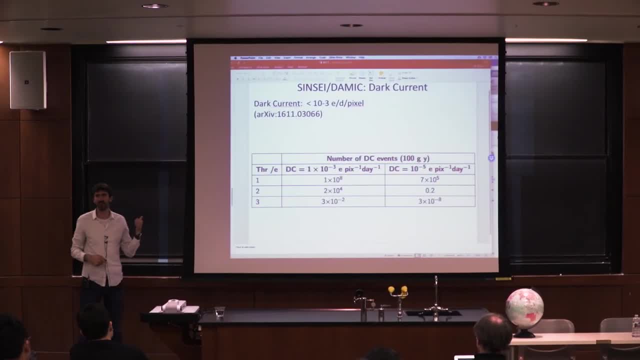 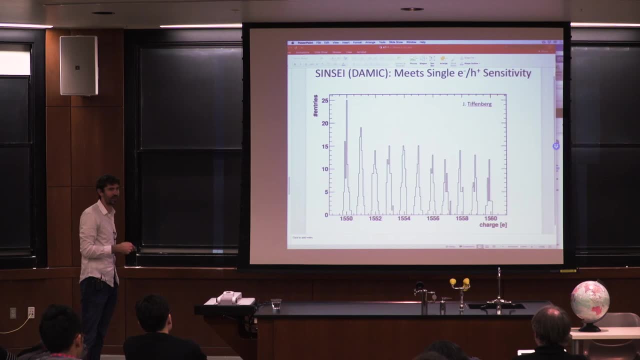 .0.. I think it's .07. electron hole sensitivity, right. This is a very beautiful device And it requires a special readout, But that readout takes lots of time. You have 10 to the 6 pixels. You have to read every one out. 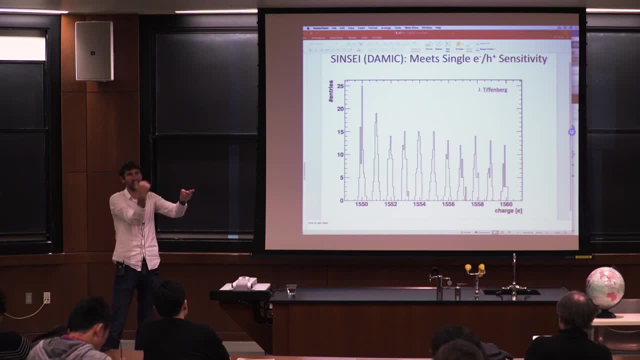 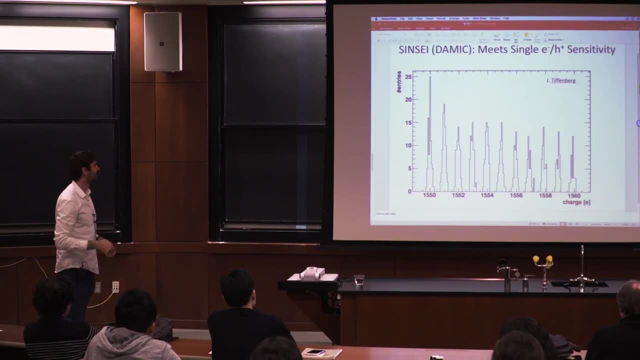 by this little sensing pixel, And to do it you have to read it out like 30 times and you have to kick it back and forth, And so that's why it's three hours. So that's a bummer, But anyway. 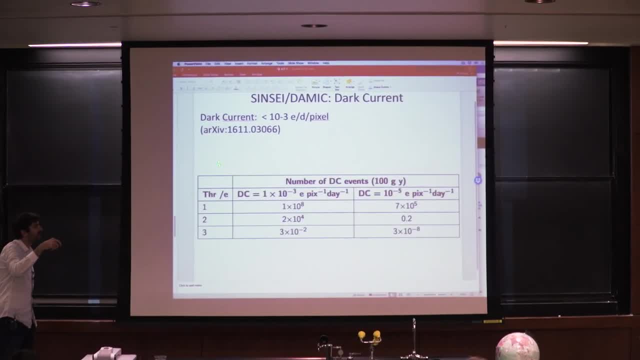 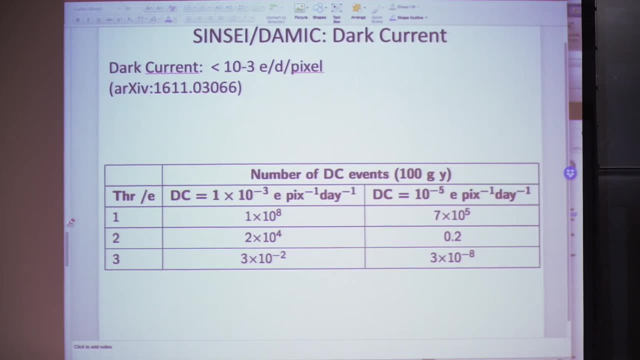 let's look at these Poissonian numbers. So they have not seen any evidence of a non-Poissonian tail. So, unlike Xenon TPCs, they don't have this non-Poissonian tail. And here are the leakage events that they would see. 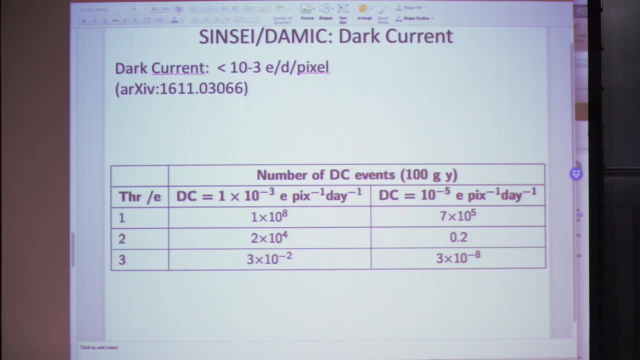 in 100-gram-year exposure. Their single electron bin is just dead. It'd be 1e to the 8. But their 2 and 3 electron bins are awesome, right, So here their 2-electron bin is questionable. 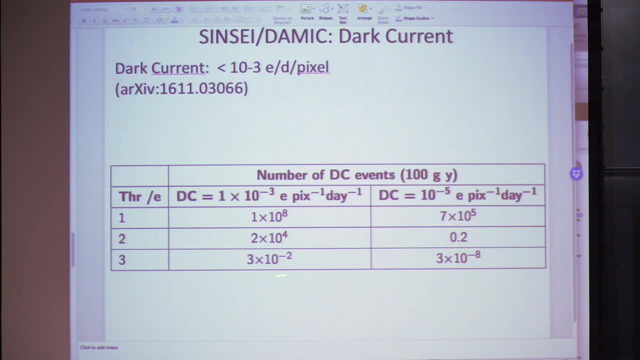 You know, 2 to the 4, so they can't hit their backgrounds, But their 3-electron bin. that one actually has single-electron sensitivity. So that would be the bin one would search and would give you the best dark matter sensitivity. 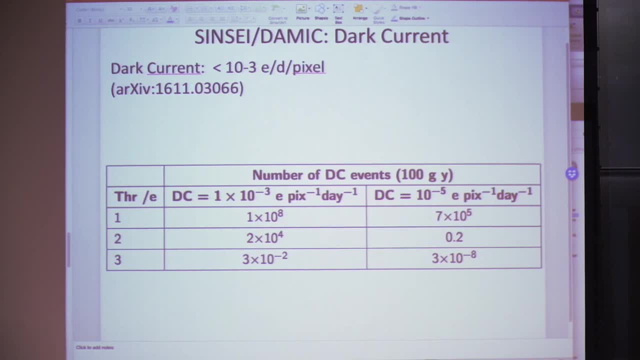 would be searching for dark matter which produced 3-electron whole pairs, And of course this is only an upper limit on their pixel on the background. If it was lower 10 to the minus 5, then you could also search in the 2.. 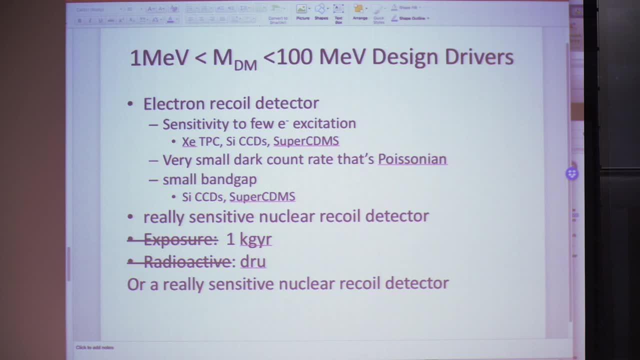 Okay, I'll talk about my experiment, which also shows single-electron whole sensitivity, in the next talk. So so far Okay. so here are the design drivers in this range. So you must have sensitivity to single-electron whole pairs. 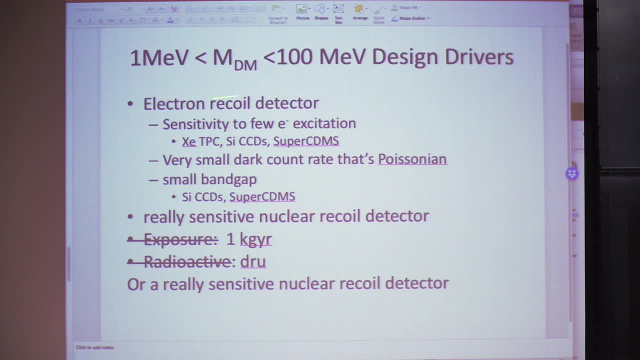 2-electron whole pairs. 3-electron whole pairs And the experiments that we've shown this are xenon, TPCs, silicon, CCDs, super CDMS. So far, we need to have a very small dark count rate. that's Poissonian. 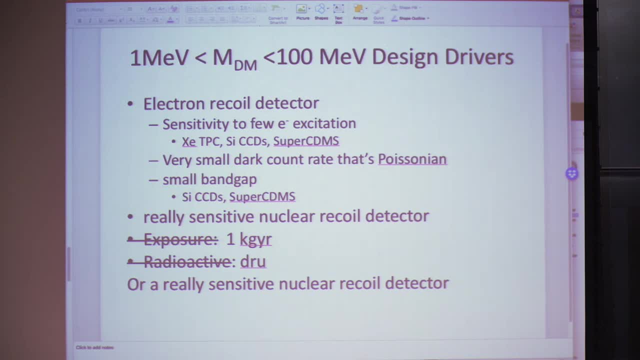 and has no non-Poissonian component. By the way, PMTs have a horrible non-Poissonian component And another way you could go is just have a really sensitive nuclear recoil detector. Again, the exposure is small: one kilogram year. 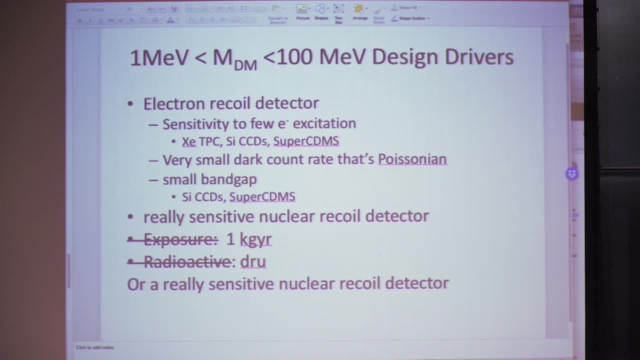 not a big deal, But it's really important to get really meaningful limits. So we're not talking about 10 tons. This is all you need is a kilogram, And the radioactivity limits are a DRU. So one event per KV. 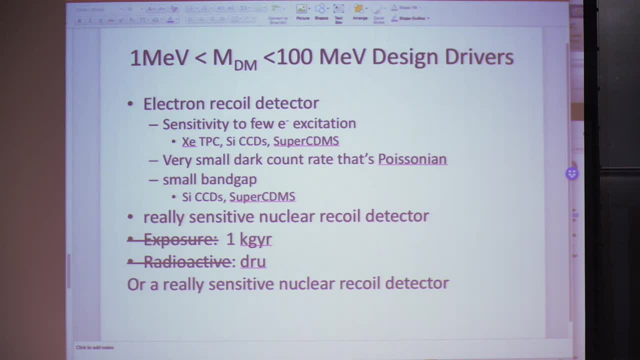 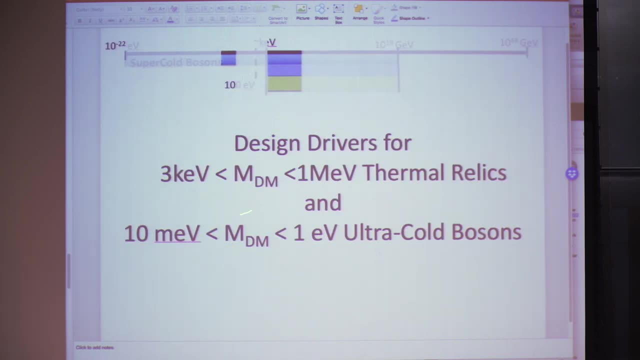 per kilogram per year, per day is all you need. So it's again manageable in today's world. So now let's go the next step down, which is 3KV to 1MeV thermal relics, to search for those. 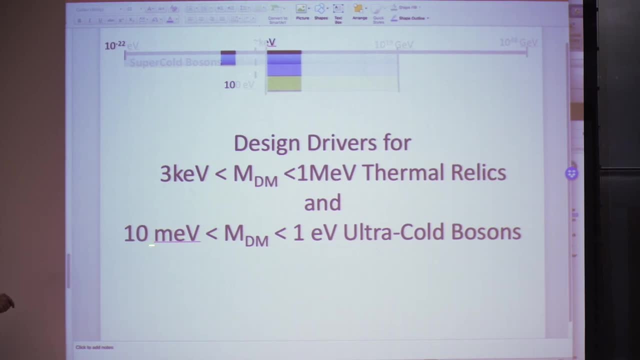 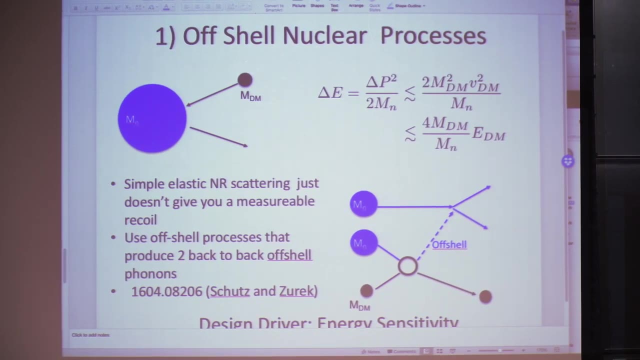 And to search for ultra-closed bosons, which go from 10 MeV to 1EV. Oh, we're already. okay, I'm sorry, Okay, okay, I'll finish quick. So the first step you could do is off-shell nuclear processes. 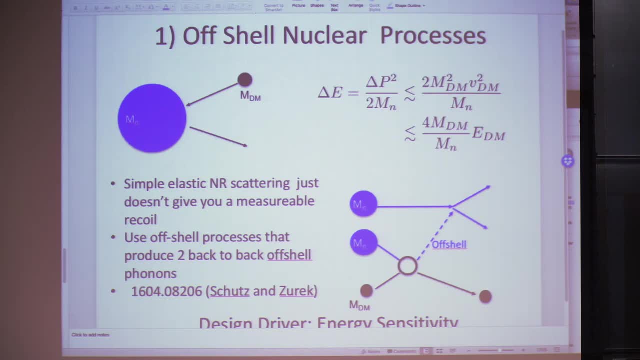 Again, you pay that penalty, but you could go off-shell. So here is so. Katherine Zurich proposed this with helium. So you have a dark matter. come in, hit a helium nucleus, You have an off-shell process, so you don't have to conserve. 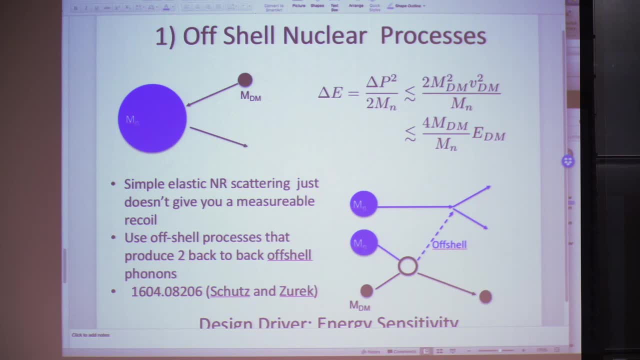 momentum and energy And you make two phonons back-to-back, So basically two phonons back-to-back. Helium is really, really massive And it is very, very slow compared to this dark matter. So if you want to conserve, 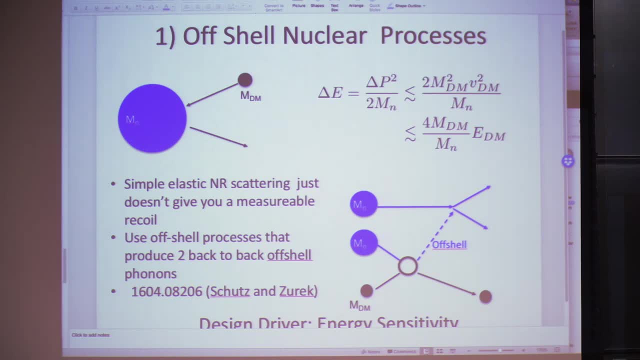 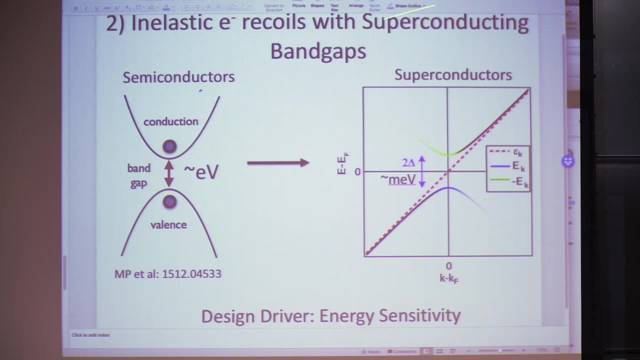 energy and momentum. you put the momentum of the two nuclei back-to-back, So you know you pay a penalty. Secondly, you could do inelastic electron recoils with superconducting bandgaps. Basically the same concept as previously. 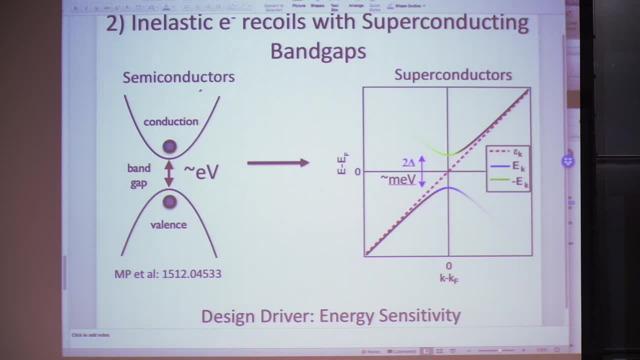 The momentum-energy conservation is not exactly the same as with electron recoils, But again you can basically conserve for momentum And the gap is small. so you're sensitive at very light to very light mass dark matter. Here the problem is energy sensitivity. 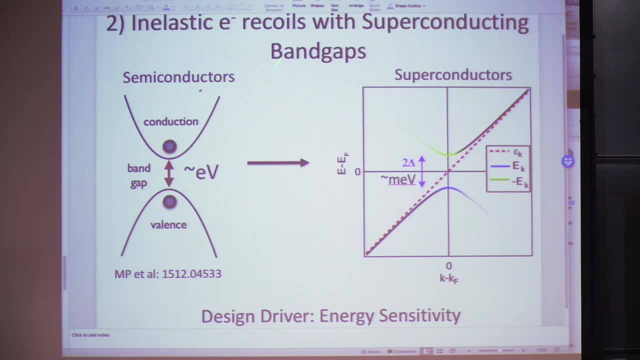 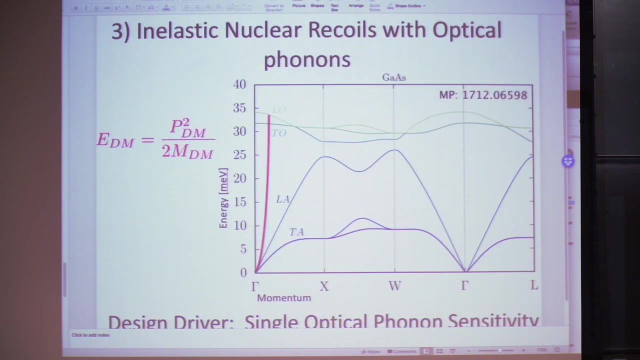 You need to read out, you need to come up with a thing that will see quasi-particles at the. you know that'll see one, two, three, four quasi-particles. So in terms of energy scale that's four millivy. 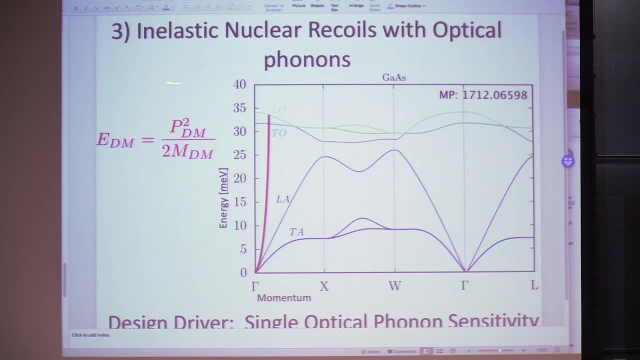 Finally, here's one that I really like You could look for: inelastic nuclear recoils with optical phonons. So here is another band. This is a band of the quantum vibrations, so the phonons in a system And the energy scale here. 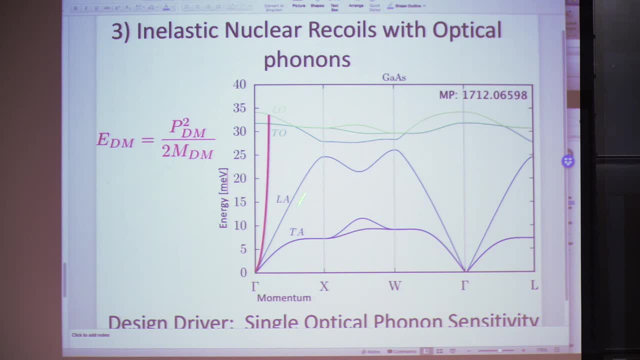 is 40 millivy And you have an acoustic branch and you have an optical branch. So why do we call these optical phonons? We call them optical phonons because they conserve for momentum very, very well with photons, right? So if you look at a crystal in the IR, 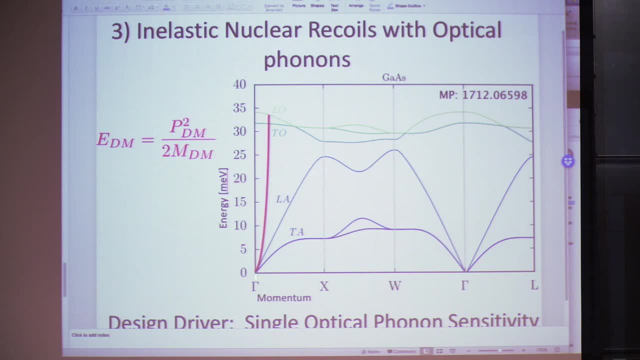 it looks black. And why is it? Because you can conserve for momentum. So if I think of a photon coming in here, it's a very sharp line. And I have a photon of an IR energy. I can absorb it completely onto a logical. 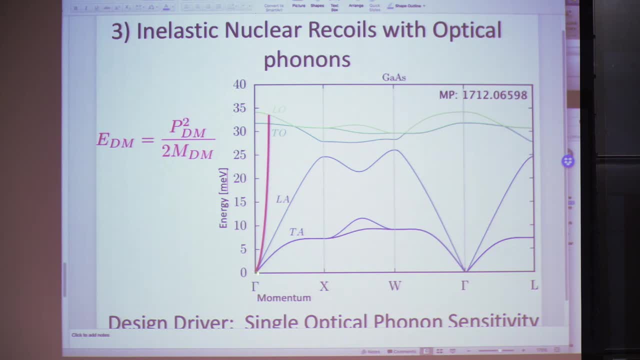 on the logical optical phonon. The same is true for very light mass dark matter. Here it's a parabola. But again, if I have a light mass dark matter with p squared over 2m right here, I can absorb. 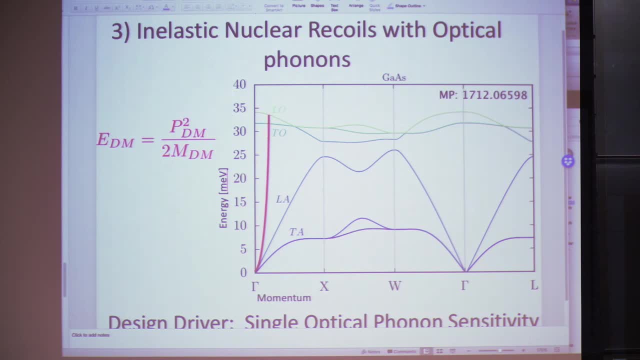 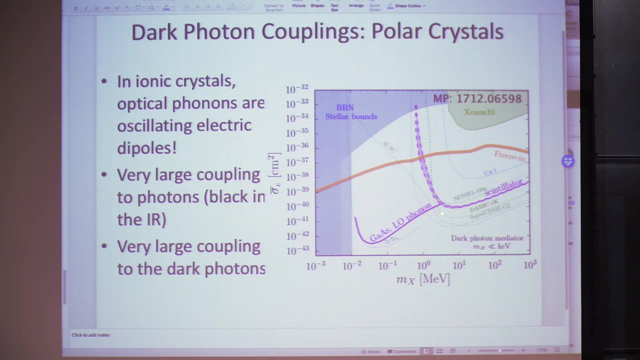 I can scatter off of it. I can take all of its energy and create an optical phonon. So here the design driver is a device that has single optical phonon sensitivity. So here is a paper that we wrote on this And you can see the sensitivity. 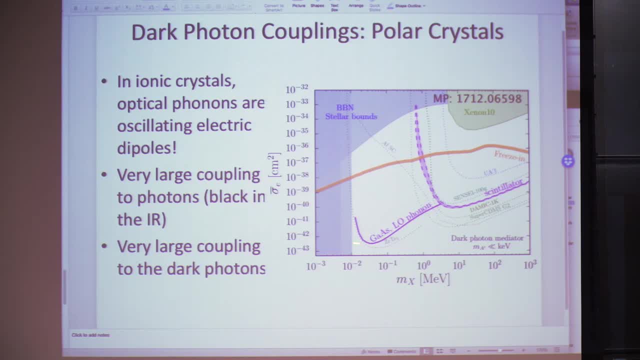 is incredibly enormous. It's below this 1 MeV to create. so here we have a dark photon mediator where we have dark matter scattering via a dark photon, which was talked about in the slide before me And the. you know this is such a great curve. 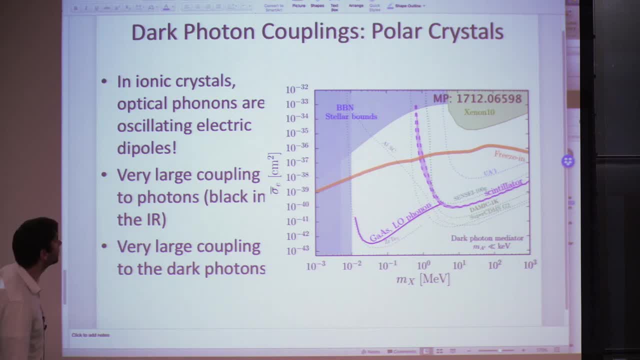 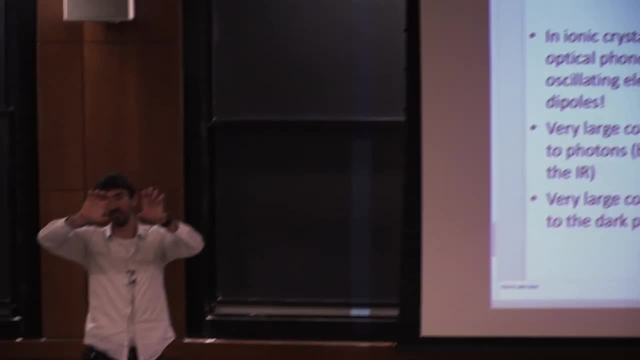 And why is this curve down there so low? And that's only because of polar crystals. So when I think of a polar crystal, I have an ionic crystal, right. I have sodium, I have salt which is sodium chloride, So I have a plus and a minus. 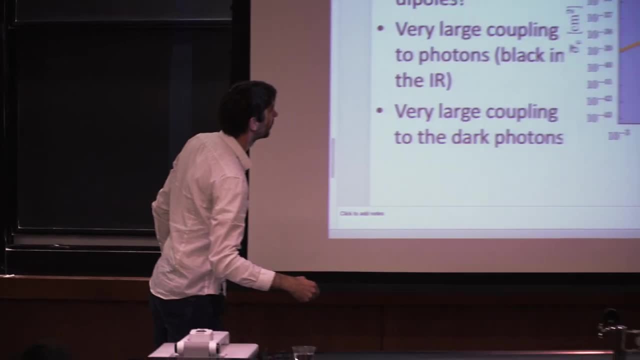 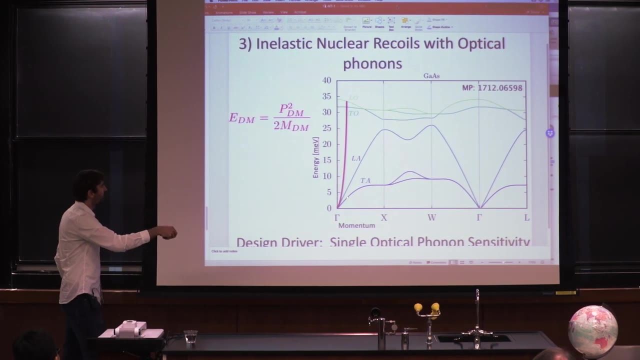 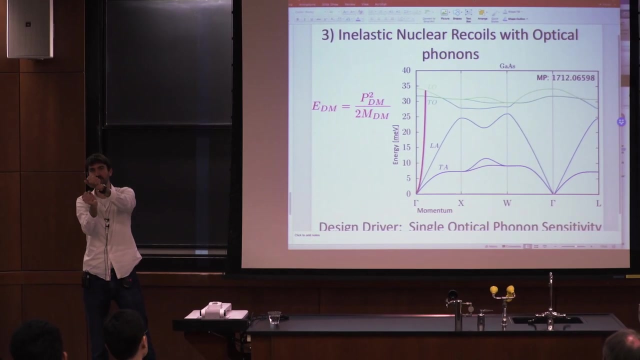 These vibrations that we are seeing, these two branches. so the acoustic branch is when I have those two atoms moving up and down together or moving to the right together. So that's the acoustic branch. All the atoms in a Berlin zone move together. 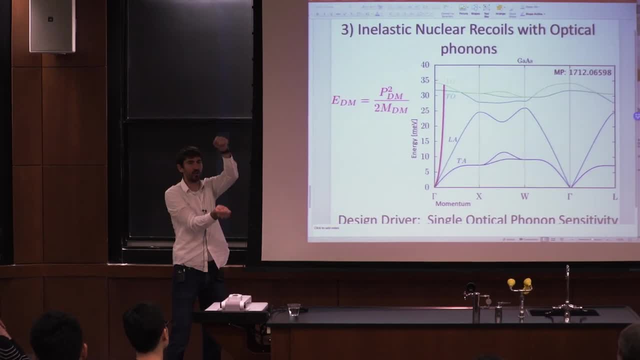 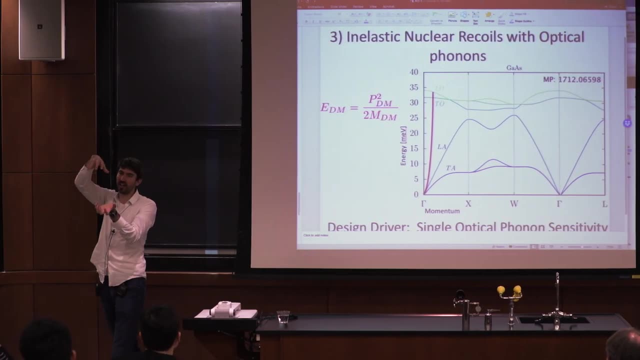 and are displaced together. The optical branch is when those atoms move against each other. So it's this, this movement, or this moment. And if you think about what I have, if I have a polar material, if I have a polar material and I have an optical phonon, 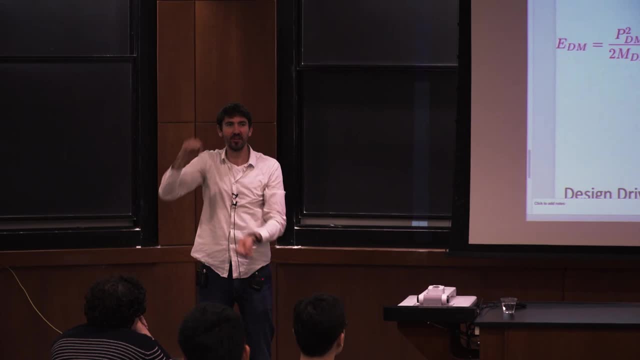 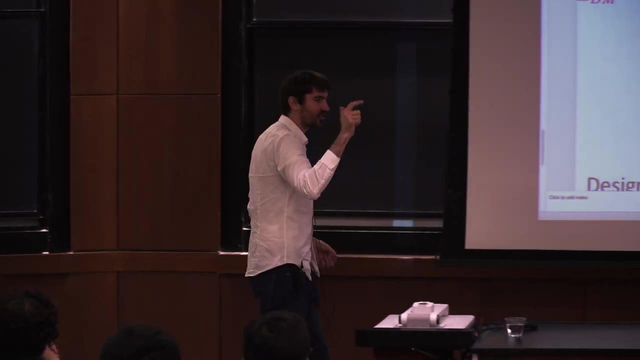 I have a plus and a minus vibrating like this, right, So I'm changing the dipole. or if I have a dipole like this and I have it like this, it's going like this, So I am naturally coupling to the truest sense of that photon. 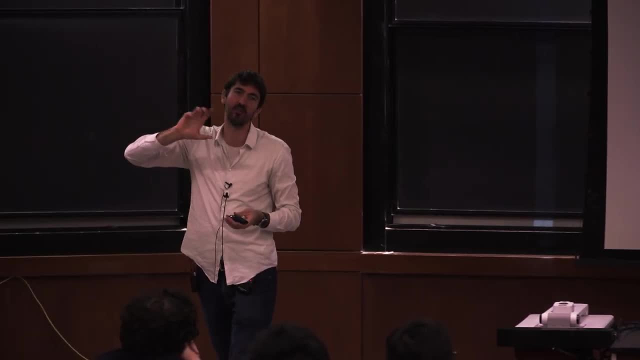 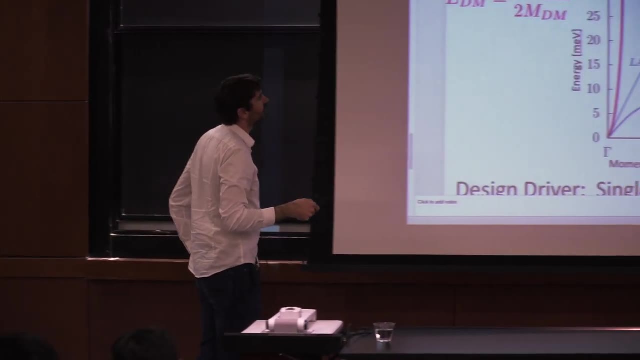 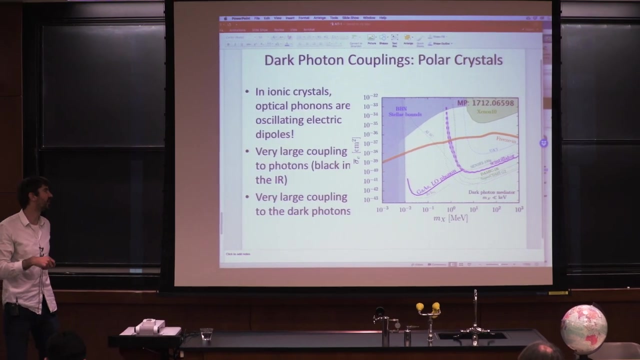 I'm accelerating the particles around, I'm scattering very well, I'm absorbing very well because I have this perfect electromagnetic coupling And that's why this is so strong and that's why these limits here. for any kind of dark photon mediator it's very hard to come up. 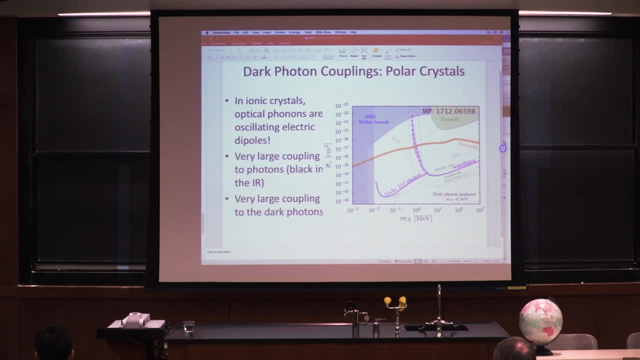 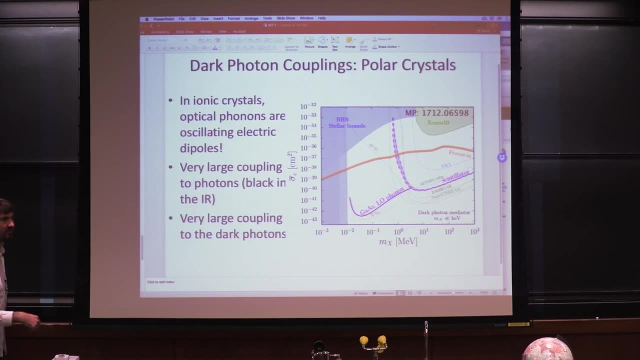 with another material that has this sensitivity because intrinsically it's so strongly coupled to a photon, which means it's so strongly coupled to a dark photon. So anything that goes through dark photons, this is a really nice technique to go for. So, finally, 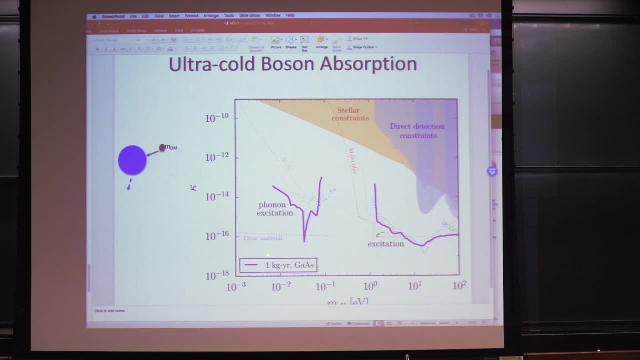 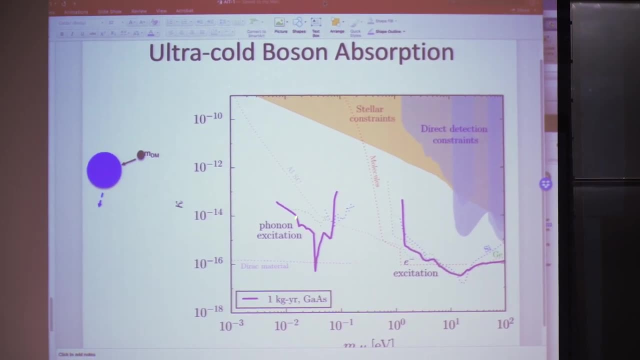 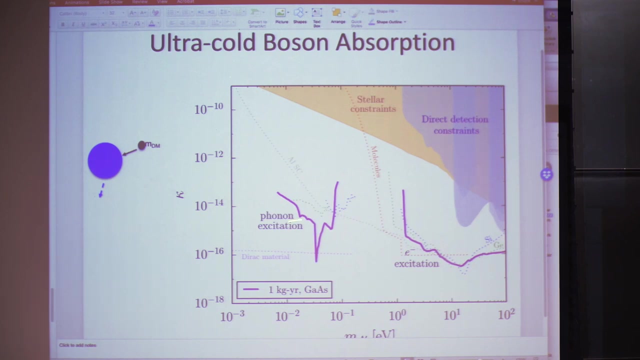 the same thing works for ultracold boson absorption. Here is again. this is for a dark photon. You have this very nice sensitivity in a kilogram year, Way below you know, something like on average 10 to the minus 15,. 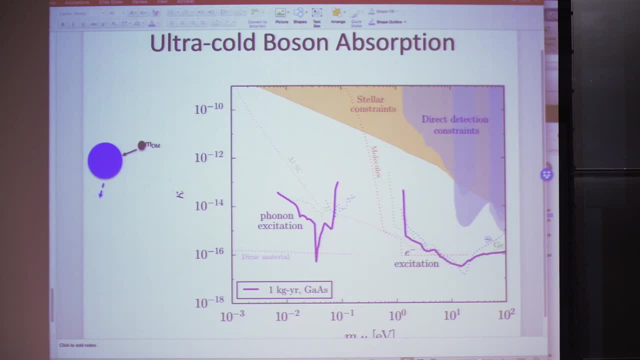 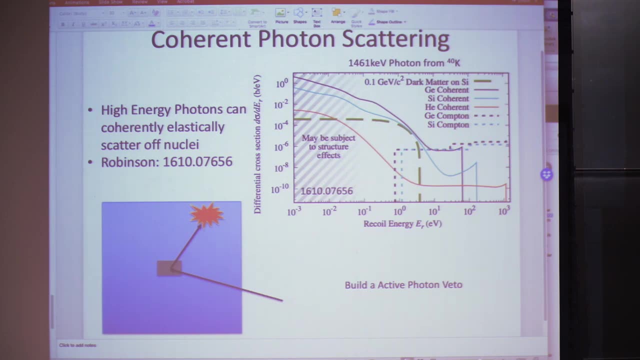 the limits are 10 to 10,, 5 orders of magnitude better than what we currently have. So there are some backgrounds down here that break the rules, which is radioactivity. There's coherent photon scattering, And the moral is that you just have to put this: 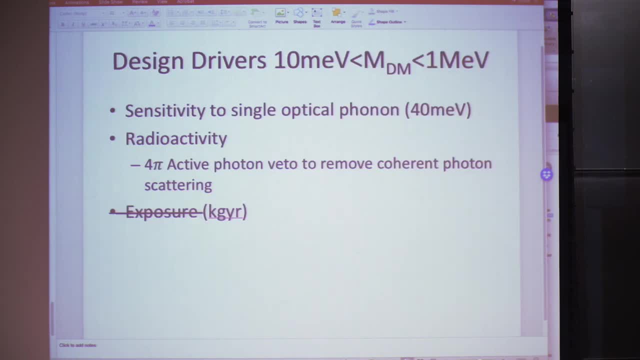 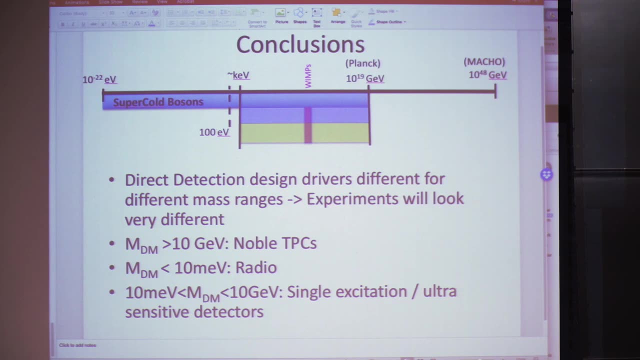 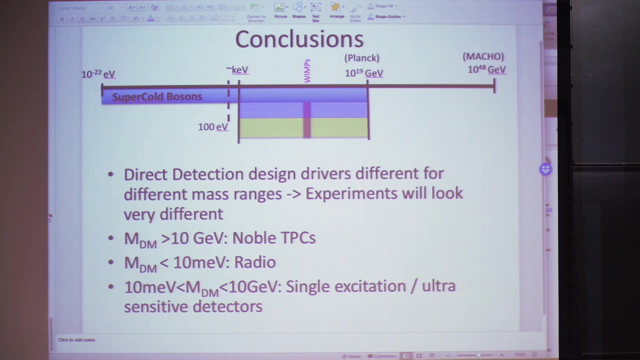 in a photon veto, in an active photon veto. So here are the design drivers in summary. So our conclusions are: in every one of these ranges we have different design drivers. As we go down in mass our rates get bigger, so we don't need as much exposure. 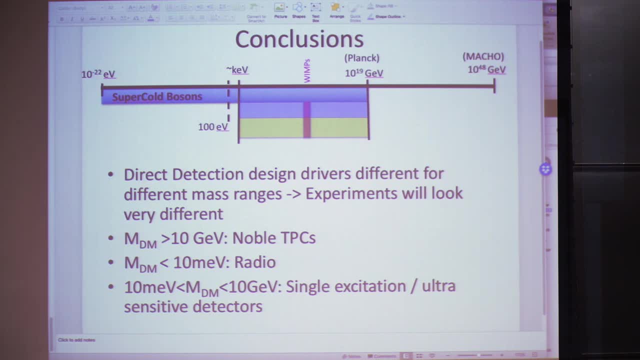 As we go down in mass, no matter what process we're looking at, the characteristics, energy scales of what we're looking for become very, very tiny. So as we go down, we always have to get better and better sensors. There is one scale. 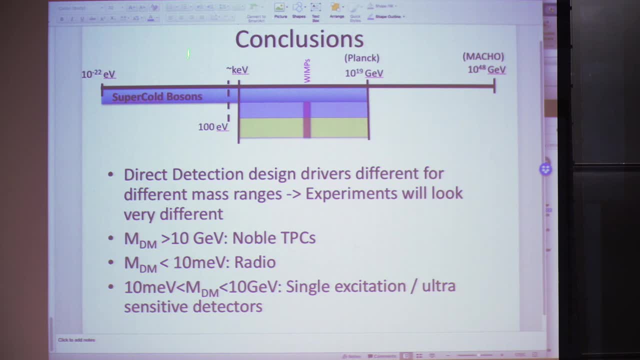 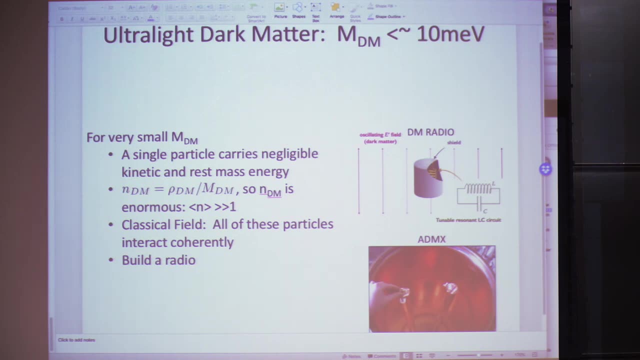 where this actually stops being true, and that's actually the 10 milliV scale, And below 10 milliV is here. Now you have so many parts of particles in a single quantum state that the quantum density becomes greater than one. 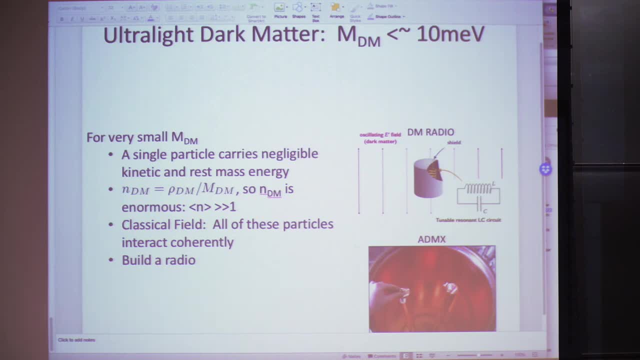 And now you're not going to look for the annihilation of a single particle, You're going to look for the annihilation of, like hundreds of particles. And this is what a radio does, right, Like when I listen to FM radio, I'm not trying to sense. 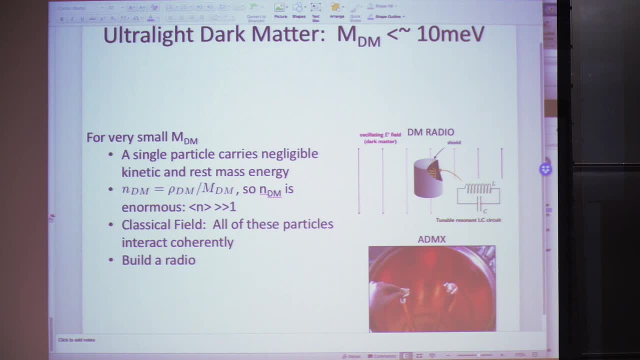 a single megahertz photon. I'm actually sensing a huge number of them and a huge number of them hitting my detector, And that's what we're going to do when we go below something like 10 milliV is we're going to try to interact. 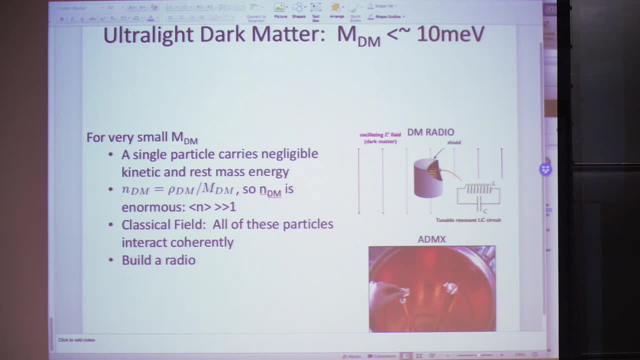 with a huge number of them. So that's DM radio. We're going to build a radio, So every experiment below 10 milliV is just a radio experiment. to first order. Okay, thanks, Any more questions? Time for a couple questions. 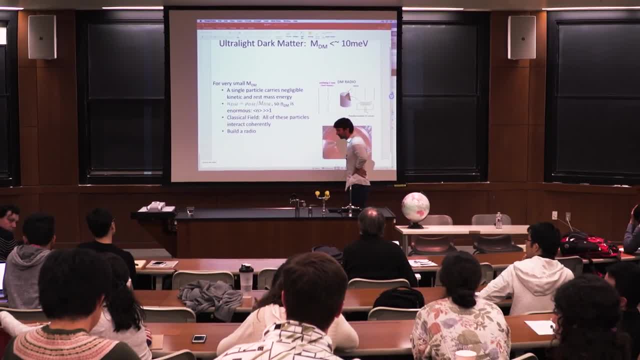 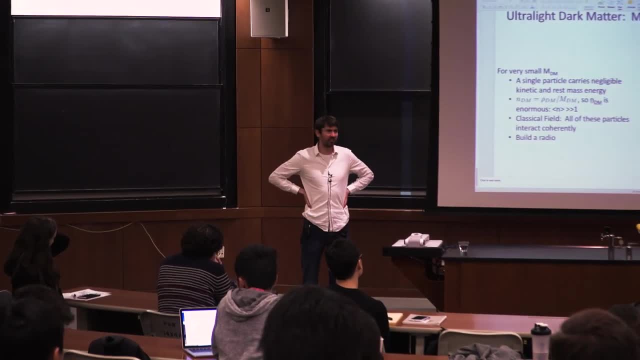 Above, like 10 to the 19th GV, where your scale cuts off. is there any realistic detector design or is that just to do? Oh no, So all of those- and actually there's going to be a talk on this this afternoon- right? 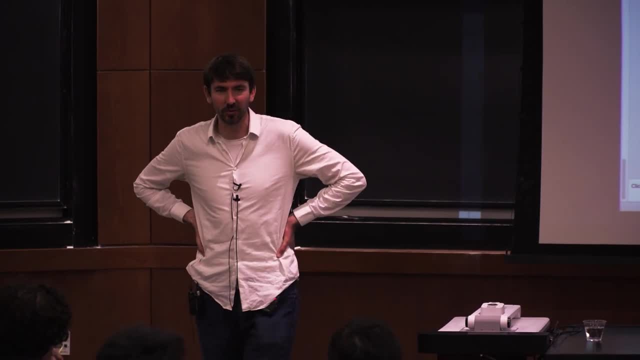 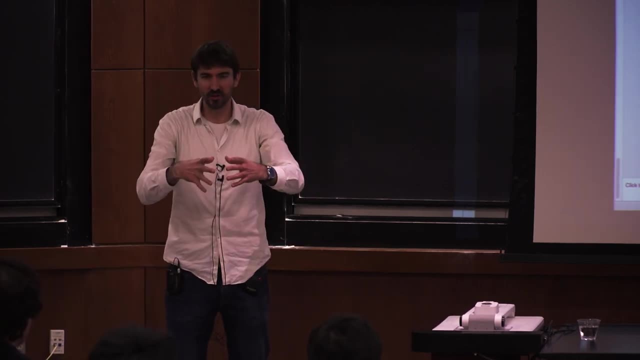 about using weak lensing and stuff. So once you get to a certain size, you're not going to look for particles with yeah. So what are we going to do? So we have 10 TEV where it's going to keep on going. 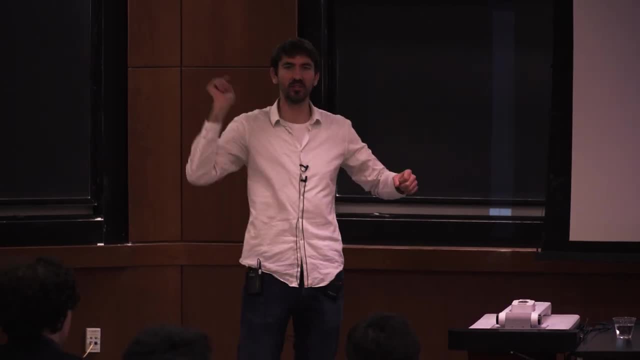 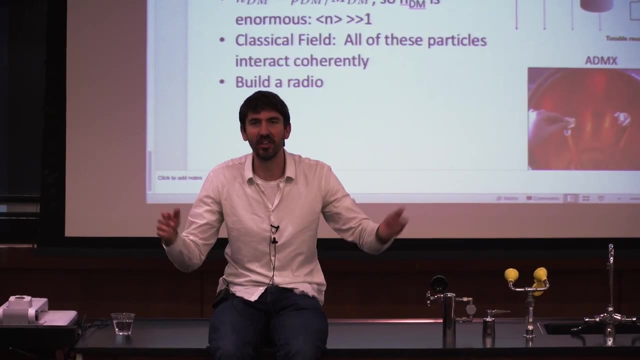 building bigger and bigger detectors And, like you know, IceCube is enormous. so you say, oh, I can go up to like 100,000 TEV, But if you get up to that size, the odds of having a single particle 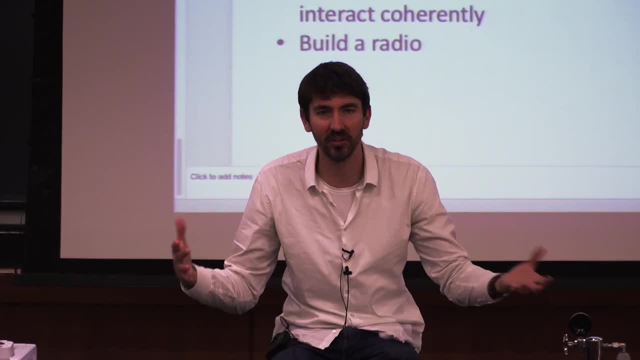 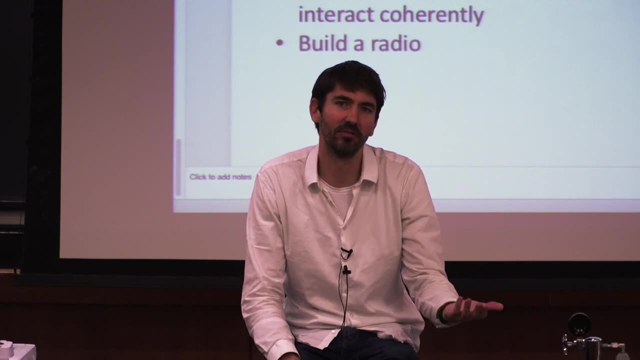 just go through, your detector becomes zero, right, So you're never going to build a terrestrial experiment to do that. But then there's some range where now we can start looking out in outer space and look for lensing off of these events, And that is basically. 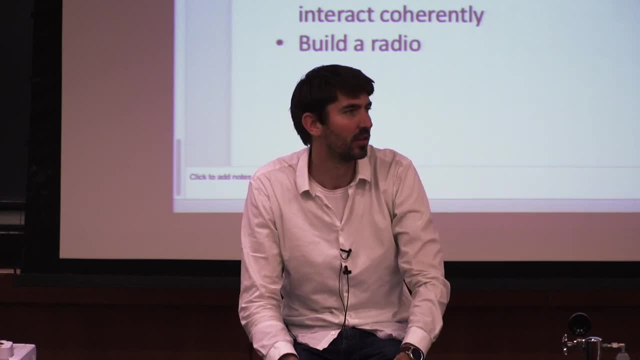 what we're going to do for high masses. Okay, All right, thank you, Matt. We'll Thank you.